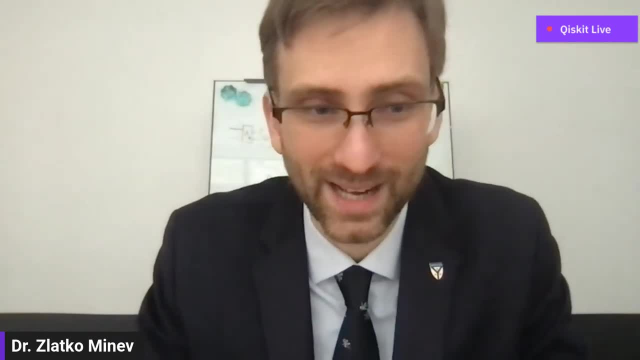 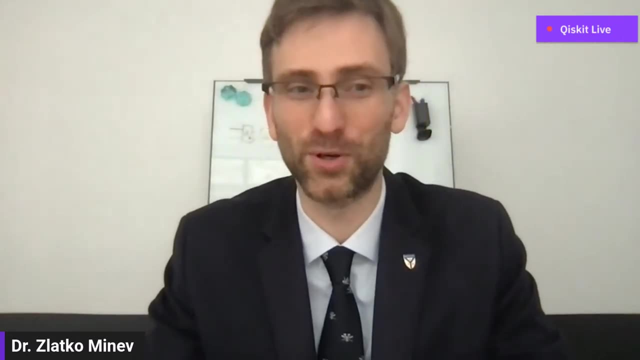 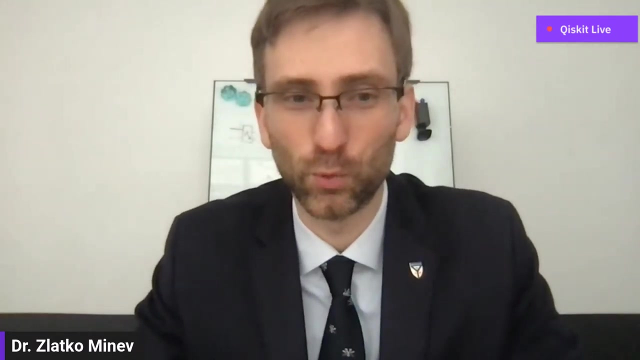 Durham, Portland, Yokohama, Canada, Michigan, Wisconsin, Madison. So thank you everybody for making all these different time zones and joining us. So with that, I think it's time to roll out the latest 111th episode of IBM Qiskit Live Quantum Seminar Series. 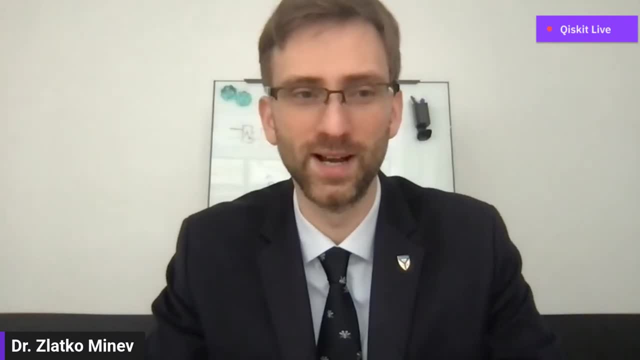 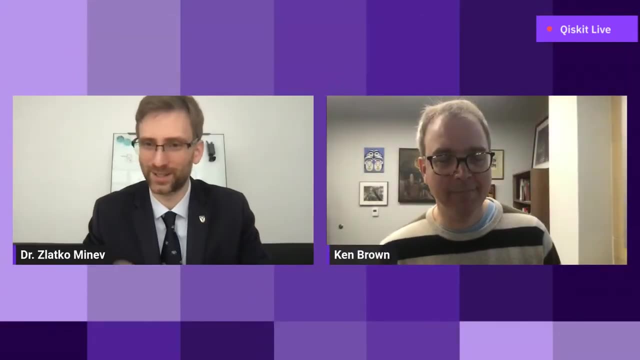 dedicated to you, the research and academic quantum communities. I'm your host, Zlatko Minif from IBM Quantum Research, And today I have the special pleasure of hosting Ken Brown from Duke. Hello Ken, Hello Zlatko, It's good to see you. Before we dive into your talk, Ken, allow me to you need. 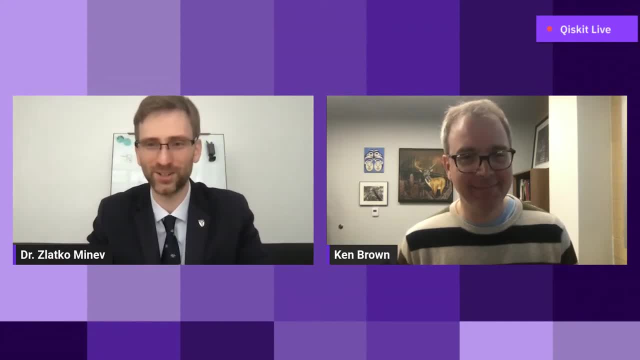 no introduction, but allow me to introduce you nonetheless, as that is my job here. Ken Brown is the Michael Fitzpatrick Professor at Duke University. Ken is a very distinguished scientist and researcher and currently is the Director of the NSF Software-Tailored Architectures. 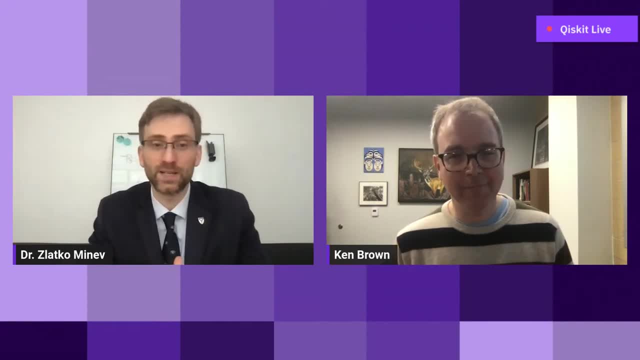 for Quantum Co-Design STIQ project. Ken represents the DPI, or Division of Quantum Information, on the APS American Physics Society Council and is also on the editorial board of PRX, Quantum and IEEE BITS and serves as a scientific advisor for IonQ Ken and Ken's work has been recognized with many awards. 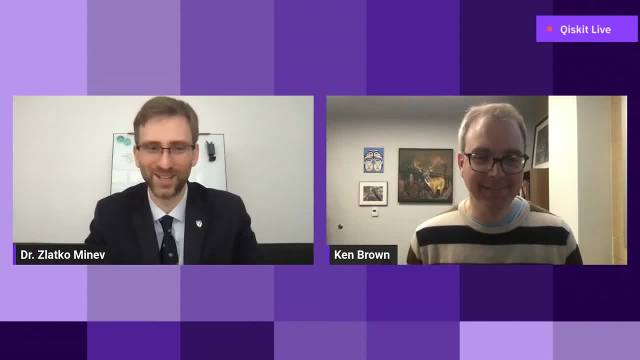 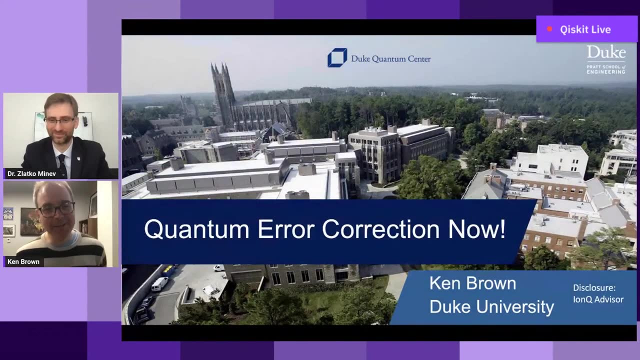 He asked me not to name all of them because it's a very long list. So with that I bring to you Ken Brown. Great Thanks, Zlatko, And thanks everyone for tuning in. I'm really happy to be here to talk to you about quantum error correction. I am in Durham. We actually are in the Chesterfield. 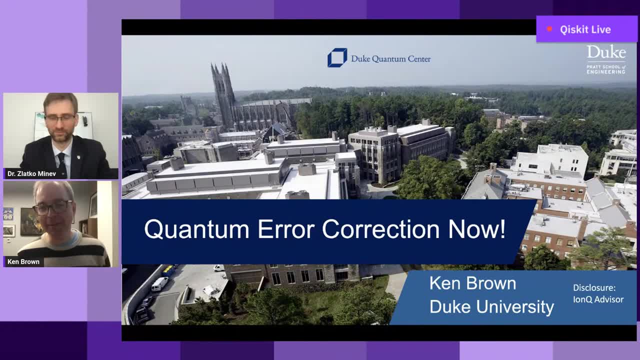 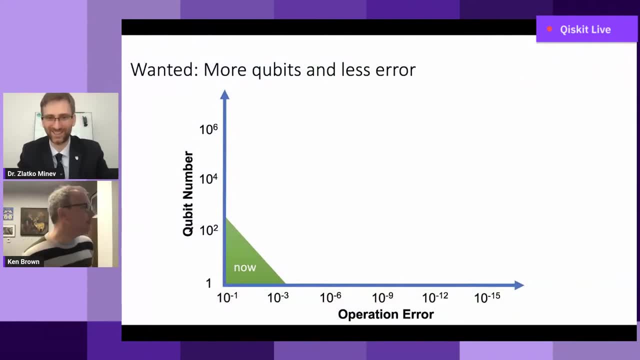 building downtown, far away from the beautiful Duke campus, as you can see on this photo, And I understand the building is quite special. Yeah, Actually, the Chesterfield building is the first automated cigarette factory in the United States, I believe, And now it's been transformed into a space for Duke Quantum. 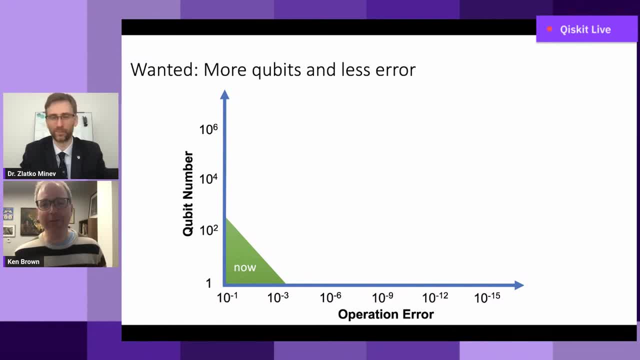 Research, the Duke Proteomics Center and then and also a lot of other things. So I'm proud to be in the Chesterfield building as well. So I'm very much excited to be here. I've been really excited to be in the Chesterfield building. We have a lot of startup spaces. 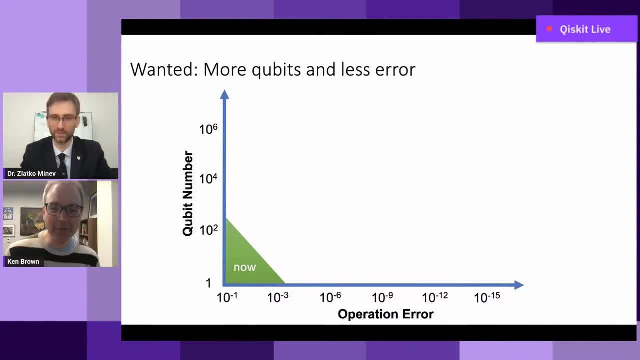 for biotech companies, and also Durham Technical Community College is here as well. Excellent, I'm excited to be here too. Yeah, And then I'll also say yeah, I'll take questions anytime. I don't even have to. I have no desire to get throughout my slides Just happy to talk about quantum. 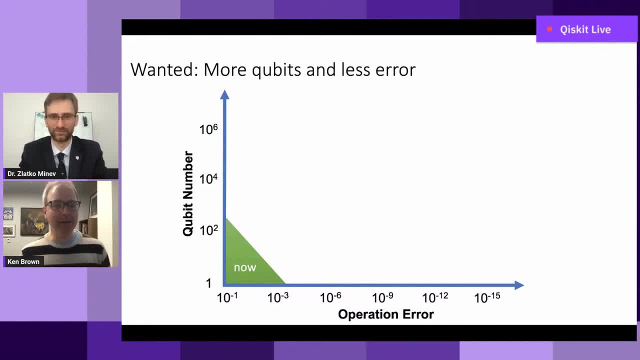 error correction and science in general. So, as we all know, in quantum computing we really want more qubits with less error, And the current time is kind of this green triangle on the side and if we think about things that maybe you want. 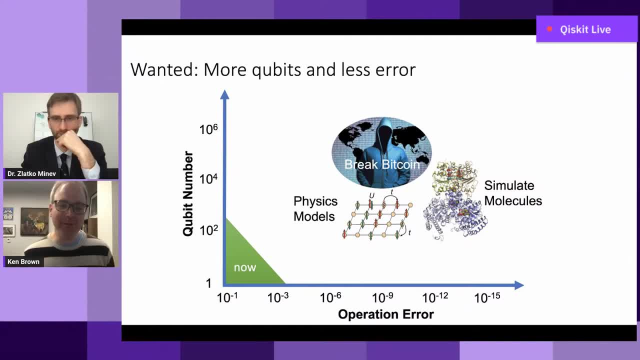 to do like i would like to break bitcoin. maybe you want to simulate molecules. i also like to simulate molecules. maybe you want to run physics models and we have to ask, like, how much are these things going to cost to be competitive, not with your laptop, but with, like real supercomputers? 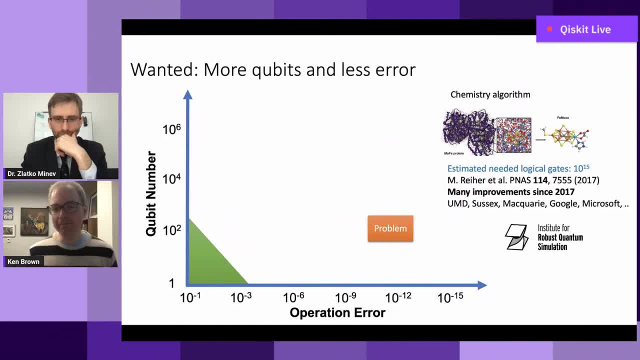 and so, just as an example um is it back from my background in chemistry i've always been interested in- can we use the quantum computers to solve hard chemistry problems? so in this 2017 paper um, researchers at microsoft and eth suggested that you would need about 10 to the 15 gates. 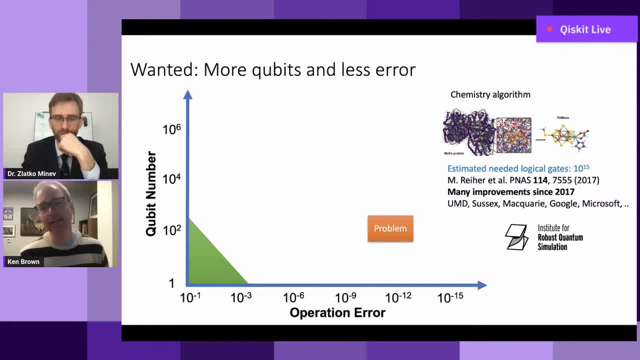 to look at this catalytic center in nitrogenase and there's been many improvements across the world of making this cost less. so let's just imagine that it's going to cost about 10 to the 12 gates and then we need kind of an operational error- 10 to the minus 12- and i just want to say 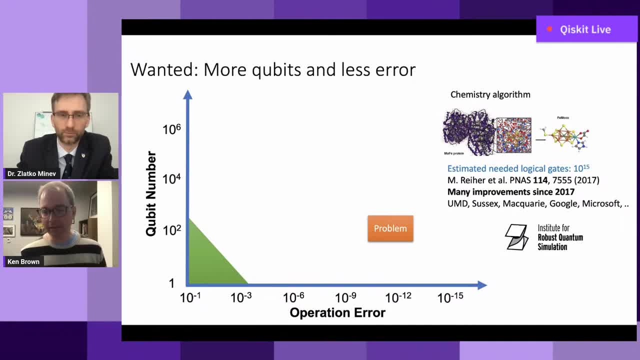 that i'm part of the institute for robust quantum simulation, which is based out of the university of maryland, and and we look at all levels of quantum simulation, from what we can do right now to these very kind of like what can we do in the future questions. so one thing you could imagine is: 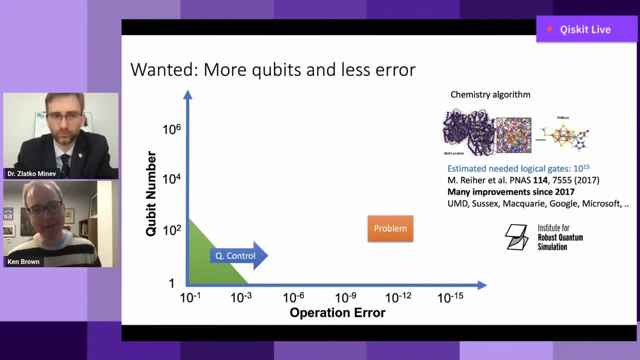 well, why don't we just use quantum control to make our qubits better? um, i don't know where the limit of that will be, but it's hard for me to imagine that will get us out to 10, to the minus 12.. we should. 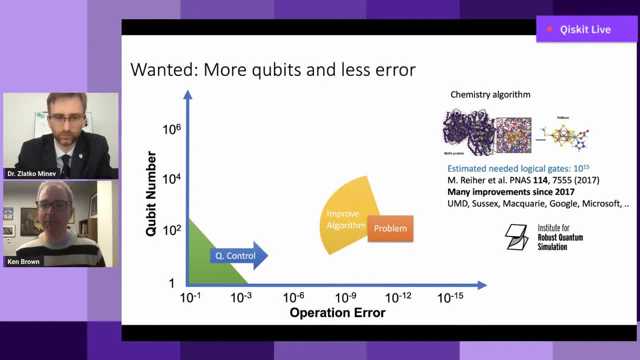 of course, try to make our problems easier, and that, again, is what many people have done and i. i find it kind of interesting, because sometimes we make the problems too easy and then suddenly they become accessible to a classical computer again, which is great for the world but, uh, you know, defeats our goal of finding these quantum. 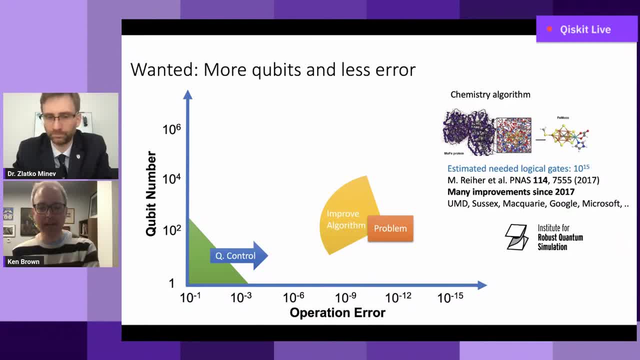 problems that we can, uh, really show an advantage on. so the idea of quantum error correction is we just scale up the hardware to many, many qubits and then we use quantum error correction to take many kind of noisy quantum bits into a few very precise and accurate quantum. 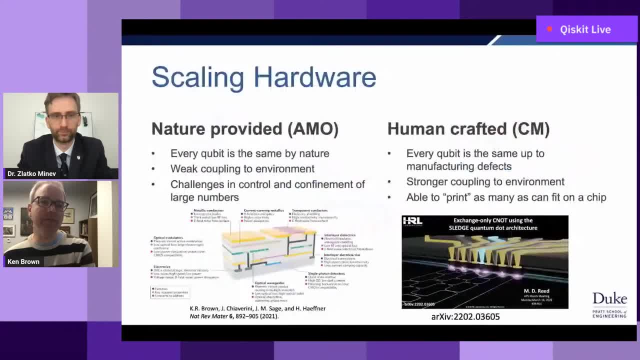 bits. so how are we going to do this? so the first question is like: well, how do you scale up the hardware? and i do think in the community there's kind of a split between kind of nature provided qubits, which we think of like atomic, molecular and optical physics, and then human crafted. 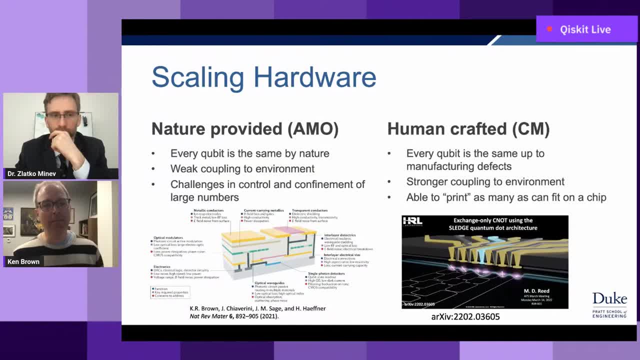 which come from more of a condensed matter point of view. um, a nice scaling question is like: what is the scaling feature of atomic kind of qubits? is that every qubit is the same by nature? um, they're weakly coupled to the environment, but there remain challenges in thinking about how to. 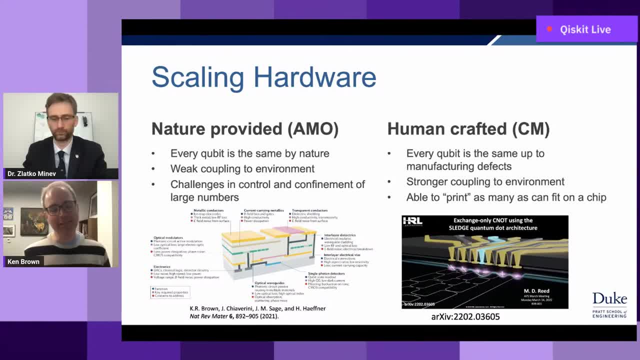 control and build up large numbers. so, for example, if you're interested in some of the materials challenges of building ion shop quantum computers, you can look at this review article that i wrote with researchers at lincoln labs and uc berkeley. on the other side, when we think about human, 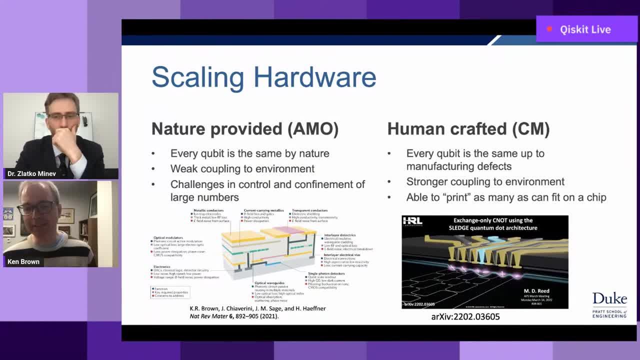 crafted qubits. what's nice is every cube is the same, up to manufacturing defects. uh, typically there's stronger coupling to the environment and normally people see these as more scalable because we're able to say: print as many as you can fit on that chip. um, but then 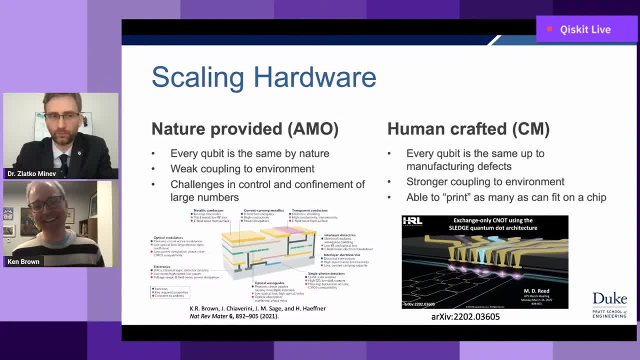 you have to ask like: why are we printing so few per se? and i really like this example of quantum dart architecture where you print basically um three, double, well, quantum dots to form just a single qubit. and that's, i think, is the most fascinating thing, which is hilbert. space is really just a vast expanse. 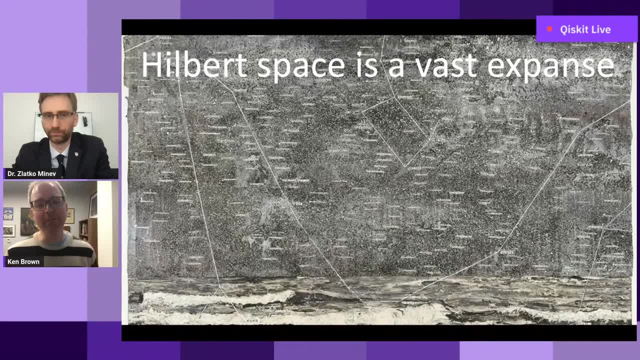 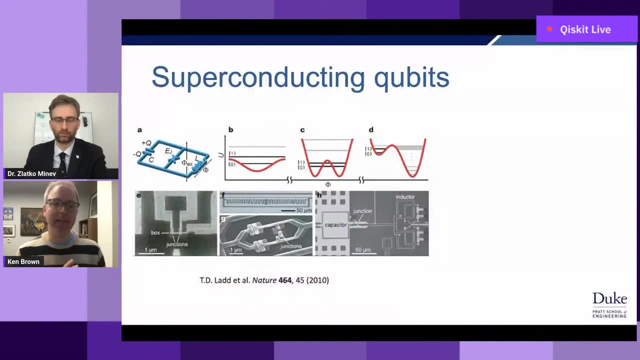 and so whenever you talk to people about like, oh, i picked my qubit or i picked this qubit, people have already made a huge down selection of all possible things you could do, and then you know they tweak with these different things: um, yeah, so this, um, as an example. 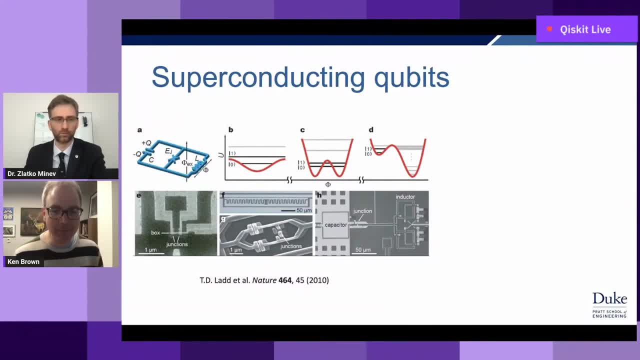 uh, one thing i really like to look at is this, this beautiful review paper from 2010 about different ways to build quantum computers, and here we have three different ways to build quantum computers using superconducting qubits out of jose's injunctions and superconducting lines. 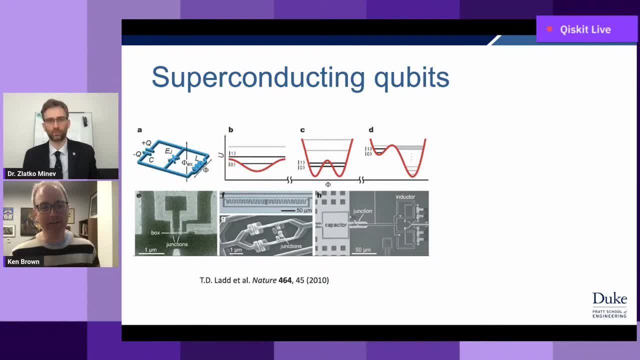 and b, c and d correspond to the kind of level structure you would expect for these energies, and there are many, many levels and we just picked two to be our qubits. what i really like about this, this picture, is that this paper is after the invention of the transmon. 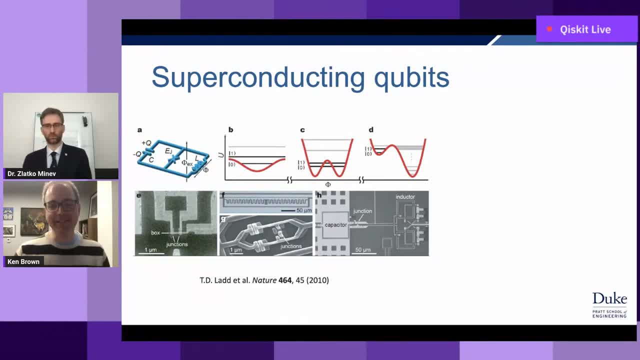 the transmon has not yet been successful enough to make it into the summary figure. if you, you know, jump ahead a decade. uh, you see that actually you know the transmon, and then extensions of the transmon are really well talked about in this um review article from: 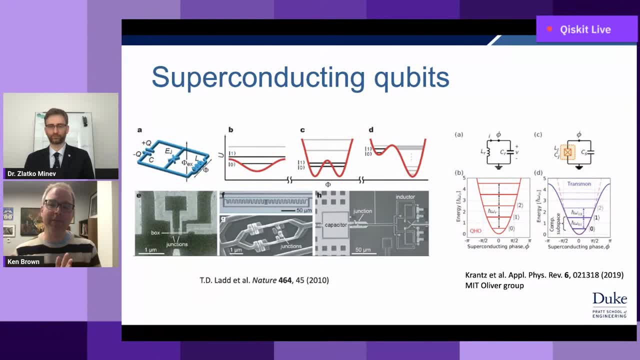 will oliver's group at mit, where we move closer to something which is very harmonic and has like a slight bit of anharmonicity. um, and from a broader perspective, right, there's no limit to how we can put together their doses and junctions of superconducting wires and resonators. 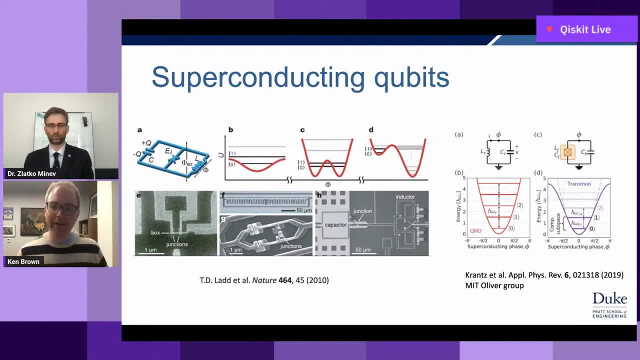 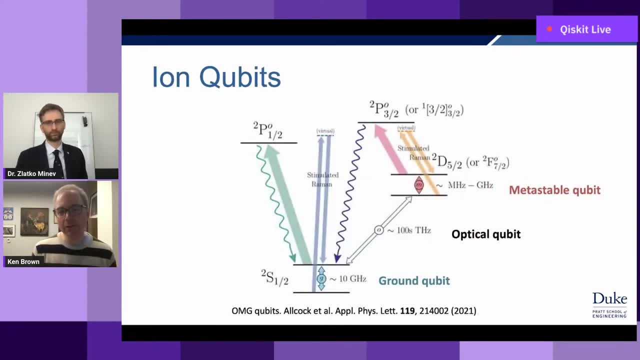 to make qubits and so there's a huge unexplored area of hilbert space. defining like, what is the good right say qubit. same thing is actually true also in atomic physics. so, as an example, looking at ion trap qubits, typically ion trap qubits have primarily been ground qubits, so the 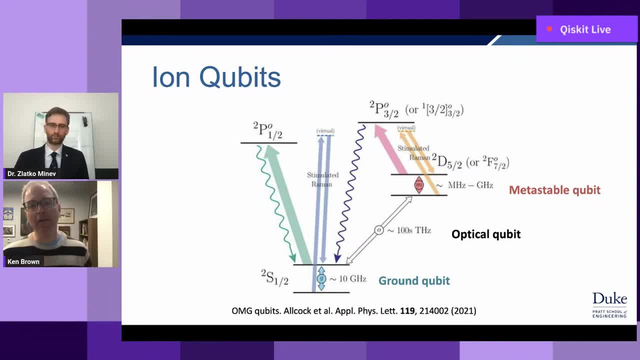 the information is stored in the ground state of the atomic ion, qubits. so a lot of the really great work in calcium ion quantum computing has used an optical qubit where one state is in the ground state of the ion and the other state is in a 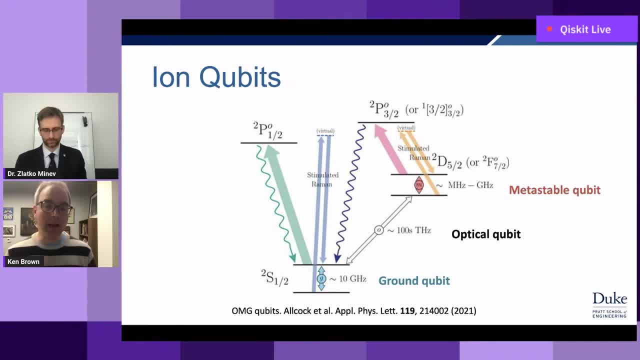 metastable state um. there has been a couple of just very few works looking at a metastable qubit, where you actually just put the qubit up into this long-lived d-state um, and recently, in 2021, there's a nice paper where they- where researchers kind of argue that to get the most out of these ions, 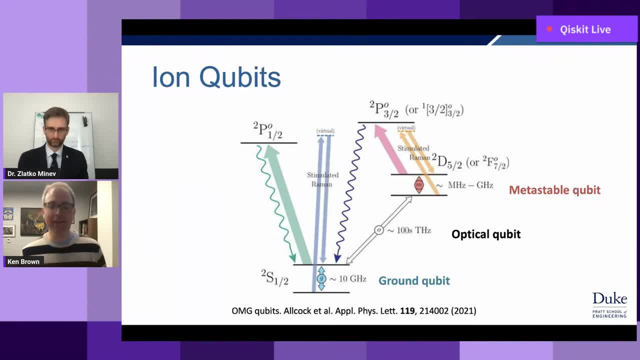 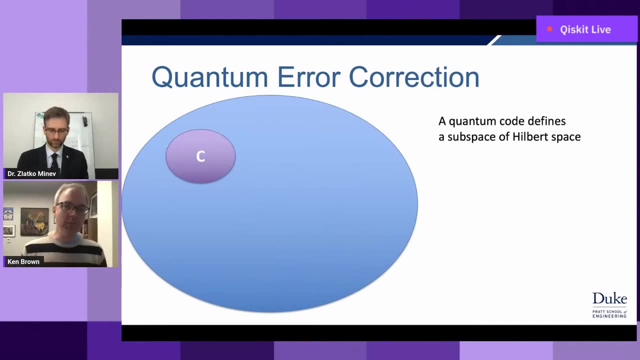 you could be useful to use all three qubits to basically push the quantum information, the two level system, around this atom, which has a vast, which which by itself has a vast hilbert space of places we can store this information. so, once we've decided on our quantum bit, 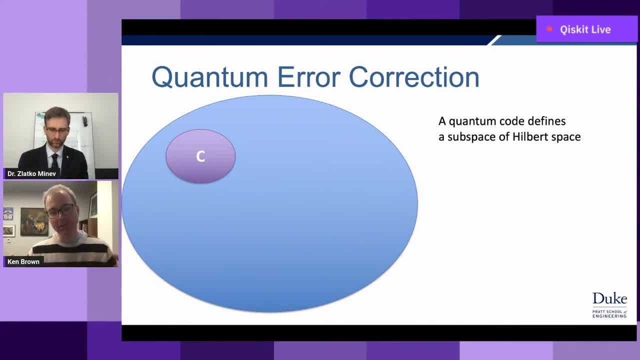 um, the next kind of region of hilbert space we want to look at is taking collections of those bits to define a quantum code. right, so quantum code is is you know? again, you just make a sub selection of a massive hilbert space. but what's nice about? 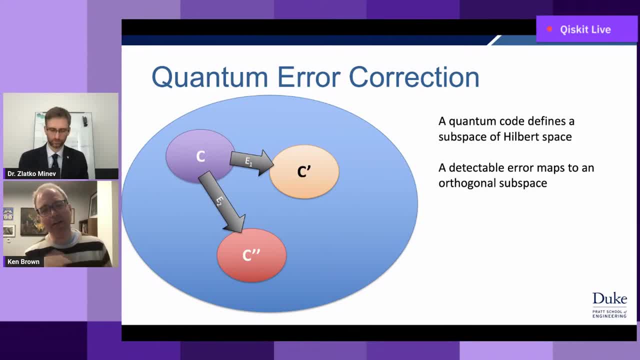 a code is. it guarantees that for the errors that we expect will happen, it leads to detectable orthogonal subspaces, and then that allows us to have a correctable error that can be mapped back right. so this is- this is kind of a an interesting point, because instead of thinking about the qubits, 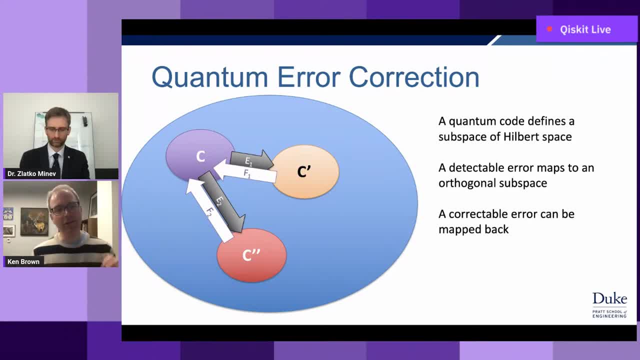 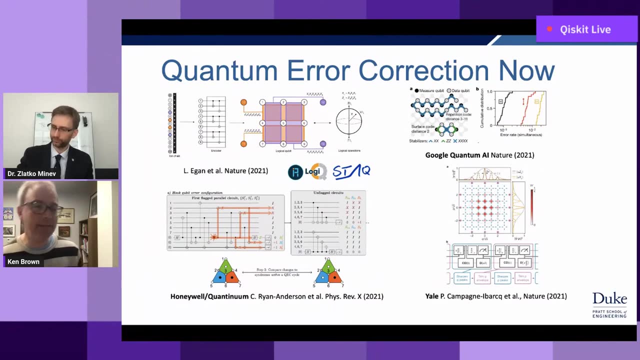 and the best single qubit. it probably becomes useful to think about a qubit which is best in terms of this next layer map, um, where it not doesn't have to have the least error, it actually just has to have the most correctability. so, um, i think what's been great in the last few years is there's been tons of quantum error. 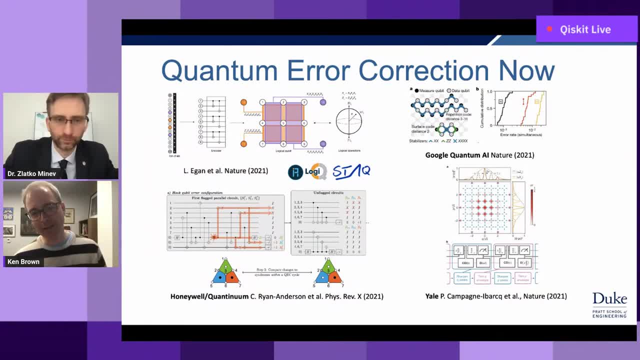 correction experiments. these are just a few. i'll talk about a few more throughout the talk. i'm going to talk a lot about this um, this experiment i was involved in with chris monroe's group, which is, uh, an implementation of the bacon short code which is up top um, using experiments that were you know, 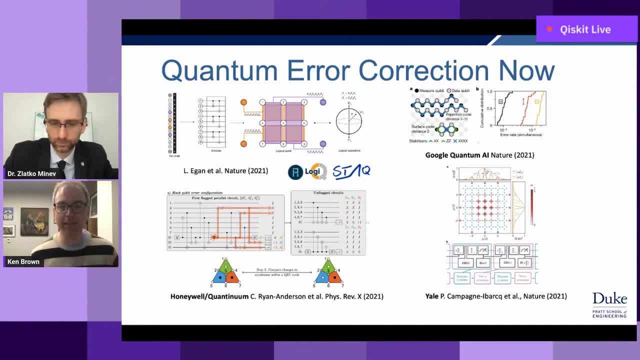 primarily funded by our logic, but also through this um nsf stack project. there have been these long repetition codes from google- it's nice work from honeywell at these color codes- and, of course, um, there's also this interesting work in bosonic codes um, which is which is, yeah, actually great. 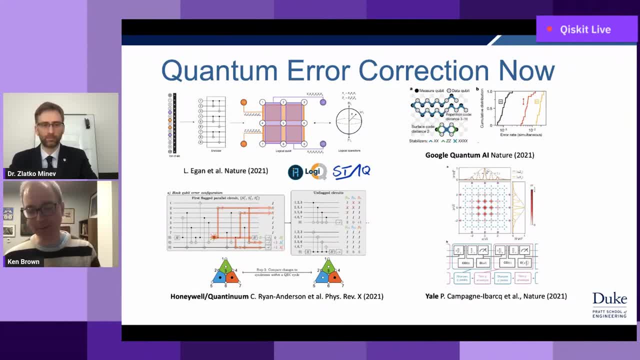 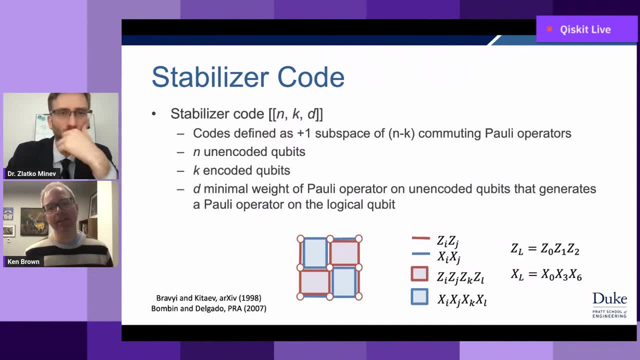 interesting direction right now, um, which i'm going to ignore, except for this one picture. so, um, just to try to get everyone up to speed, we want to talk a little bit about stabilizer codes. so remember that a stabilizer code is defined by three numbers: number of qubits, the number of encoded logical qubits, k and the. 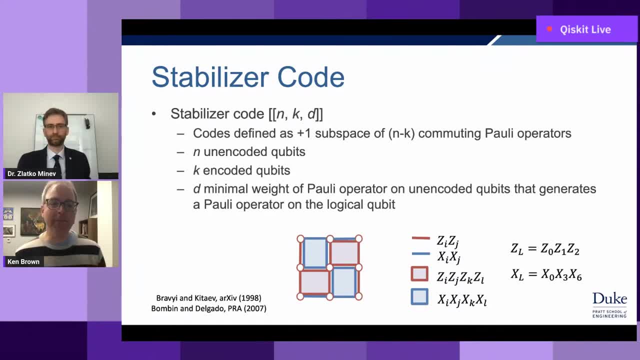 distance d? um. we typically look at these um calderbank steen shore codes, where the z checks and x checks are separate um, and then we look for the plus one subspace of all these poly operators, these poly operators that splits hilbert space into these different correctable subspaces. 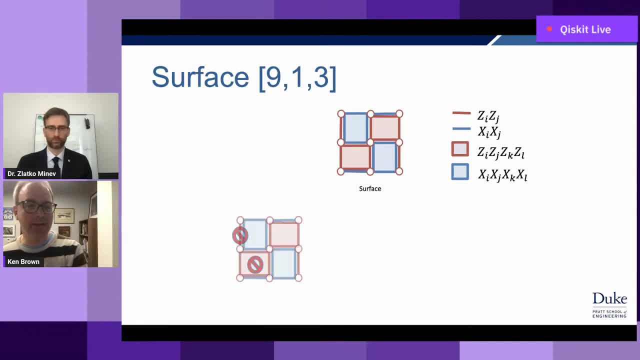 um, so again with the surface code, just as a reminder, what we see is we see syndromes being changed and these, uh, red circles represent, you know, syndromes which have flipped, and then we can decode them to find that. okay, there's an x error here. 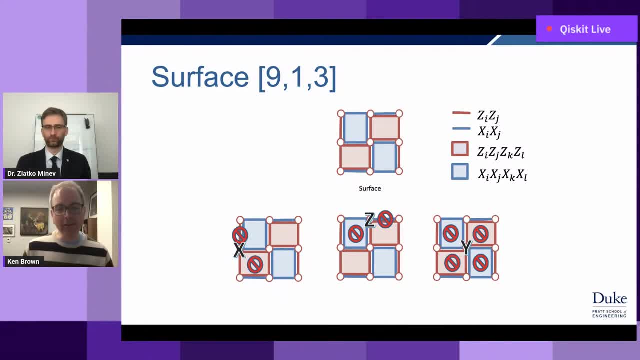 z error here or y error here, and that's the encoding, decoding procedure, and it relies again on the data of what the error is, and we can use that to burger from the original model if we want. and so the parts that we use in order to define the error are the poly operators, um, the stabilizer. 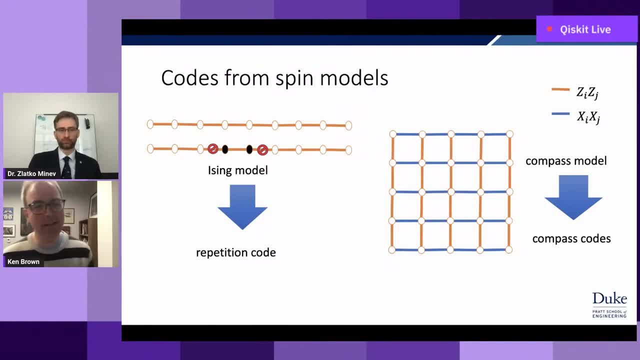 operators, fitting the code into different spaces, and then the fact we expect the errors to be poly operators so that we can then fix it. um, what i find interesting about this, uh, and we spend a lot of thinking about, is if i think about classical error correction. the simplest example is kind of a 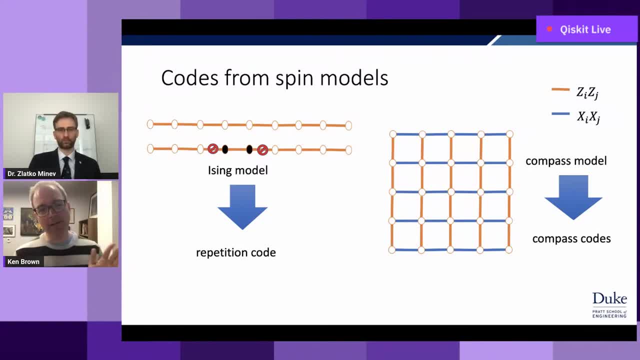 And then the errors in my stabilizer basically correspond to domain walls between spins that are pointing different directions. Now we actually want to fix two errors And so one way that we've thought about it, a lot is through. well, what's the spin model which would have energy violations if it had X or Z errors? 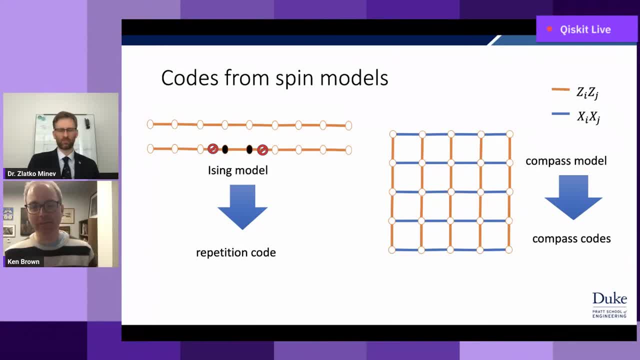 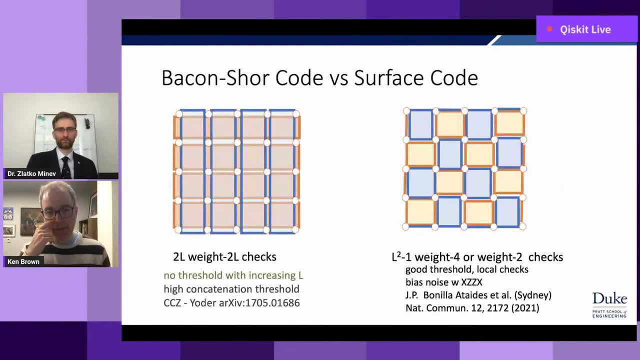 And that could be a compass model. And here's like a 2D square compass model with Z-type easing bonds and X-type easing bonds And what we find is that that model can be mapped in limits to two important codes. The one is the Bacon shortcode. 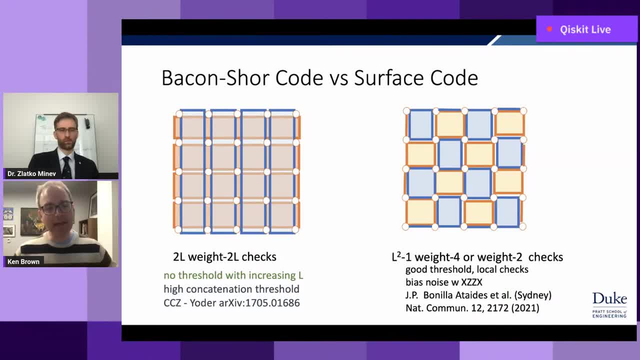 So the Bacon shortcode is interesting because it just has massive checks. They have these 2L, they have 2L weight, 2L checks, Whereas the surface code has- It has- many more checks which are much smaller. So the plus side of the Bacon shortcode is there are actually not that many checks. 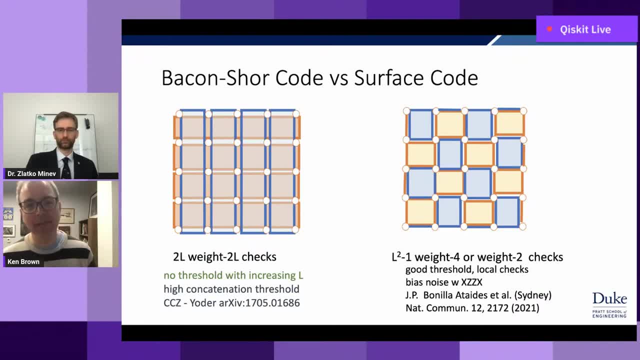 The downside is there's no threshold with increasing L, And on the surface code side, of course there's a threshold, And then of course we can also modify it through things like local Clifford deformation, such as the X-Z-X code, to really map to the kind of errors we actually see. 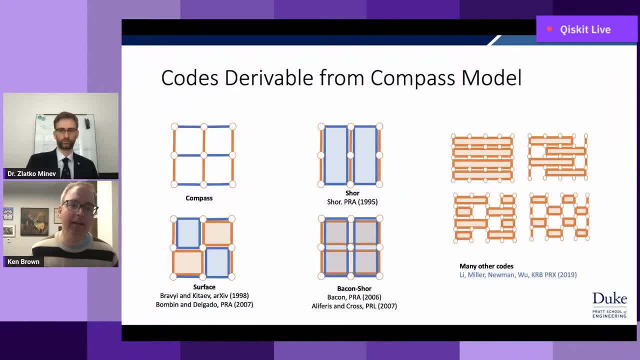 So we've spent some time thinking about what are the other codes that live And what are the other codes that live inside the middle. So from the compass code I take these gauges. These gauges don't form a code space because they don't come with each other. 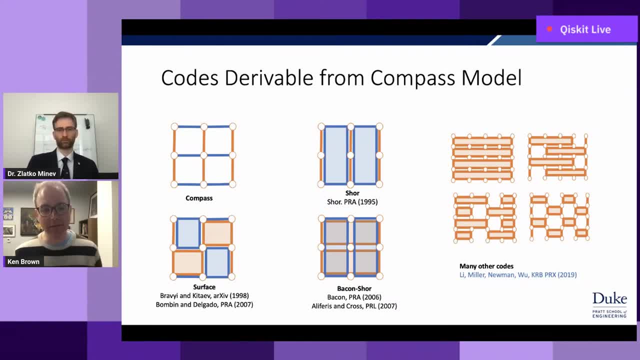 And then I take products of them to generate CSS codes and I can get both shortcode Bacon short surface code. thinking of this, And with me and Lee and Daniel Miller and Mike Newman, we were able to basically look at a very broad range of these codes. 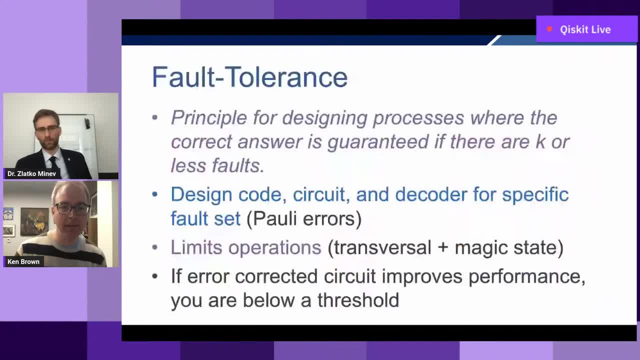 And actually kind of see where the threshold comes from. So we want to move beyond codes to actually implementing the process of doing the error correction, finding the syndromes and getting that error, And so I call that procedure we want to implement, say, a fault tolerant procedure. 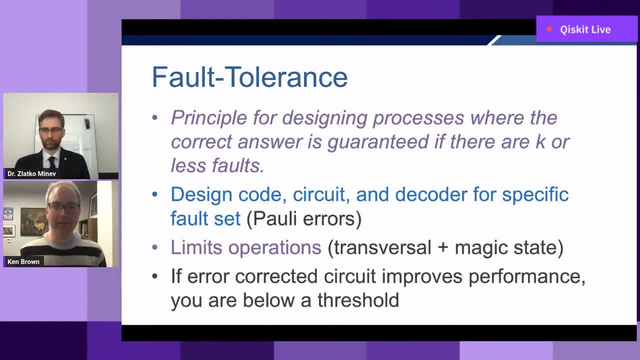 And I don't think- I personally don't think- fault tolerance is a, is a physical, measurable thing. I think it's the design principle, So our principle for designing processes, where the correct answer is guaranteed if there are some number of faults or less. we'll say K faults. 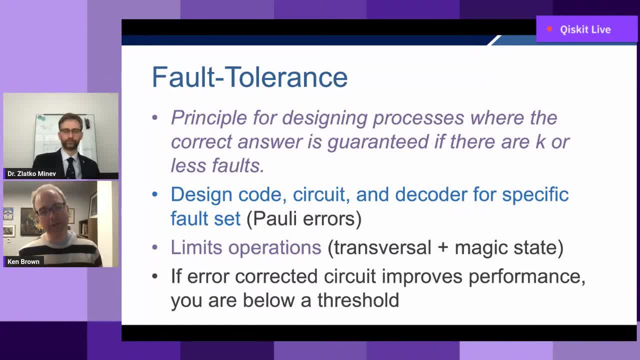 So here we've designed the code, the circuit and decoder for a specific fault set, which are poly errors. This leads to a limit of operations and it leads to like one of the main cost of error corrections in terms of having, like magic stays and ways to get engaged that are not transversal. 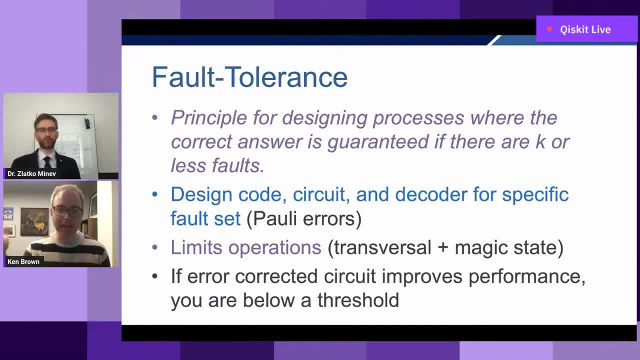 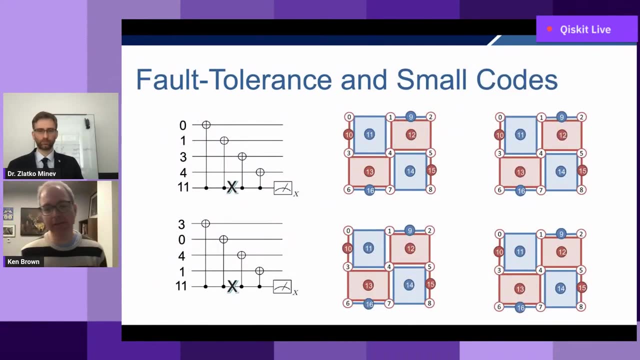 And Okay, That can all happen just through design Right. And then error correction is useful if the performance improves, And that means we have to be below some some error threshold. So what's tricky about fault tolerance is that the errors interact with the circuit in a way where things like timing and dynamics matter. 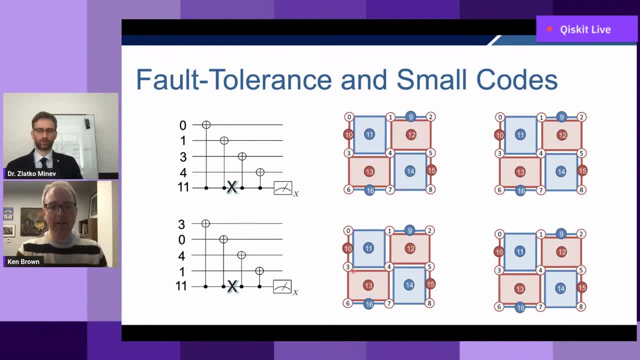 So here what I'm doing is I'm I'm measuring this, I'm measuring this syndrome here, this X syndrome here, and I have these four qubits- 0,, 1,, 3 and 4, which are the data qubits that touch the syndrome- qubit 11, and then I can pick some order of CNOTs to implement that circuit. 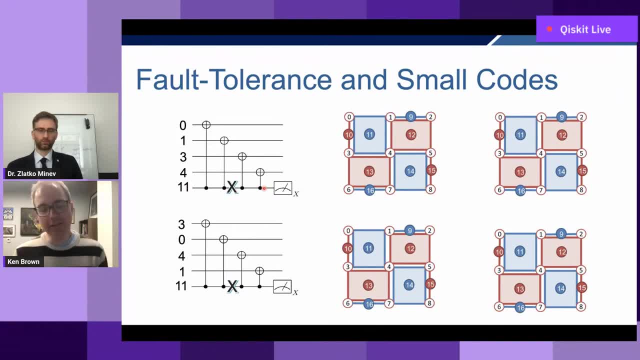 And these CNOTs all commute with each other. So if I just look at the circuit, it doesn't matter, for example, if you're, if you have a compiler which tries to compress things together, they can easily push them all over the place. 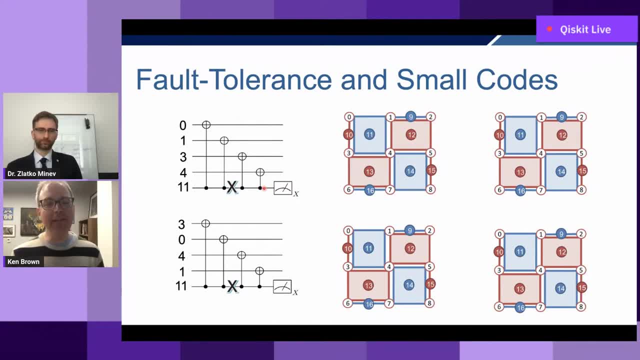 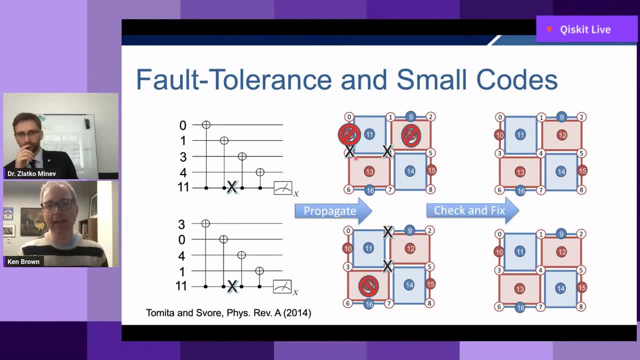 Now in the top situation. when I then check my syndromes in the next round in the bottom situation I get a very different pattern And if I do a fix based on a single on the minimum weight error On that next pattern, here the minimum weight error is an X on the bottom, here it could be either three, four or zero, one or equally good checks. 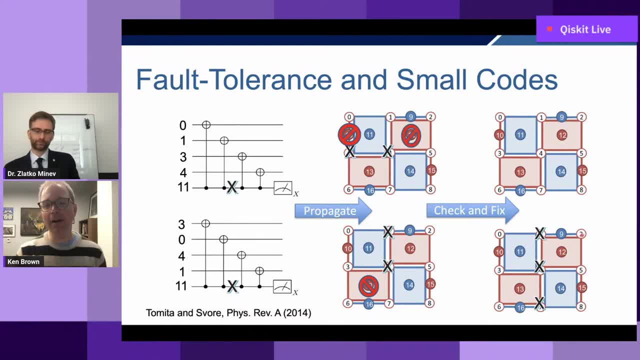 And the result is: at the top, error goes away, and at the bottom you've generated a logical error with this single X file, And so the value of this ordering for these small rotating service codes was first shown by Tamita and Suar in 2014.. 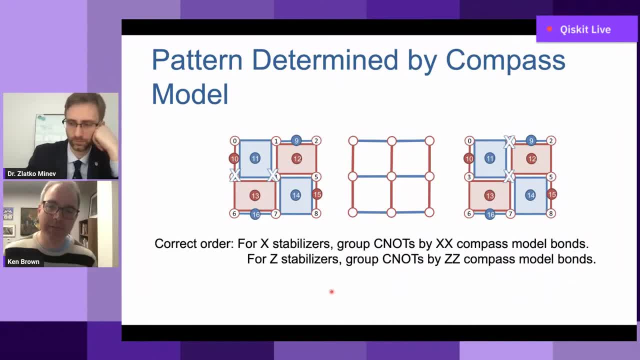 So what was useful for us in terms of rethinking this, In terms of the compass code, is that we basically think that these bonds of the underlying gauge give us information about how to build the circuit. So as long as we build these circuits so that we collect the gauge operators in order in the circuit, then it will be default time. 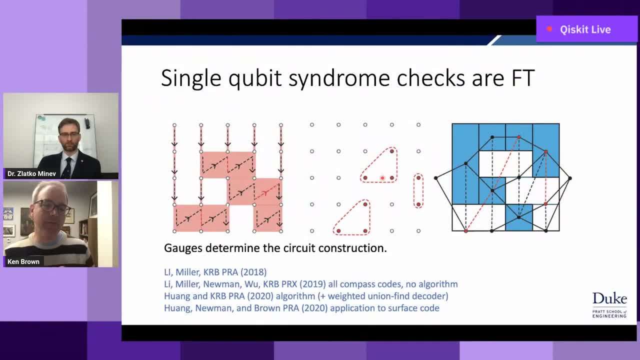 And what's remarkable is that actually works for all of these codes that exist, Exists between Bacon Shore and the surface code, and it actually doesn't depend on the size of the checks And so these weights. So these are the checks here. This is the corresponding decoder graph. 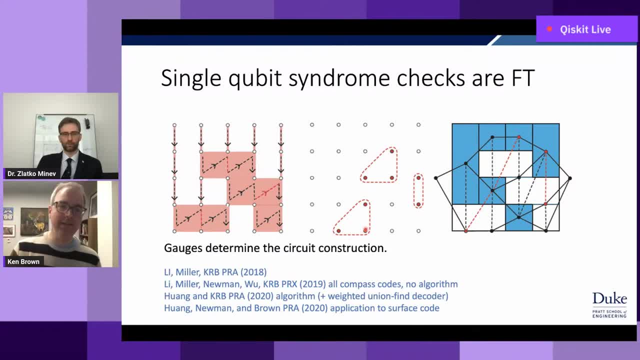 This is kind of a graphical description of how the errors can spread. We're basically guaranteed that by following this gauge is our way to make the circuits, We maintain this sort of capable tolerance. So we were able to first show that for the Bacon Shore code, show that it works. for all of these codes that come from compass codes, show that we could actually build. 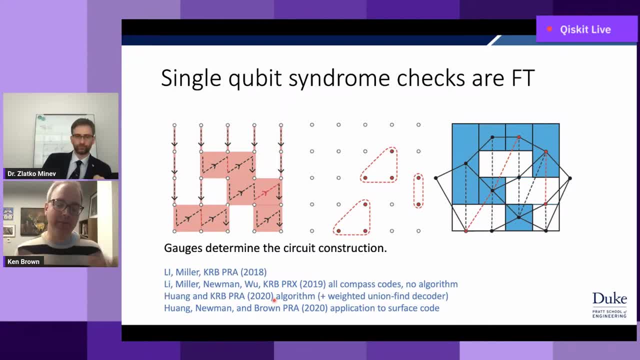 Yeah, we then tested it numerically with a fault tolerant decoder, And my student Shilin Wang developed this weighted union-fine decoder which then we find is like a nice, fast way to do decoding which exists between sort of union-fine and minimum weight- perfect match. Okay, So we're able to show that for the Bacon Shore code. So we were able to first show that for the Bacon Shore code. show that it works for all of these codes that come from compass codes. show that we could actually build. 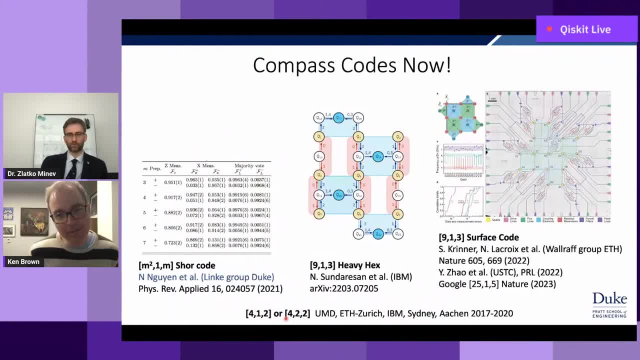 Okay. So what's great is a lot of the error correction we've been seeing lately are related to compass codes. with Norbert's group- Norbert Linka's group, who's now here at Duke- We did this kind of simulation of Shore code, making larger Shore codes but just emulating. 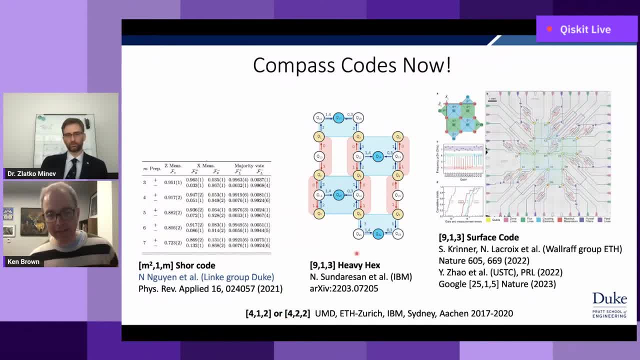 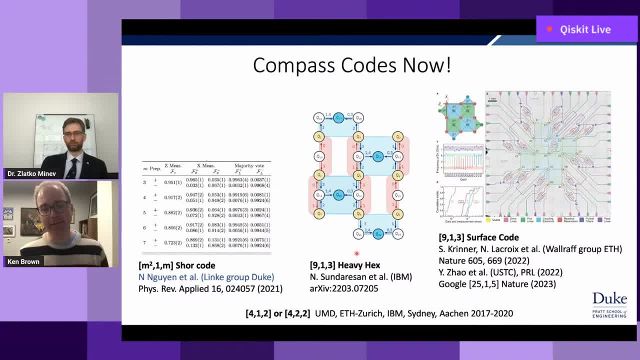 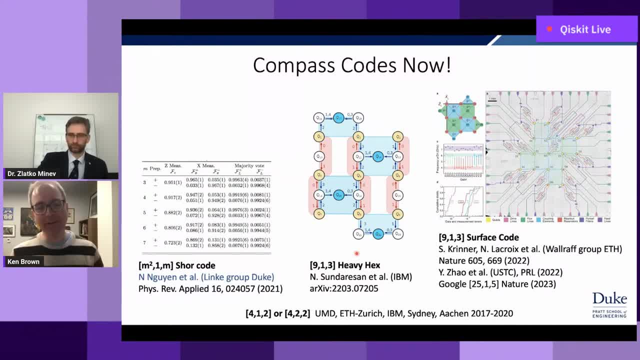 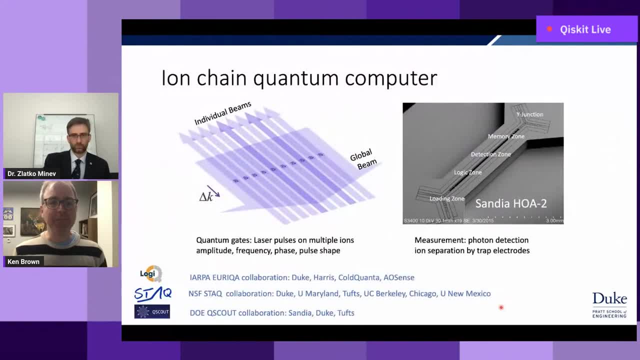 model And, of course, before these error correcting codes, people had done work on error detection code again all over the world, which is quite nice. So now what I want to talk about is our nine qubit Bacon Shore code using trapped ions. 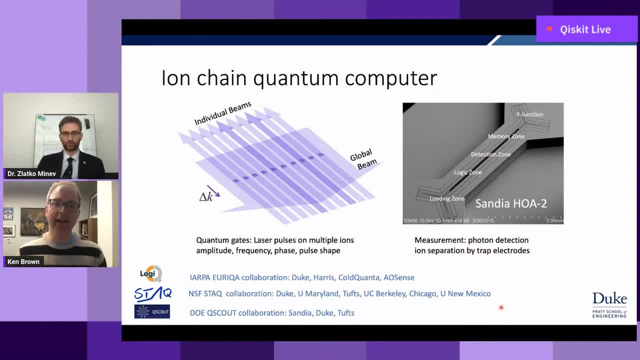 We have an ion chain quantum computer. Basically, the ions are addressed Individually by laser beams with a global beam on the other side. to create the Raman transition, We use the Sandia National Labs surface electrode traps to hold the ions above. 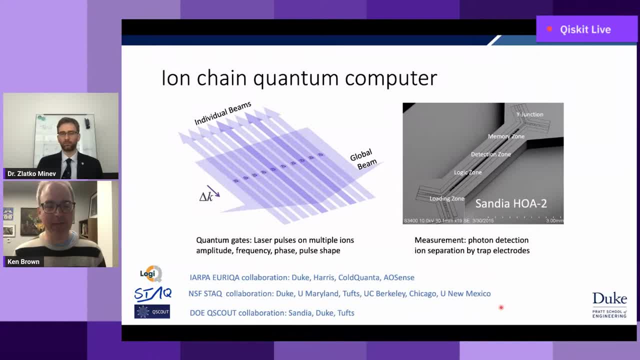 This kind of trap is common. It's more common nowadays, I guess. So here at Duke we have this, the IRF-Eureka traps, and then also an NSF stack trap which has a similar frame, The DOE QSCOUT program in Sandia. 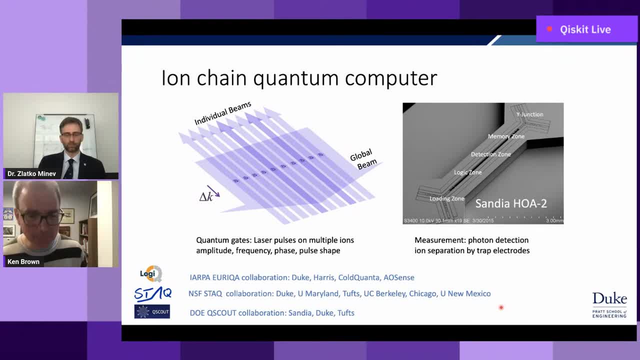 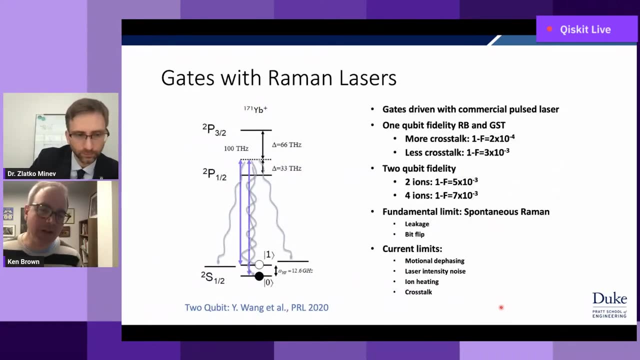 We have a lot of data. Sandia, of which I also collaborate with them, also has a similar trap which is an open source. You can apply to run projects on the QSCOUT project. So in the ion traps, all of our gates are done with these Raman lasers. 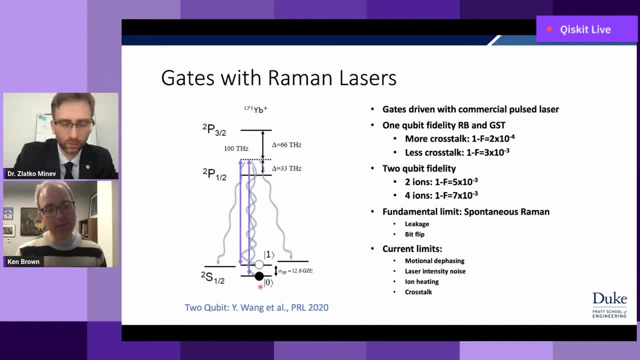 We use ytterbium ions, We use the ground state qubit of this hyperfine state which is first order and sensitive to magnetic field. Okay, And then we use these two lasers to drive both the single qubit gate transitions and by detuning it so it pushes the motion, to do a two qubit gate transition. 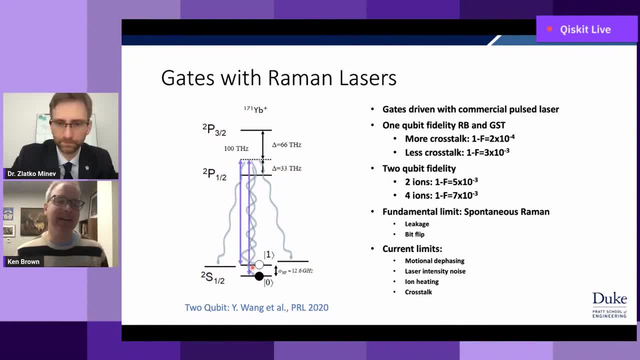 So I'm not going to go into the physics of the two qubit gates today, But the key thing is for us there's kind of effectively no memory error. Our real problem is always gate error. Now, in our best gates at Duke from the US, there's no memory error. 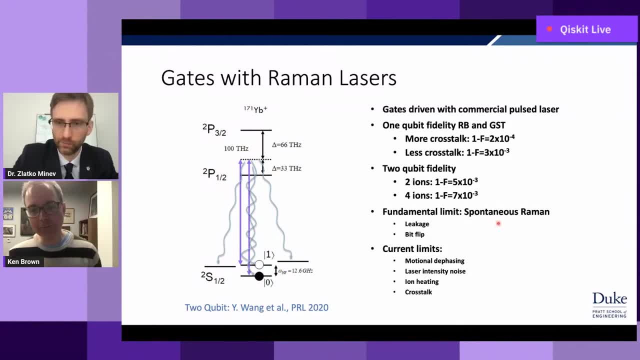 There's no memory error So we're able to get 99.5, 99.3 kind of fidelity in small ion chains. The work I'm going to talk about with the short code- there's the two qubit gate error- is closer to 1%. 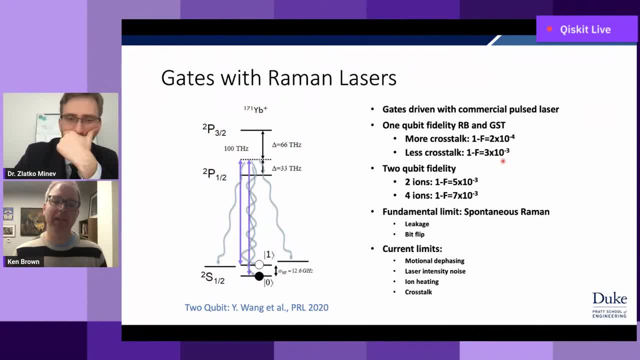 Single qubit gate, errors can be quite small. Fundamental limits involve unwanted spontaneous scattering to these other states, which is leakage and also leads to bit flips. Okay, are due to technical things like motion dephasing, laser intensity, noise, ion heating across them. 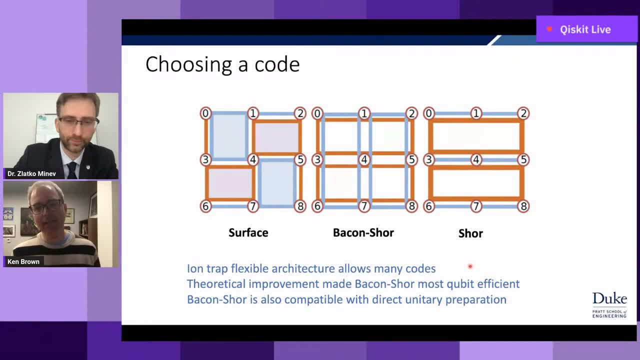 So now the funny thing with this chain of ions is we can do a two cubic gate between any two ions in the chain, And so you could really- yeah, you can- pick any code you want. So once we agree, okay, we're gonna have a nine cubic code. 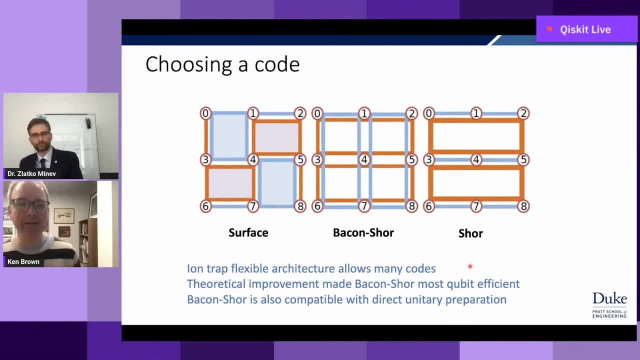 and then I'm gonna have a bunch of extra syndrome checks which we'll count later. So let's just take three nine-qubit compass codes could be rotated, surface code could be Bacon, short code could be short code. and which one should we pick? 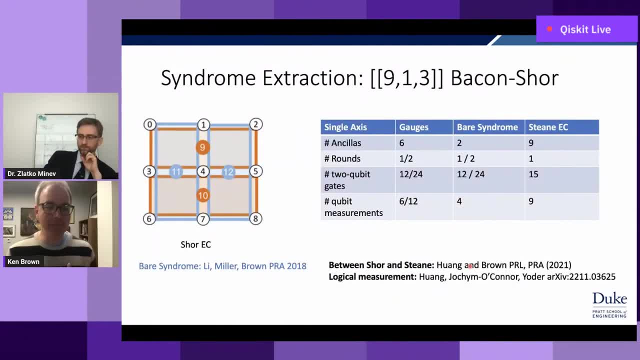 So one of our key results in terms of understanding that we can use a single qubit to measure these, the whole stabilizer, is a real reduction in the number of syndrome-run silly qubits versus measuring the gauges. So yeah, so the original. 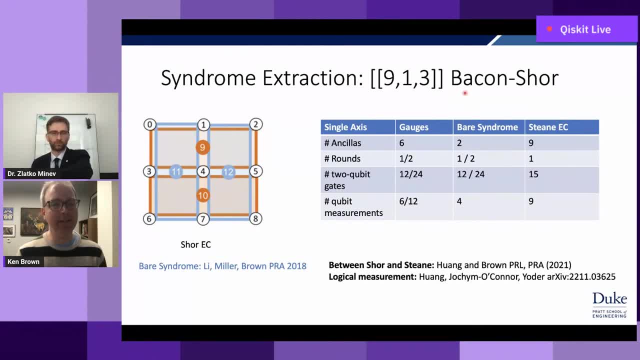 one of the original plans of the Bacon-Shore is because you measure the gauges directly. you would just have a single syndrome qubit connected to these two data qubits and then have kind of again a planar layout. but because we don't worry about the planar layout, 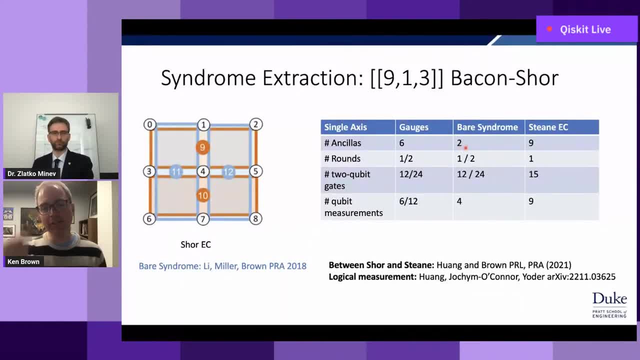 we can go directly to measuring the syndrome, which greatly reduces these number of check qubits we need. Yeah, and so in that work- the work I'll talk about- we do exactly that. so we end up using 13 qubits. 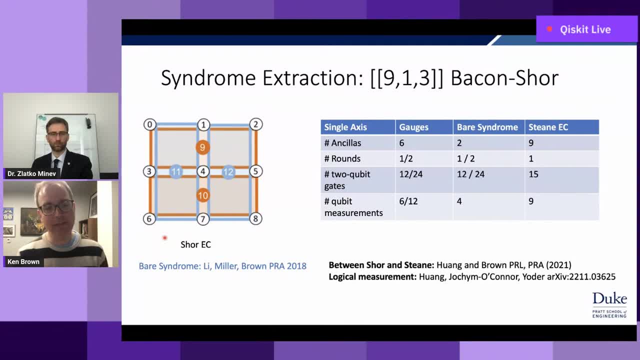 Nine to beat the data and four to check the syndrome. We're also very interested in moving towards Steen error correction. So Steen error correction basically uses one logical qubit to check the errors of another, and the beauty of Steen error correction is that it has 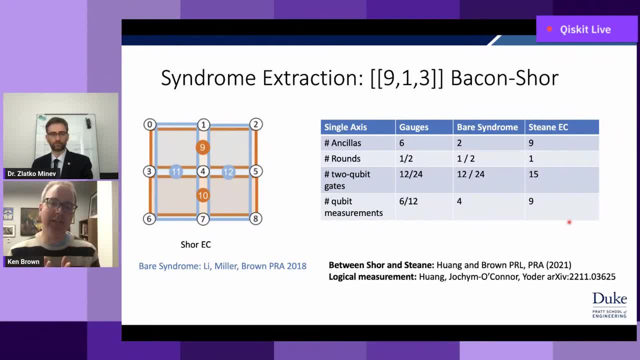 kind of a minimal number of interactions between the syndrome qubits and the data qubits. So if, like us, your problem is gate error and not memory, it makes sense to re-check the errors, reduce the number of two qubits, And so what we see is because I 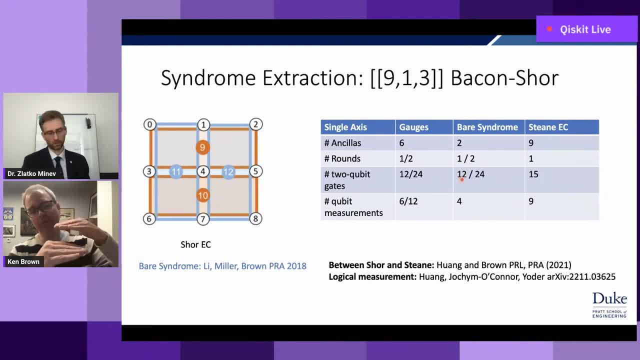 for these kinds of error correcting codes. I have to have it be fault tolerant. I have to do it multiple points in time In our scheme. you could end up having to do like 24 C knots per one type of error- X or Z. 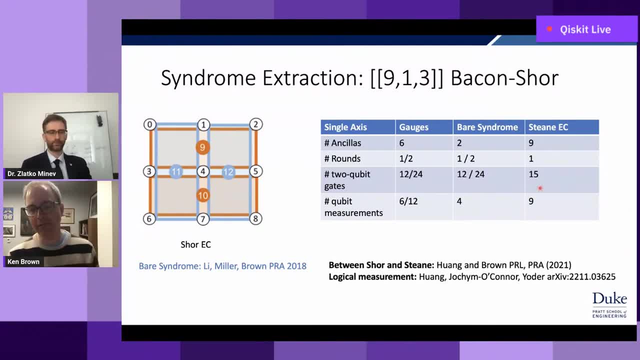 But in the steam code you just need the preparation of the other steam qubit and then this thing. And then I just wanna point out my student, Shilin, had some really nice work looking at all of the different ways to do fault: tolerant extraction between Shor and Steen. 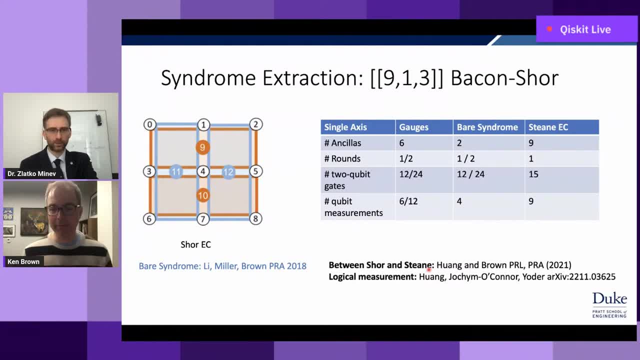 And then he was able to use techniques that he developed in that paper to work with these researchers at IBM- Thomas Yokel-McConner and Ted Yoder- to show how you can use those similar techniques to do logical measurements on a wide range of codes. 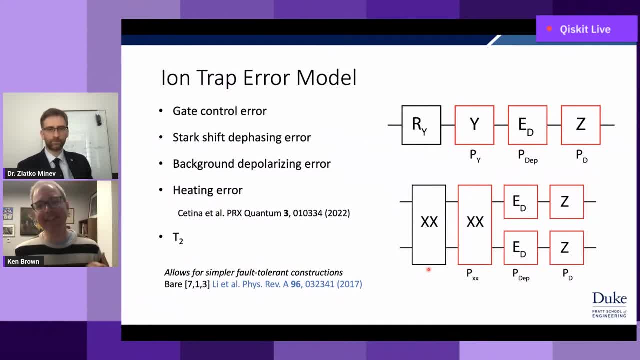 All right. so the next thing is: I've been emphasizing that for us the problem is the gates And, more specifically, for us the error is primarily related to over-rotation, which could be systematic. So there's like a real angle error. 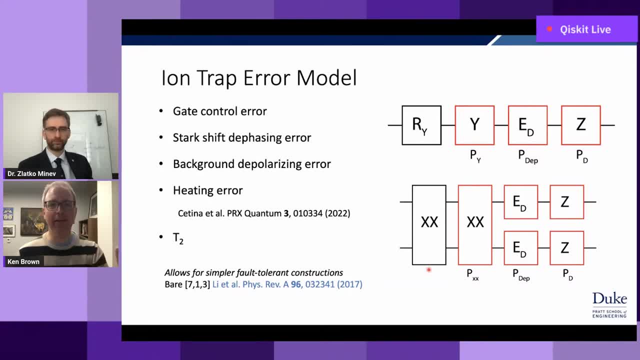 or it could be stochastic. So it ends up looking like a kind of poly error that's aligned along the axis of the gate And that will differ between different ion traps. So some ion traps they may suffer more from, like unwanted start ships. 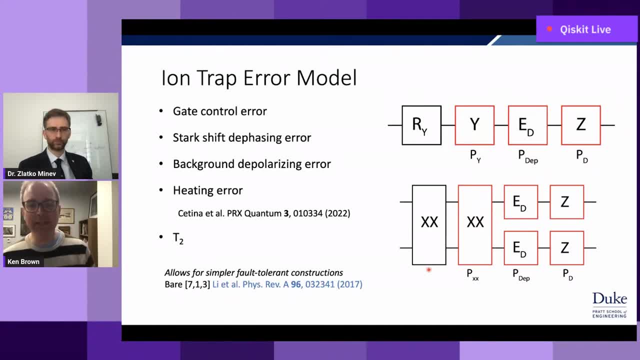 which lead to kind of a defacing T2 type of process. But in our experiments we really see errors that primarily look like a slight error in the gate And as a result we can actually use this to make simpler fault tolerant constructions. 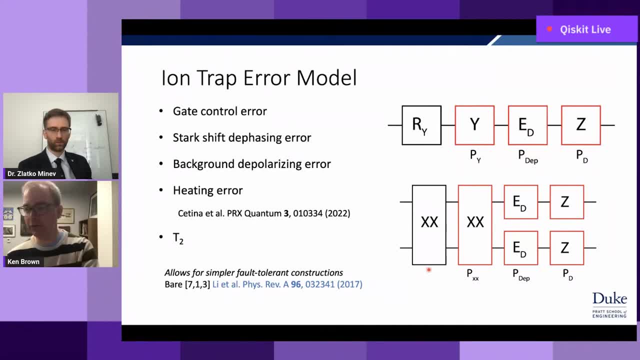 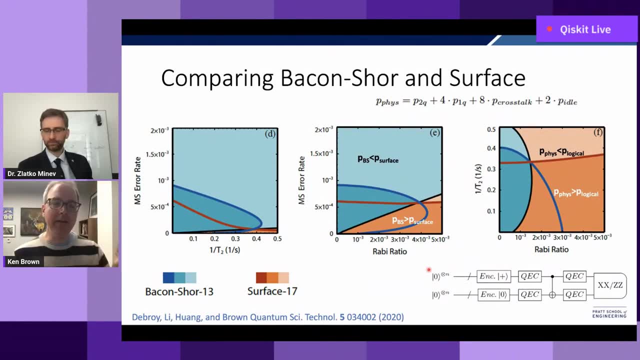 But in this case we're just gonna use this as our way to model which of these systems we should try to work on. So in these plots we compared vacant shore versus surface code, And one challenge, I think, is that once you start to have a real error model, 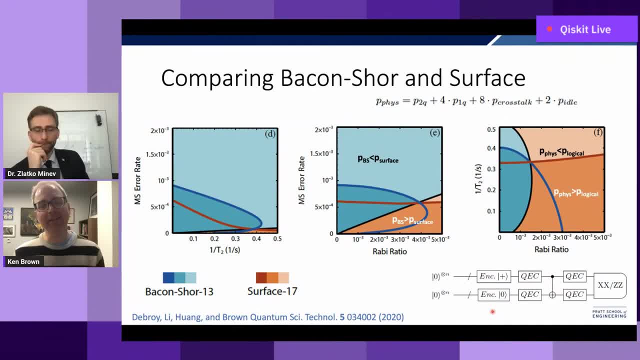 the idea of a threshold becomes really fuzzy, because there's not a single parameter that controls error, right, There are actually multiple parameters that control error. So the whole thing is some complex space, And so then because of that, it's kind of like: well, 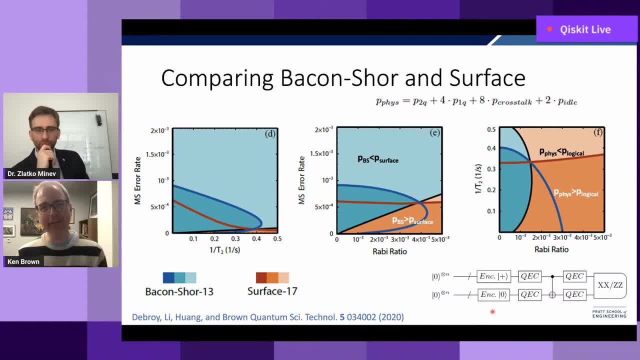 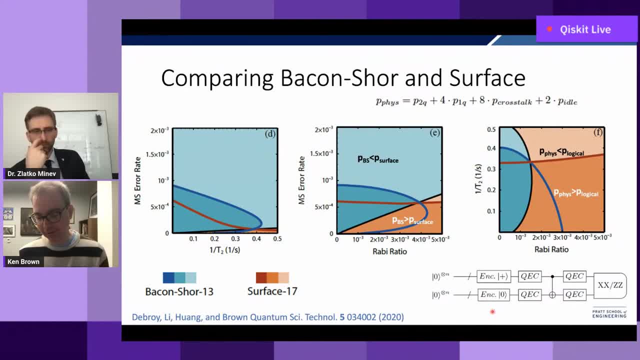 it's really hard to have a logical qubit live long, like to live longer than like the physical hyperfine qubit lives We're interested in. okay, can we make like, say, a better gate, for example? So what would be the cost of doing encoded logical CNOT? 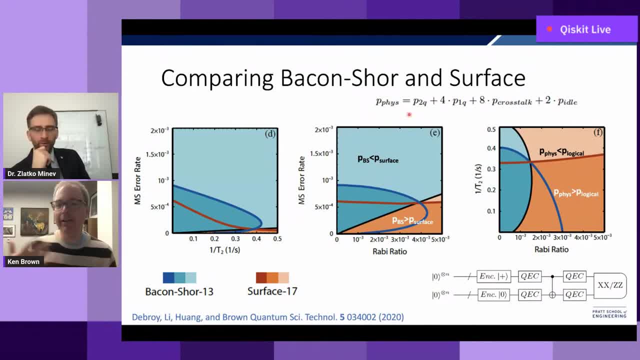 And then we have like a basket of errors which is the total physical error is somehow the two qubit error, These single qubit gates, any errors that may arise from crosstalk, any errors that may arise from memory. And then we compare here when the logical error 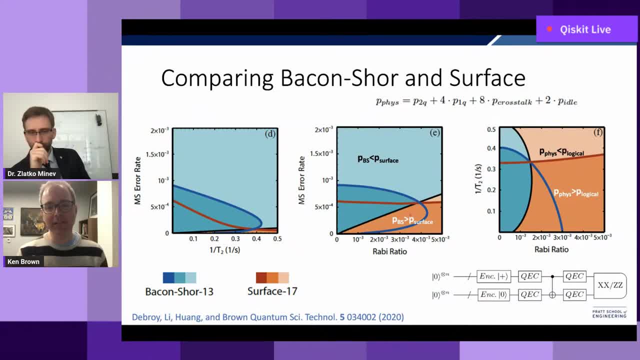 is smaller than the physical error, and that's corresponds in these pictures to the dark colors versus the lighter colors. So when the logical error is better, we end up in this dark regime, And so these dark colored lines represent kind of a threshold. 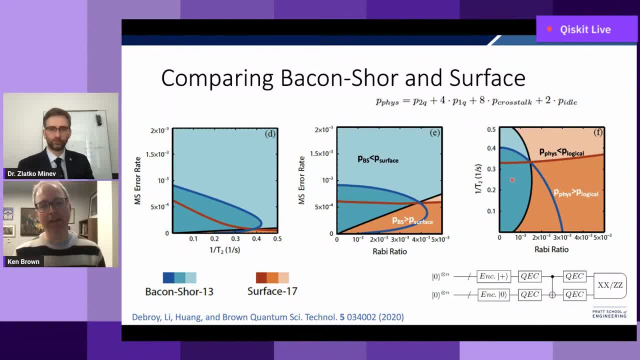 colored lines represent a threshold for those two codes. Now the blue versus orange actually represents when you should use bacon shore or you should use the surface code. And then in this particular thing we look at basically two qubit gate error, some kind of memory error. 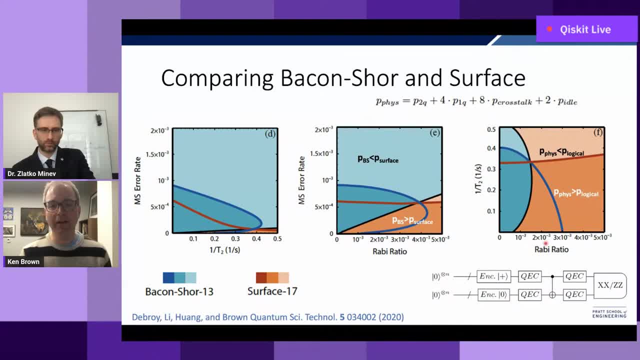 This is a crosstalk error And, depending on the values, the right code changes right. So that I guess that's my. the key thing I want you to take home from today Is that the right error correcting code really depends on your errors. 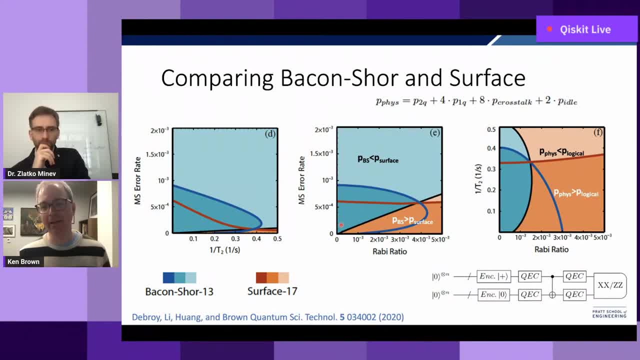 And the right procedure really depends on your errors And so the in the end. so in this case we see, for almost all regions bacon shore is good, unless we have a lot of crosstalk. So let me talk a tiny bit about that. 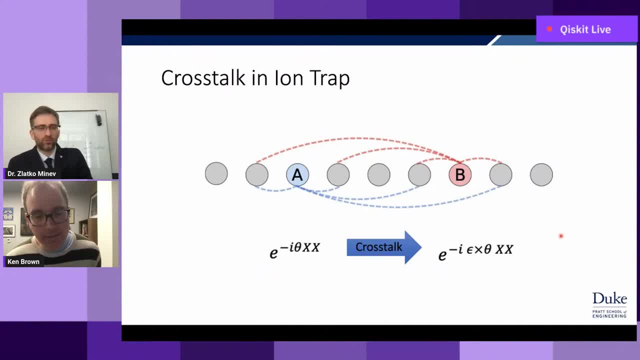 So for us, yeah, Ken, I was just gonna say perhaps that perfectly answers the question that we had from Hong Yao, which is: you know, is there a generally well-accepted threshold for the error rate below which we believe in fault tolerance? 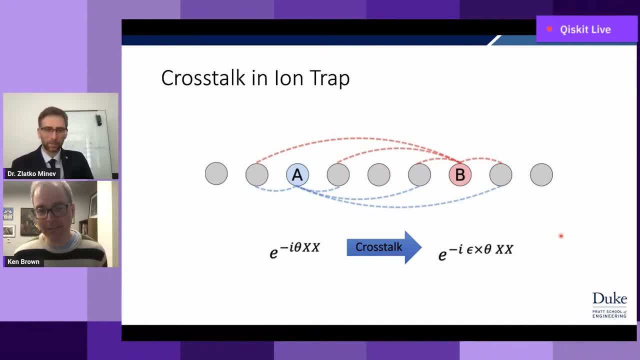 But I think maybe you're kind of hitting that on the nose here. Yeah, yeah, yeah, So you know. so we have this idea that you know: for the surface code, the fault tolerance threshold is around 1%- 0.7%. 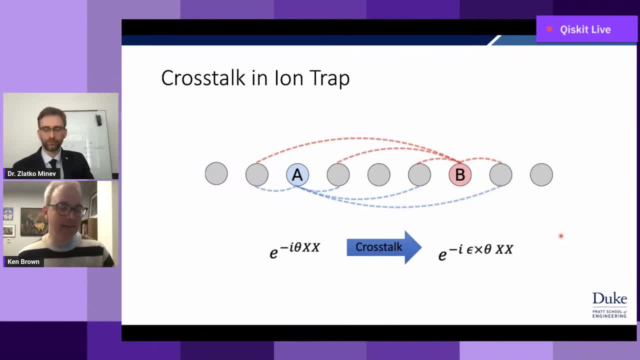 But those models really depend on the fact that you have one parameter P, which controls everything: Measurement error, two-qubit gate error, single-qubit error- like controls everything right. So in reality those errors will be quite different And the damage they do is quite different. 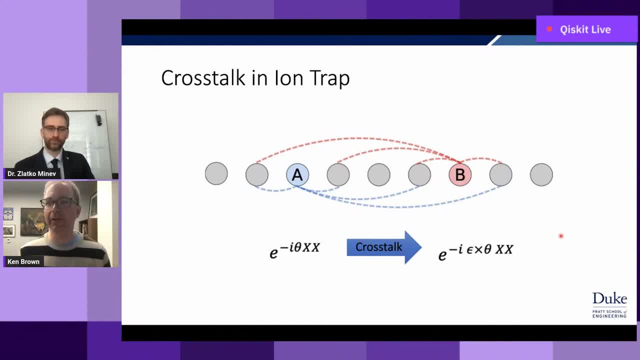 So, for example, in the surface code right, Usually you can suffer a larger measurement error than you can suffer a two-qubit gate error, And so once you move to this basket of errors there's really- yeah, it's hard to think about. 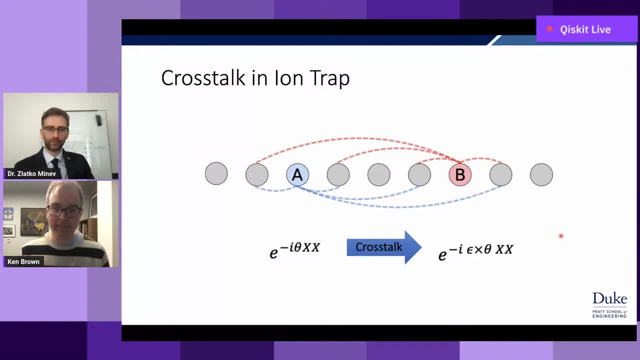 that single threshold is great, thank you, and thank you for the questions. by the way, feel free to post them in the chat guys. um, yeah, so in our ion trap systems, our basic gate is this kind of angled xx gate. um, and then, due to spillover of laser beams, um, we end up with unwanted, in this case. 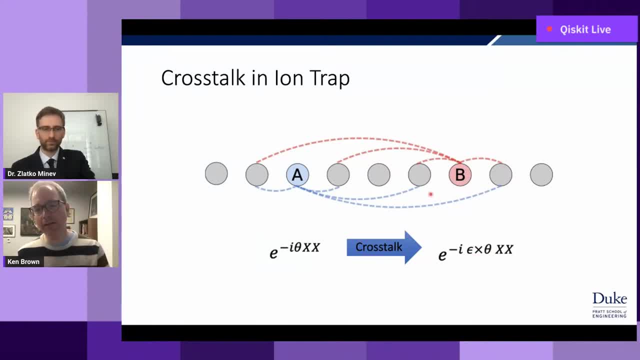 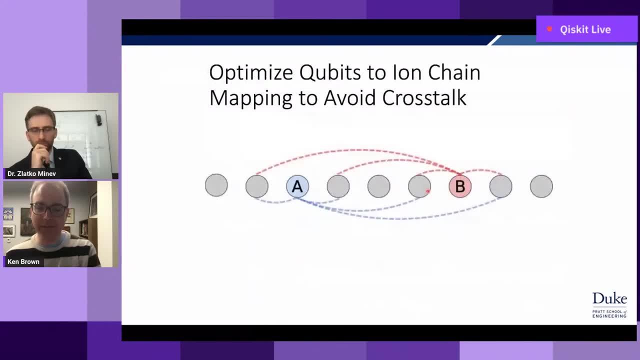 we imagine the phases are fixed but we get an unwanted extra two cubit rotation, basically between other other other gates. so, um, in the sorry, the plots that i showed you, um, those numbers are all based on an idea of actually using, um the chain reordering to get rid of crosstalk and 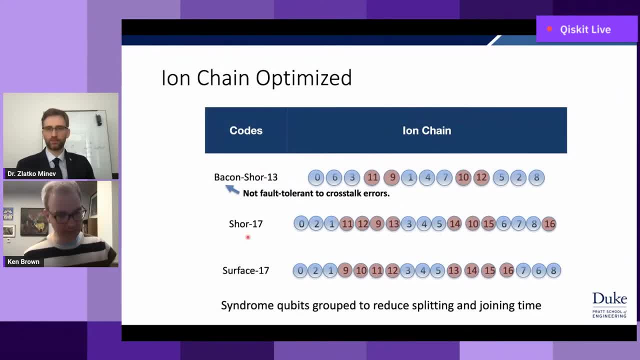 so what's kind of interesting is that for um, the shorter code, which i didn't show, the short and surface and bacon, sure you can see it in the paper. um, for the shore of the surface code, we can actually find an ordering that is fault tolerant, meaning that we can accept in. 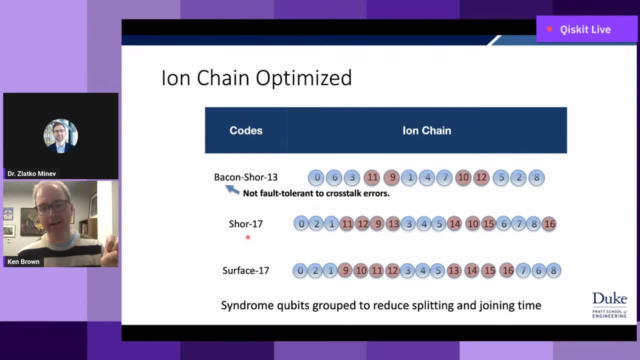 this case, a single crosstalk error, uh, without ruining our decoder. um, whereas for bacon, sure we cannot find an ordering, we don't have enough space, in some sense, to like shift the qubits around to have no crosstalk errors, but it ends up still being better. so, even though it's not formally, 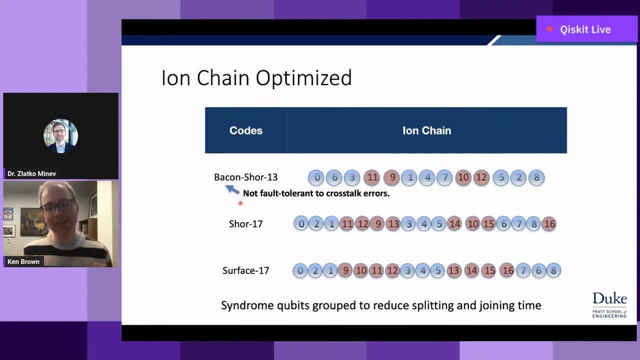 fault, tolerant to the crosstalk errors. for that, for that specific task of the logical c, not for most of those regions- it is better and, of course, as crosstalk becomes worse, um, that's why the surface code, as we saw, becomes more desirable in this, in this specific case. now, 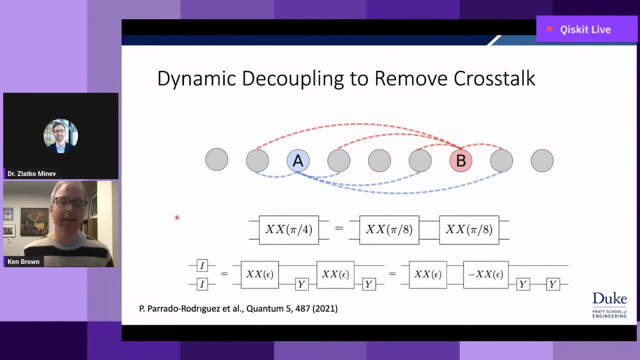 of course there are other ways to try to get rid of crosstalk and, for example, there's some nice work for marcus miller's group, which basically says we can spin echo away by applying: um yeah, basically spin echo y turtle pulses to the qubits that we don't want to have. talk to our. 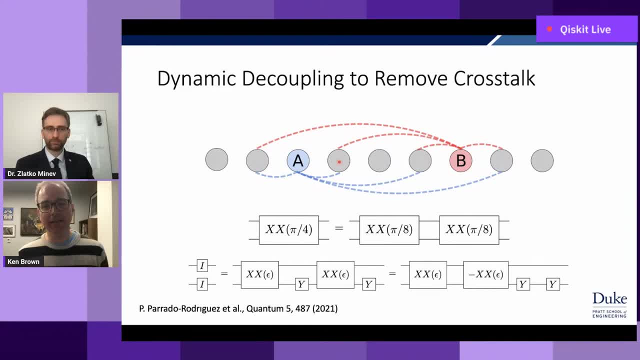 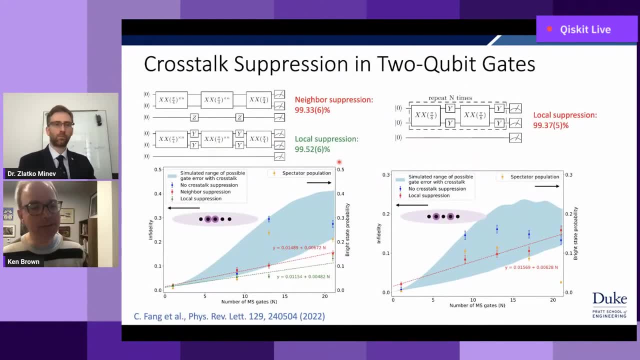 main qubits, um, and then, and then, and then, if it's, if the error is coherent, it it vanishes. so recently, in a nice experiment again with jun-san kim's group, uh, we, we shifted to sort of a interesting scheme, which is shown here, where we kind of do um, i don't know what best thing to call. 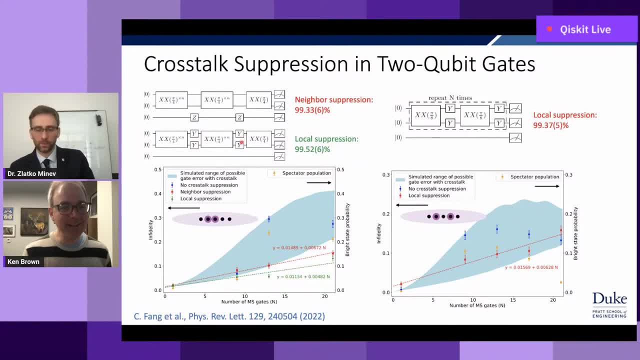 it is not spin echo. uh, we applied the grosso order error with some speen echo spell route example. But we apply these two Y gates, which don't do anything, to this XX kind of two-qubit interaction. But what it does do is it cancels out any unwanted crosstalk. 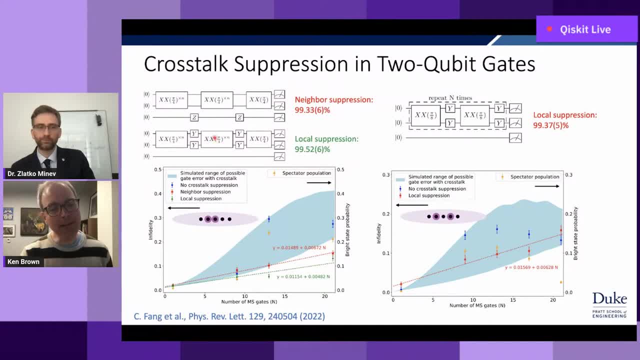 It does the spin echo on the crosstalk side, And by applying it to the qubits that are engaged in the gate and not the qubits that are neighbors, we can actually suppress all of the neighbors. And so, in these plots below, what we find is this local suppression, which is the green bar here does better than these neighboring suppression. 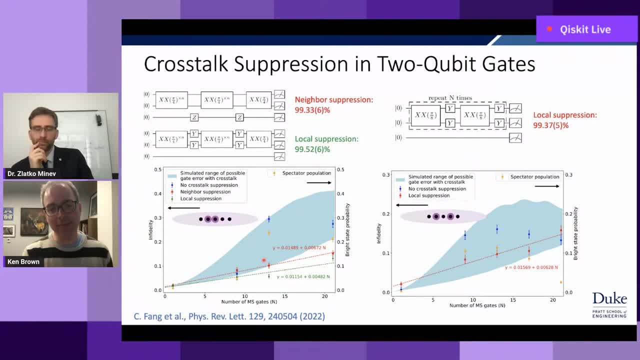 And, of course, if we don't do any crosstalk suppression, the amount of error that happens on the neighboring qubits, basically through the neighboring qubit being excited, can grow in this kind of envelope way because it is an overall, coherent error. 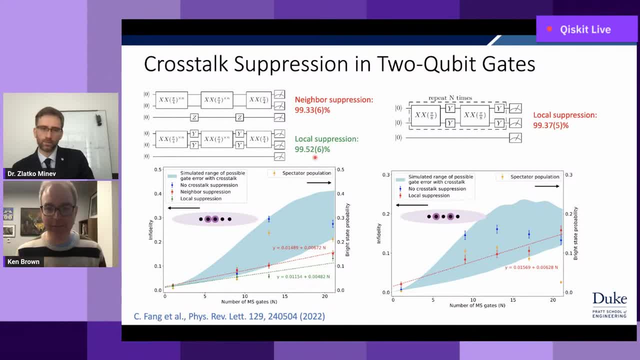 So key thing again is we're able to have very good two-qubit gates. And the second thing is that that axis where crosstalk is increasing isn't really our problem, And if it was our problem we should be able to remove it through this sort of coherent control. 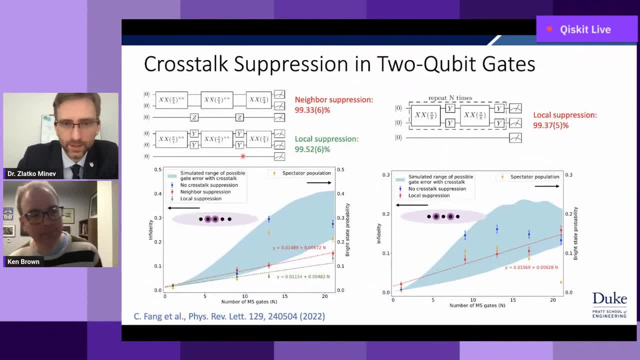 So just to make sure I understand, so on, like this local suppression plot on the second wire you have a Y gate because it was, did you say, because I have the type of CZ interaction with the spectator right below on the third wire that's going to flip and cancel that one. 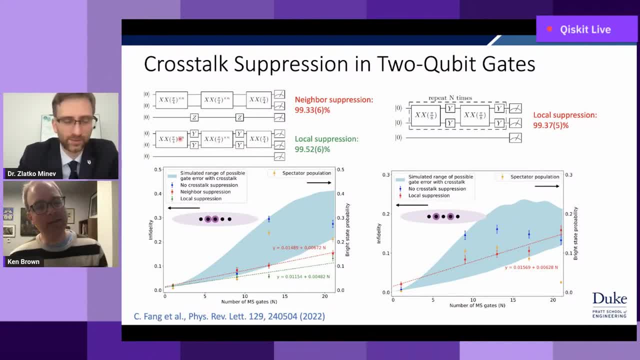 That's right. That's right. Okay, And the key thing is- the other kind of subtle thing is that the real interaction on the spectator qubit here, or yeah, it doesn't want to interact, right- is a sigma phi in the XY plane. 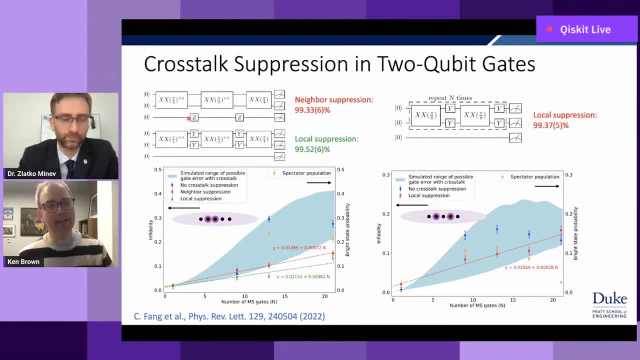 So then the Z will work fine because we know it's sigma phi. But here, because we know really well that the qubits we're interacting with, we've chosen that phase to be X. Then this Y works really nicely And you don't need any extra Zs on the third qubit. 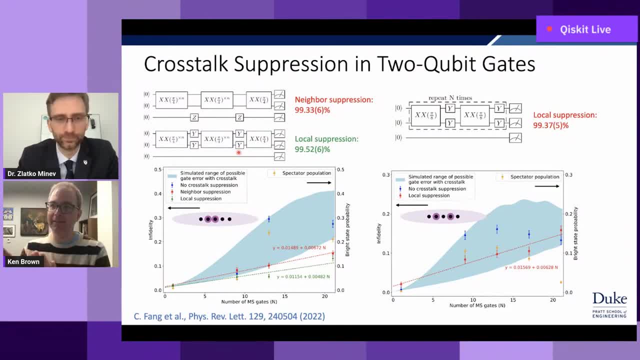 No, No, Because they, because they, yeah, because the angles cancel away at that qubit. And so in this limit of three qubits, it, you know, it looks maybe cheaper to do this, But when we look at the actual system there can be. 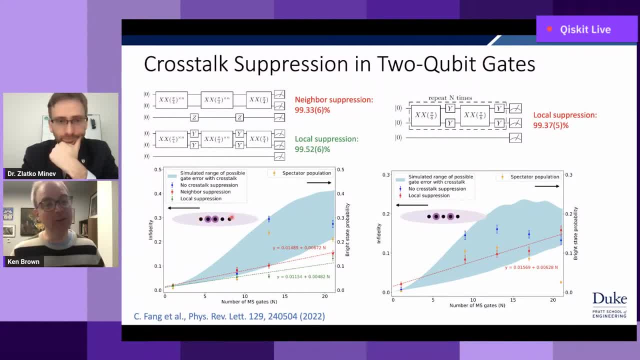 There can be crosstalk onto one, two, three other qubits And by shifting to this region we actually only have right. we only ever have to talk to the qubits we're talking to And on the spectator qubit here. is the T2 star an issue or is that totally negligible? 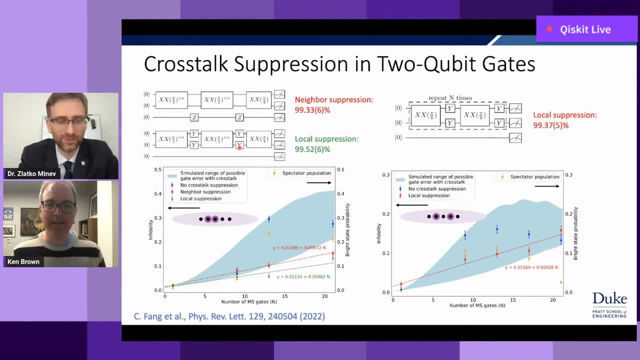 It's totally negligible. It's a bit different from super connecting qubits in that sense. Yeah, Yeah, Yeah, I think that, yeah, I will say generically when I'm talking with super Connecting qubit, uh, people, I think that's like the biggest, the biggest difference, which is our memory is basically good. 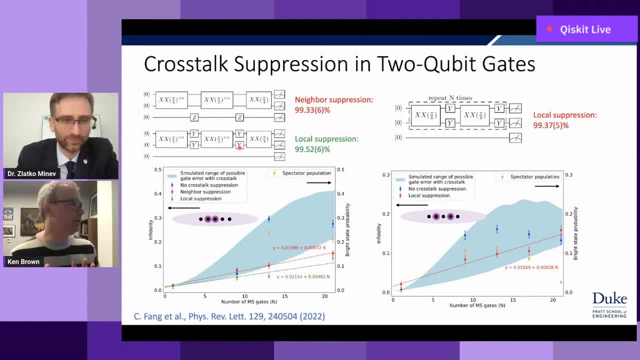 Um and so so. so the you know superconducting qubits. in your ideal case, you get to the point where your gates are just like, say, T1, limited Um, but that T1 is basically the same whether you're applying a gate or not applying a gate. 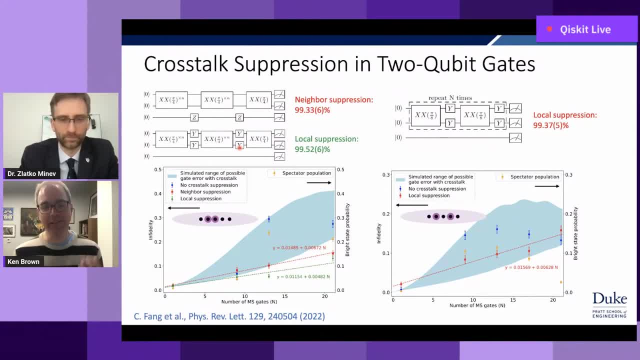 But for us, when we're not applying a gate, the qubits are really just Good. basically, it takes me. it takes many, many gates for the error to accumulate, um for there for a memory error to be equivalently bad. 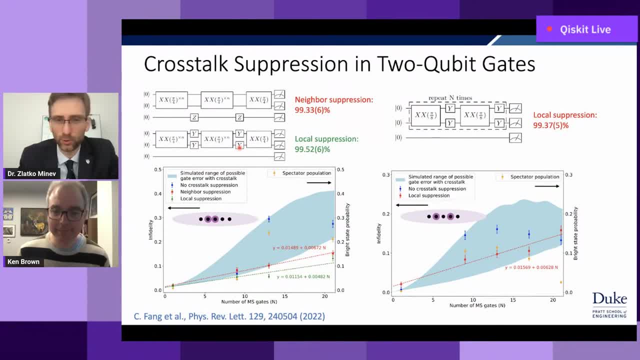 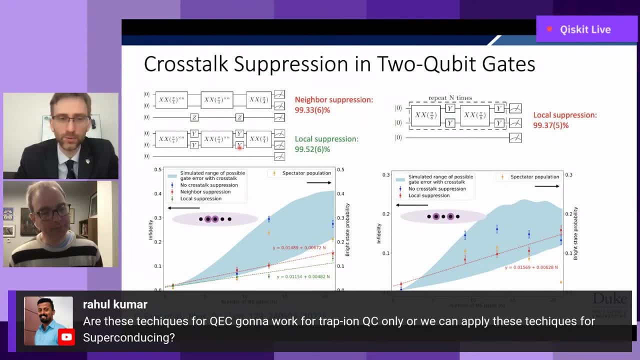 And quick question from the audience here, from Ro Khumar um. are these techniques for quantum error correction and the kinds of things you're showing now going to work for ion trap quantum computers only, or can we adapt them to, say, superconducting devices as well? 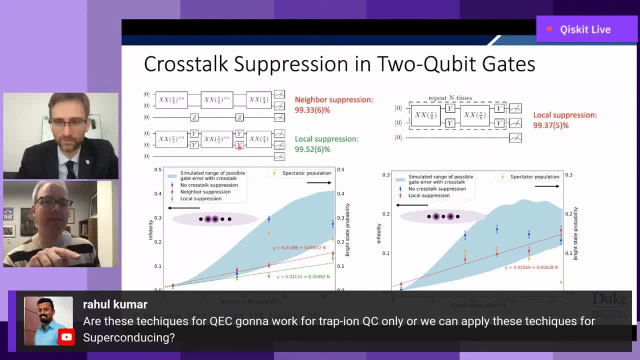 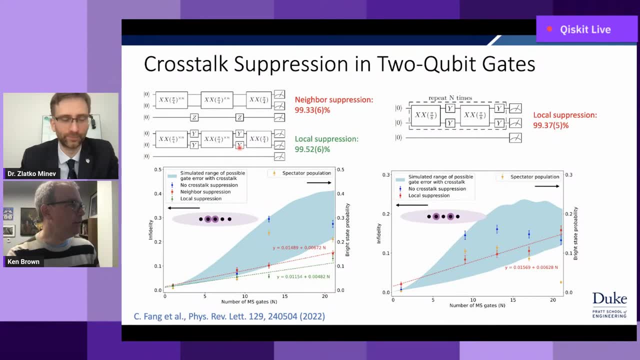 Yeah, So this one, um this, this idea of kind of a local suppression should work fine for superconducting qubits. Um so imagine you were doing um like: imagine you're doing like a cross resonance type of gate and a superconducting qubit and you have like an unwanted additional coupling to however many other qubits due to some- um, I don't know some chip mode you weren't thinking about. 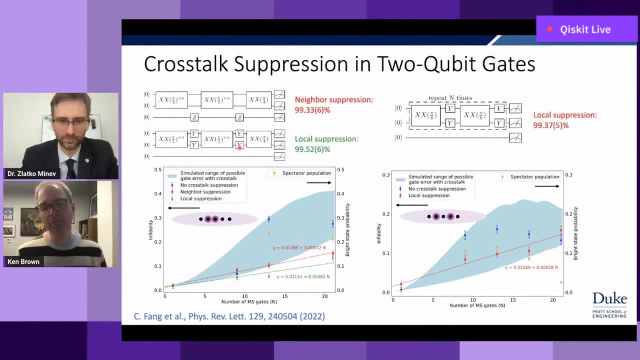 Then this kind of coupling- yeah should, yeah should- in principle work because it just relies on the fact that I Find Something that commutes with the two qubits that I want to have something happen on, and then we'll anti-commute if, if, if there's this um yeah, some neighboring piece, but then it does get into this question about the um coherence part, right? 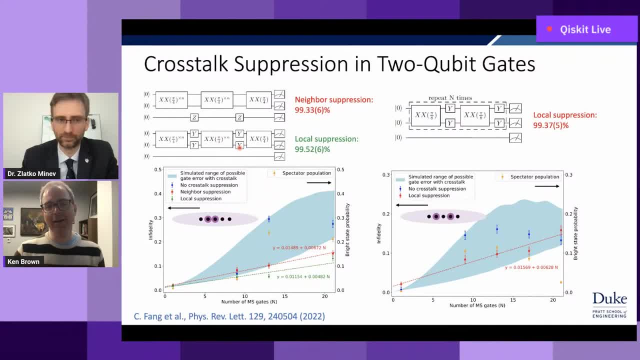 So that's only true if that dominant error remains coherent. So as, like I mentioned, like if the defacing is too fast, then it won't help you Like you really need it to be. you need the defacing to be slow relative to that time scale. 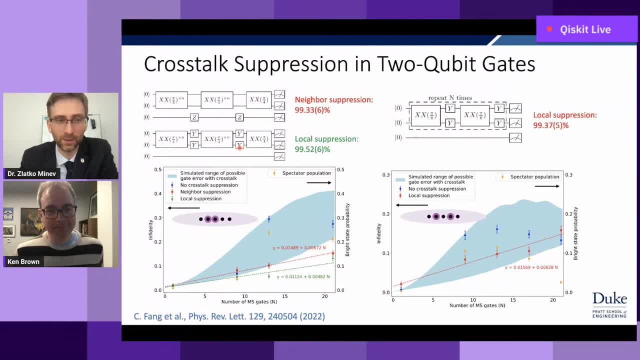 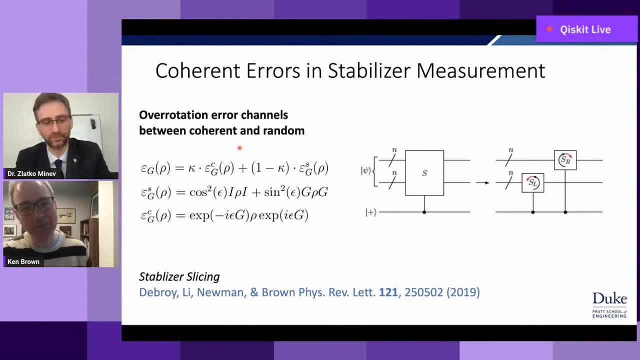 Right, Awesome, Yeah, We worked very hard with Coupling here sometimes. Thank you, Ken, Yeah, So so I just want to keep pushing. So on this, this, this coherent errors piece, Um, so we, we have kind of a simple model we use um to move between stochastic Pauli errors and coherent errors. 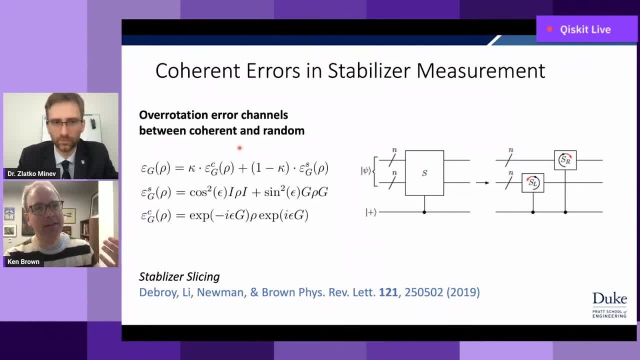 and then i just want to say for for people thinking about it, the the difference between these two things is really a question about time scale. so if the noise in your system is slow relative to your gates, it seems like a systematic rotation, and if it's super fast relative to your gates, like you can write down the same physics but that super fast. 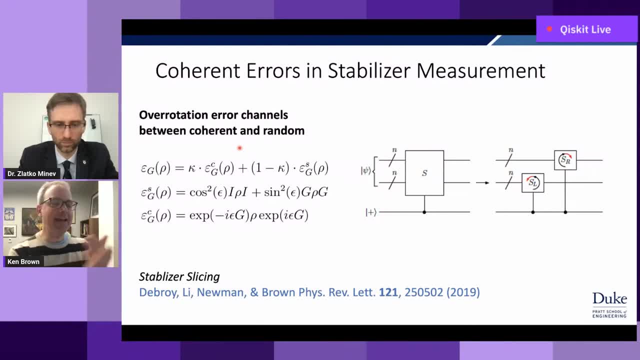 part basically averages it out, because you can't. you don't have any access to where your gate stops relative to this like fast dynamics. so we have this model where we basically um extrapolate between a system which is purely an extra rotation and a system where it's. it becomes just this: 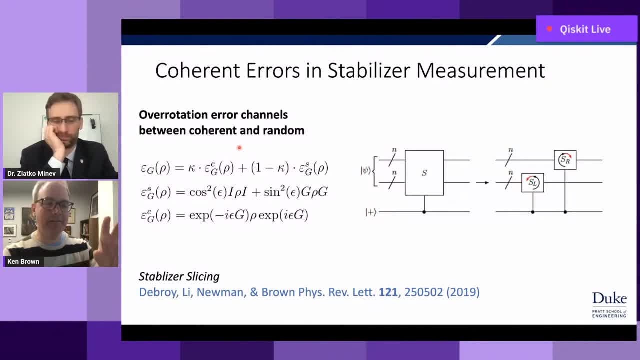 stochastic ing and then our, our like conceptual models. we just think about it as a gate. so if we do the gate perfectly, we just get the gate. we have a little bit of epsilon. it's like we do a tiny over gate. and so my student um dripdo, yeah, and we on a mic. 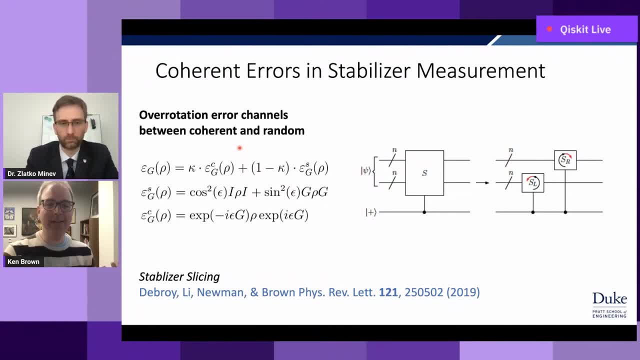 basically had this idea: well, if somebody gave me, um a control left and right part of a stabilizer, if i put them together it would actually cancel this kind of coherent error. um, and then normally that's not so useful because your stabilizer, um, you know, your stabilizer will. 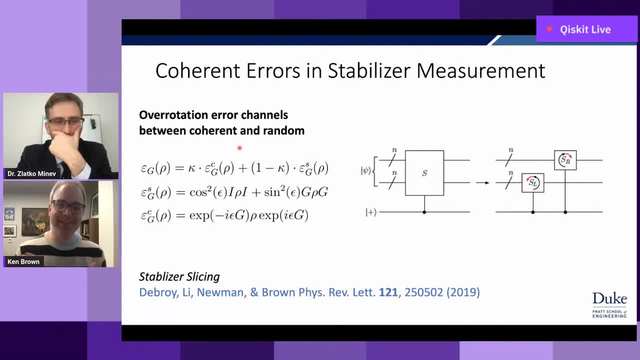 be like weight four. so these two things are like weight three interactions and you probably don't have that kind of. you don't have like a three qubit native three qubit interaction in your system most of the time. um, so that's kind of what we're trying to do here is we're trying to figure. 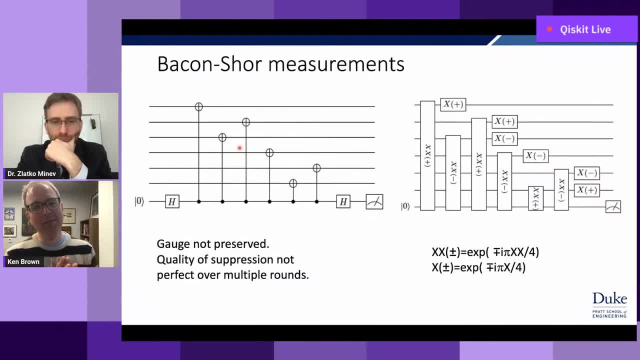 out how we're actually doing the same thing. but what's funny is for bacon, sure? um, this corresponds, because of this connection, to gauges. back to the gauges. so now i'm going to measure this weight six stabilizer- i'm going to pick this- really weird. 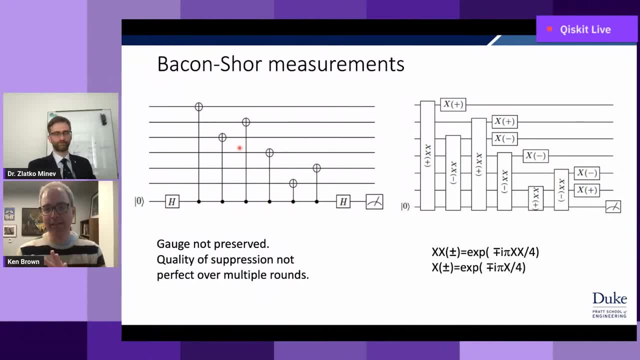 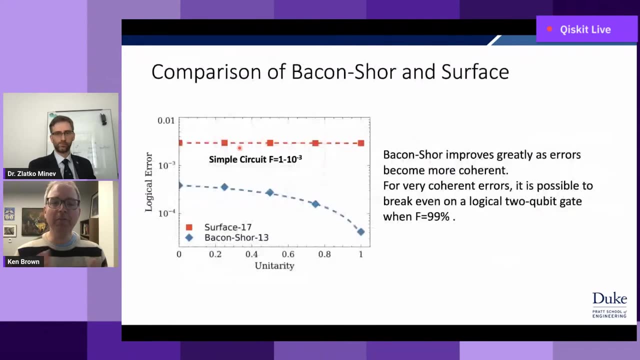 order because i want to make it follow the gauges, and then i use this idea of stabilizer slicing to make the entangling xx interaction be positive or negative. it will actually cancel out the coherent gate error And, kind of remarkably, if on the left side is purely stochastic error after gates. 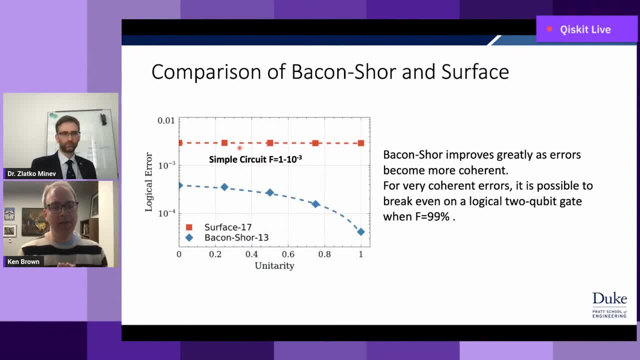 and the right side is purely coherent error. we find that the Bacon-Shore code. so in this particular set of errors we have- and this is just a preparing, doing an error correction and measurement circuit, As you saw, for most of the region. 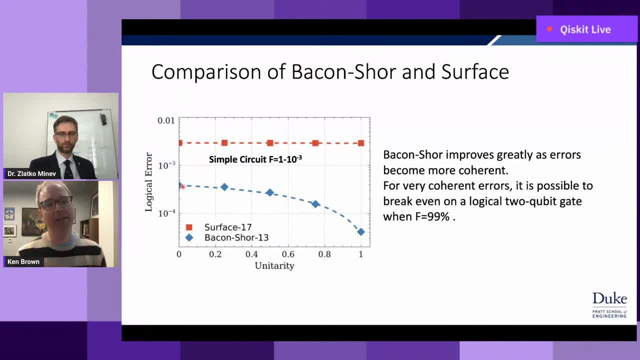 the Bacon-Shore code does better than the small surface code. Kind of surprisingly, surface code became more or less in this model like, independent of how stochastic or not it was. but the Bacon-Shore code really gained as the errors became more coherent, which is nice. 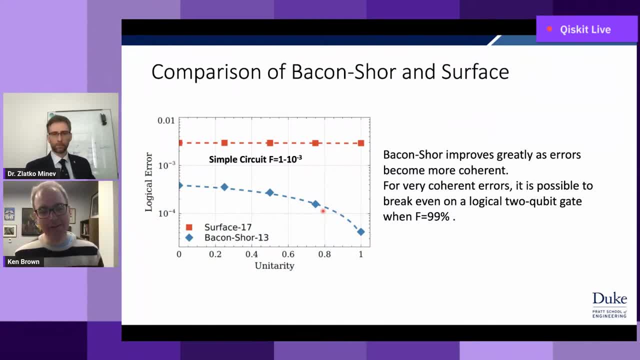 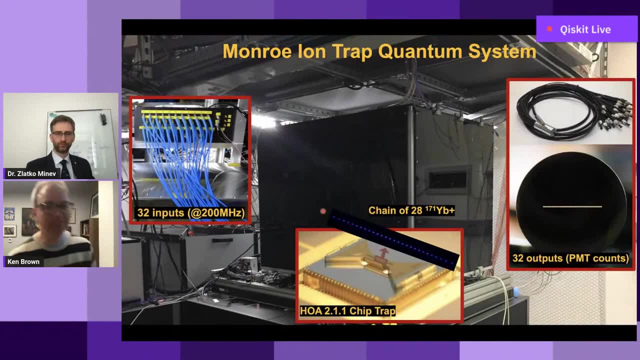 And it's like an example of how, if you have coherent errors and you know about them, you can do a lot of good work. If you don't know about them, then they are bad. So now we talked with our good collaborator, Chris Monroe. 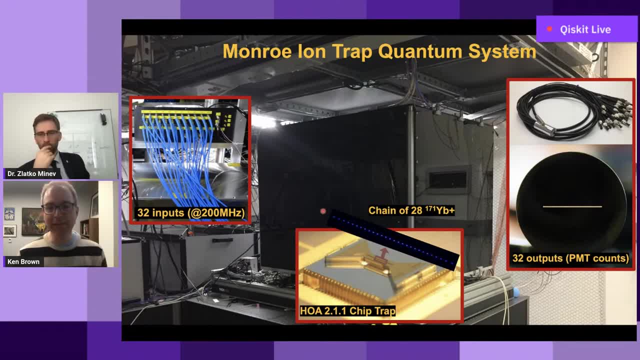 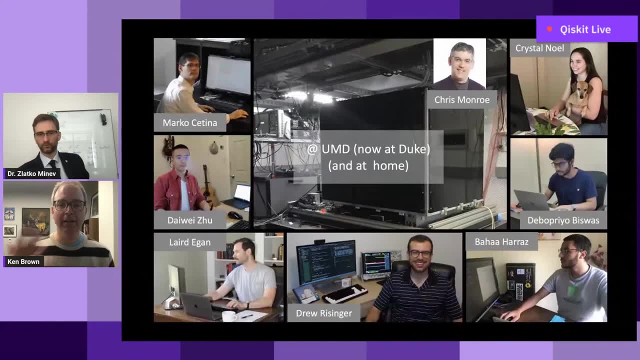 about trying to run some of these Bacon-Shore experiments. This is the setup which was at University of Maryland when these experiments were done, but now it's here also at Duke. Again, here's Chris and his team who worked on it. 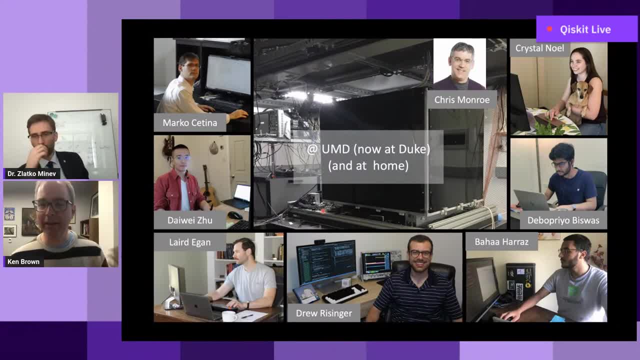 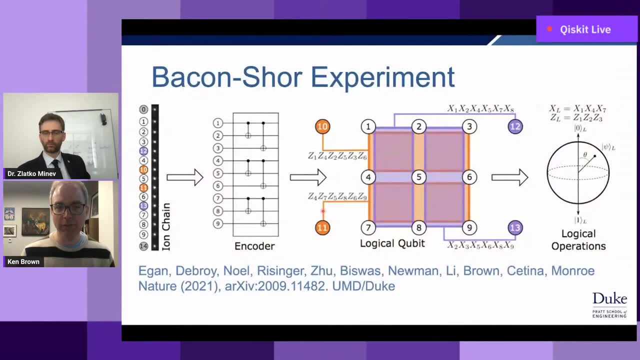 Marco and Crystal were research scientists and postdocs respectively at the time, and now they're both also faculty here at Duke. And yeah, so the idea is we have these 15 ions. We just take 13 of them to be our computer. 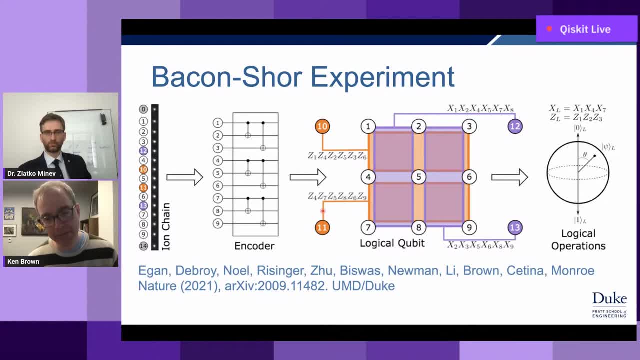 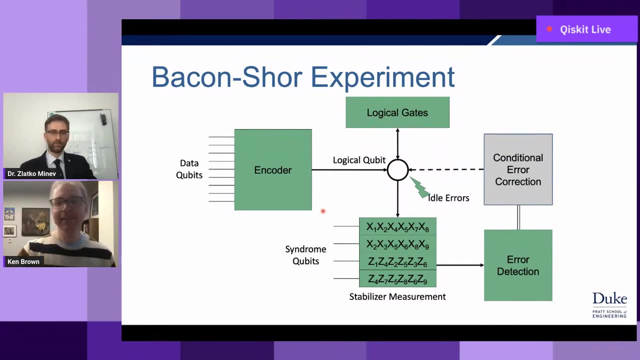 An advantage of Bacon-Shore is that you can prepare the logical state unitarily without having to do measurements. We then check these stabilizers and we look at doing logical operations. So in this experiment we were able to do everything except for conditional error correction, where you would do multiple rounds of error correction. so we 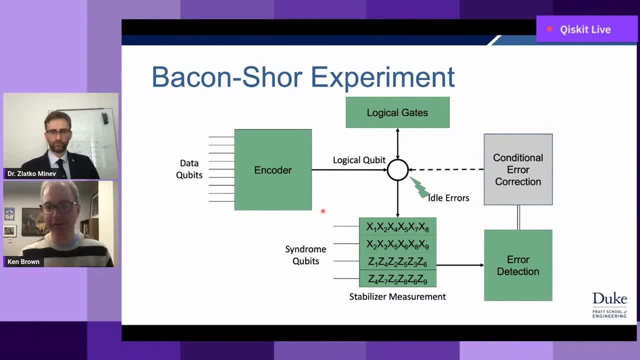 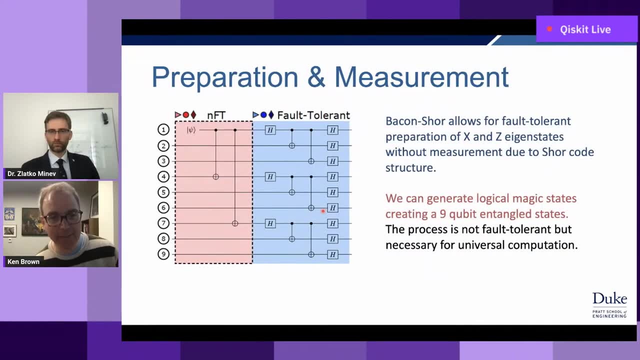 can encode, you could do logical gates, you could measure syndromes, you could do error detection and this. this, this last part of the initial error correction was missing. so the first thing we examined was, um, the difference between, say, not fault-tolerantly prep and fault-tolerant prep. so in fault-tolerant prep we again, we actually just generate these. 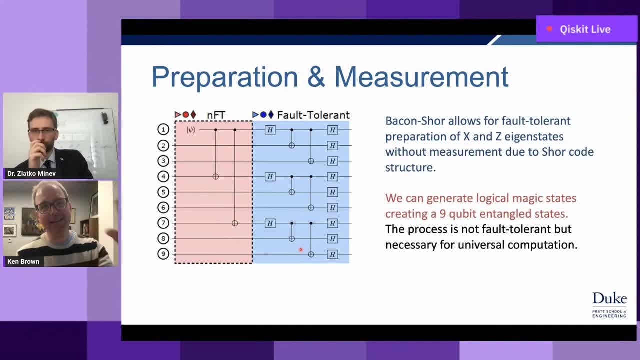 three ghc states because of the concatenated nature of the short code. basically, each of these blocks will fail independently and we can have one block fail and fix it and still have good logical information. if we want to make an arbitrary state, we need to make that state. 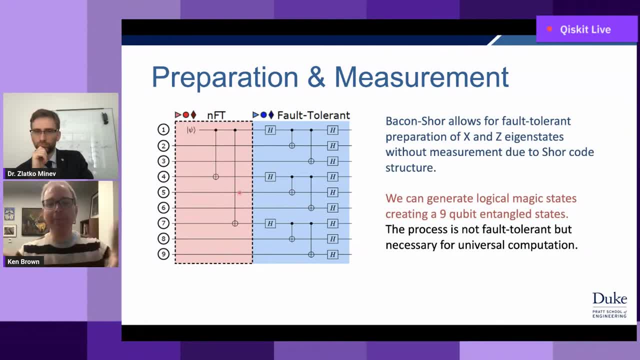 and then we need to make these two control knots to then propagate that information to these three pieces. you can tell this is not fault tolerant, because obviously if the state is bad you're in trouble, um. and the second thing is, if you have these, uh, if either of these control knots go bad, you're also 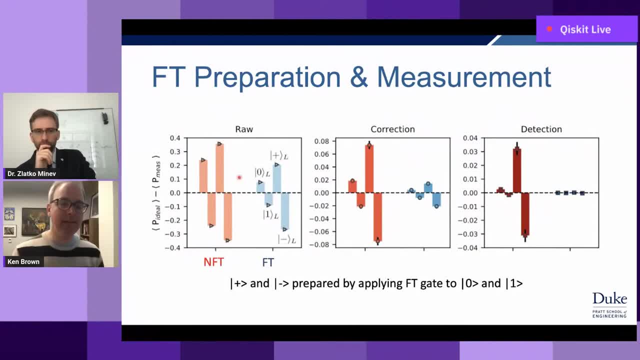 in trouble. so what we saw is, if we just took the non-fault tolerant preparation to make plus minus zero and one versus the fault tolerant preparation, if we just looked at the expected outcome of z or x minus what we measured, we actually see it's not so bad. they they line up the way you expect. 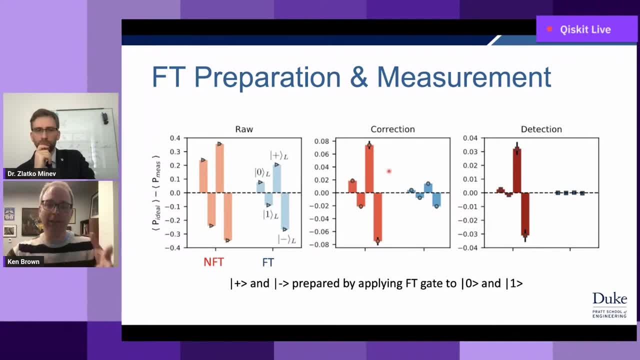 but the cool thing is then move to correction. so then when we look at the measured data qubits, we get syndrome information in that information and we're able to then do a correction and we see that the, as expected, the fault tolerant procedure leads to a much lower span. and if we go all the way to detection, where 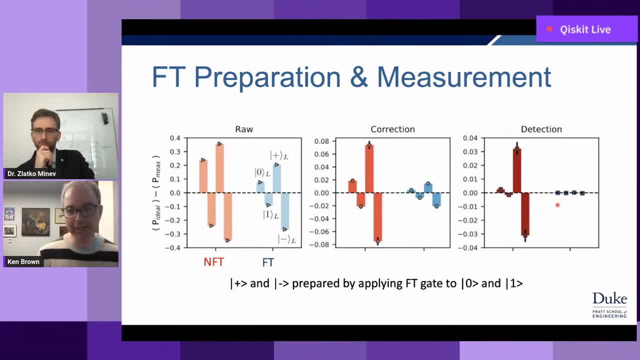 we reject any. um yeah, we reject any states that that fall outside of the code space. uh, we actually saw. no, there were no residual errors in the default one away. um, we want to prepare other states, of course. so, for example, if you want to do magic state, 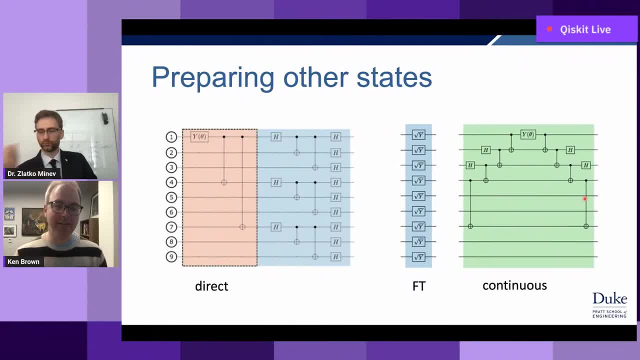 distillation um, you need to make states that are not um, c or x um and so we compare, doing, you know, rotations between the z and x states in a fault tolerant, transversal way, versus directly repairing some state on that axis, versus applying a very complicated um. 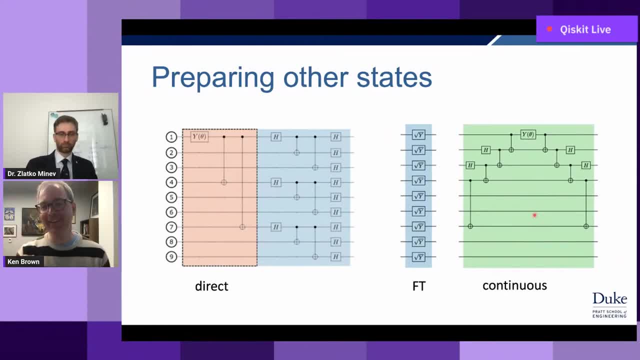 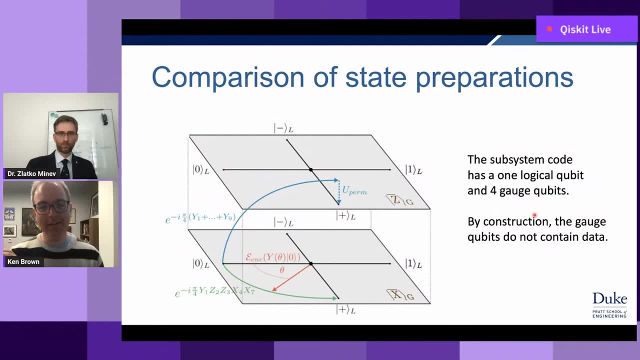 yeah, you know multi-qubit uh unitary, which does the transformation on the very basic right, and so i think we're able to get all of those of the state unitary values into one and separate state uh. but then we also have to be able to look at the 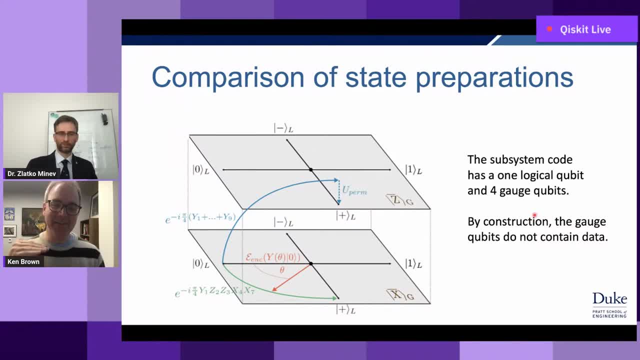 right range of what we want here and what we're trying to pull out of this um. everyone needs to be able to get all of those things and get an unitary state of their own um, so we're able to go from just checking the state of the Yorkshire or the South of the state and then going from 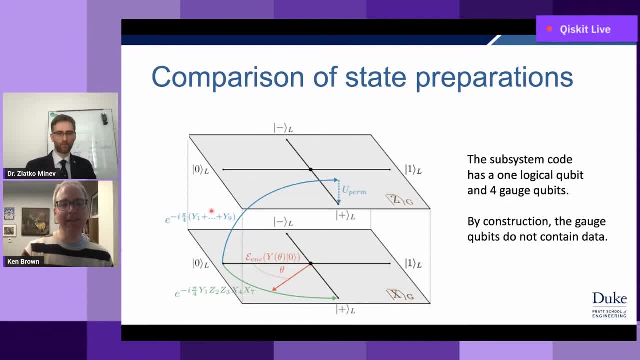 just stronger elements to more birds, open tests, and so we get all of those, some of those states. that's one of the reasons why i think this is is really important, because then we can actually make other states more flexible, or you're able to take some states away from each of them and then 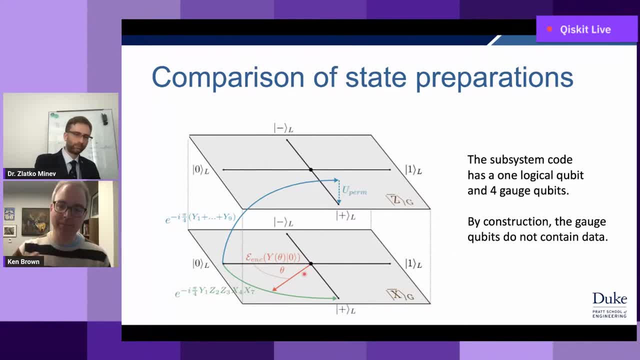 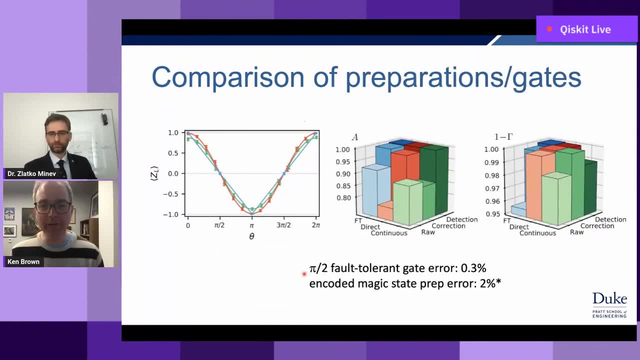 it's like: what are some of the options that we can do to take in the state space? that's really important. this logical operation all happen in the same X gauge And then what's nice is that actually all of them work pretty well If we just look at the points. 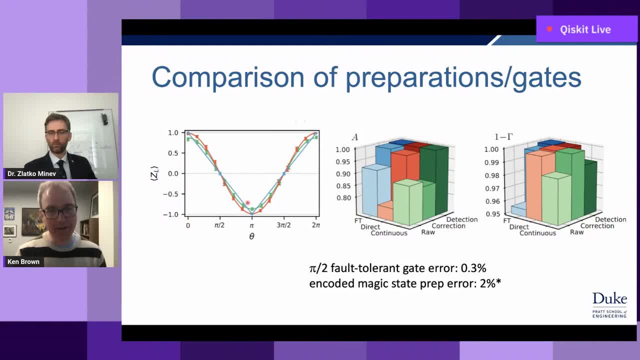 so the fault tolerant one can only be at zero. pi over two, pi, three pi over two, two pi. And then, if we fit them to kind of basically a oscillating cow sign with some decay, we see, the decay is quite low, The amplitude is quite high. 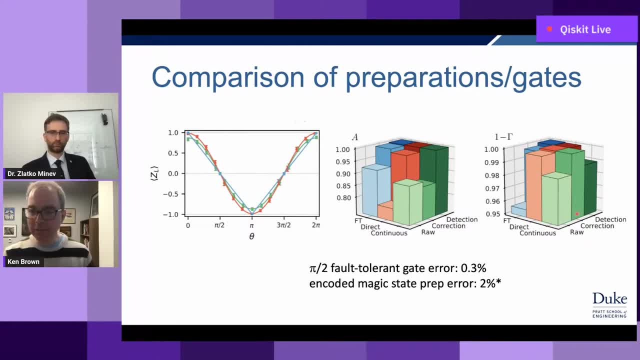 particularly after we do correction and then detection. And then I think this one with the continuous is quite nice because you can see the correction helps quite a bit. The detection actually hurts you a little bit in that in some sense weight two errors are a little more likely. 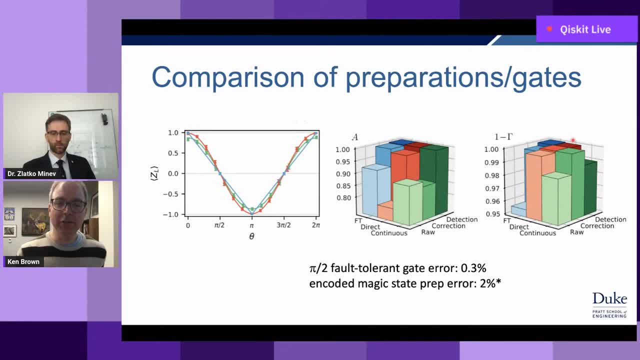 because of this large unitary block. The direct preparation is the most important part And it looks like, based on our measurements, that we can prepare the states who would need to do magic states in the story of the installation- with an error of about 2%. 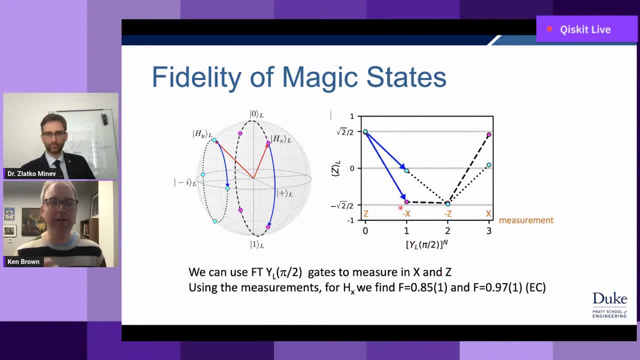 Yeah, so this is an example of how we calculate that. So we just look at these different points. The one challenge of fault tolerance is we can't measure any direction. right, You can only measure directions. Yeah, you have to measure directions in a fault tolerant way. 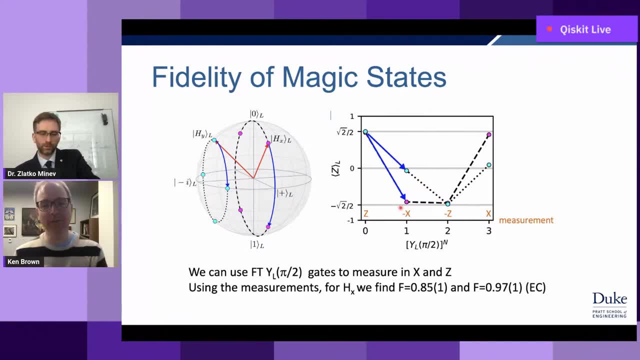 and for Bacon's short answer to all these codes. really, you can only measure X and Z, and measuring Y is quite challenging. And so from X to Z there's a lot of room for error. X and Z we can get a bound on, kind of what we expect the fidelity to, So then we're able to do. 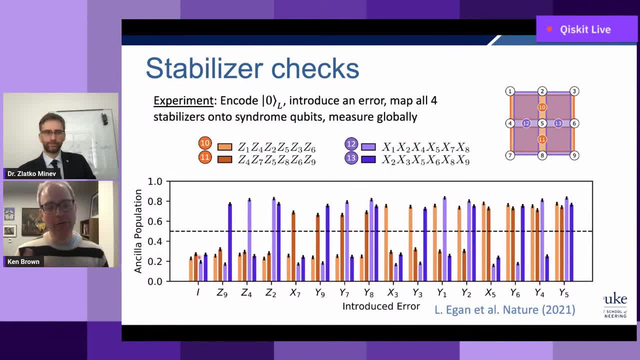 stabilizer checks. So this is what happens if we don't do anything. We see, you know, kind of 20% of the time. Ideally, if there were no errors, these would all just be zero here for all four checks. There are errors in our system because it's a real system, and so we see 20% of the time. 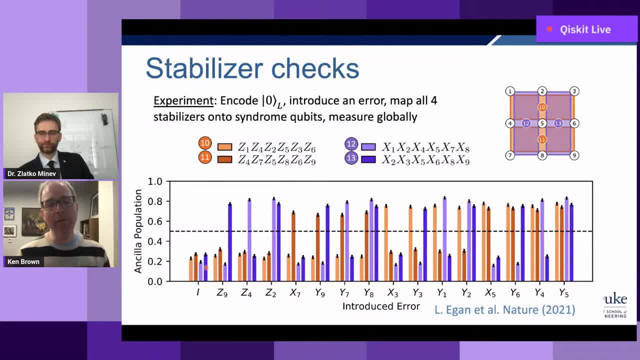 something might click inappropriately, But when we add in different errors we get the right pattern. And then I think this is like one sort of big difference between kind of quantum simulation type experiments and error correction. So in quantum simulation you can use all kinds of, say, error mitigation techniques to extrapolate to what the right answer. 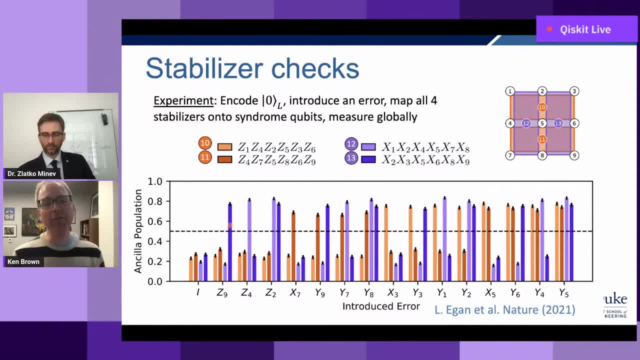 should be, or like: push you to that answer, And so here that would be equivalent to basically the same thing that you would do in a quantum simulation. You can use all kinds of error mitigation techniques to extrapolate to what the right answer should be, or like: push you to that answer, And so here that would be equivalent to basically: 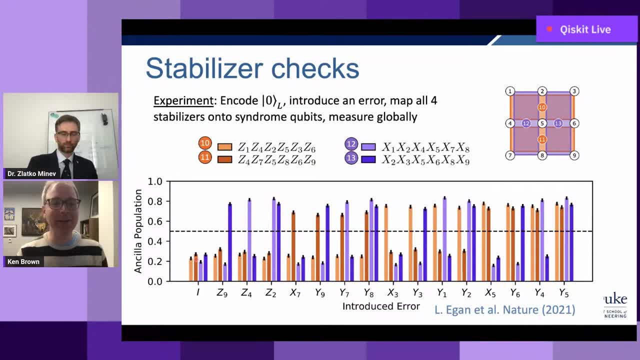 you can use all kinds of error mitigation techniques to extrapolate to what the right answer should be, or like push you to that answer, And so here that would be equivalent to anything which is below half. you basically suppress to zero, and everything which is above you express to one, And then you would see that this looks perfect. 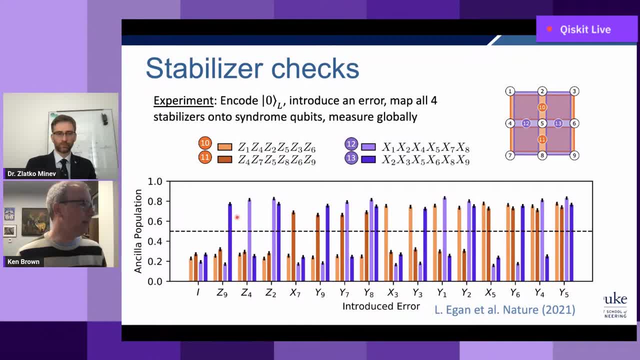 But in error correction it's a little bit tougher because we have to- yeah, we're kind of forbidden from doing that- We have to accept. just accept the bit that we get, And I think that's one reason why- yeah one. I find it one reason why I find it hard sometimes to convince. 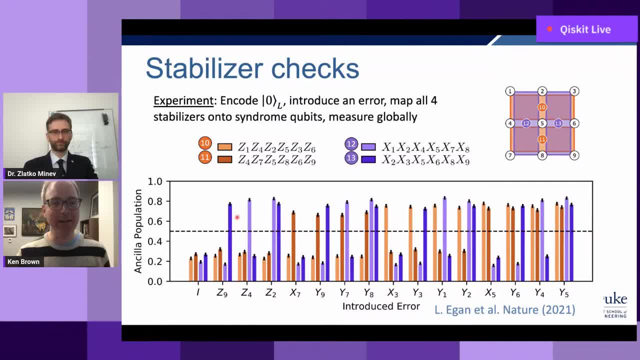 people to do error correction experiments because you have to just have to accept the bits you have. And I think that's one reason why- yeah one. I find it one reason why I find it hard sometimes to convince people to do error correction experiments, because you have to just have to accept the bits you have. 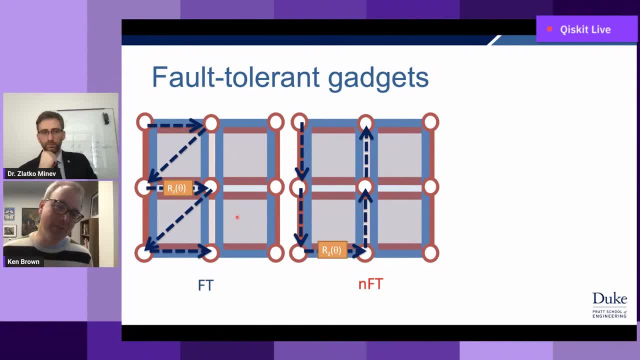 Now, at the beginning I talked a lot about our one of our main results is this new fault tolerant gadget for these compass codes, And we have, you know, this idea that you should follow the gauges and then we imagine there's going to be a z error here, versus kind of a naive way of doing it where. 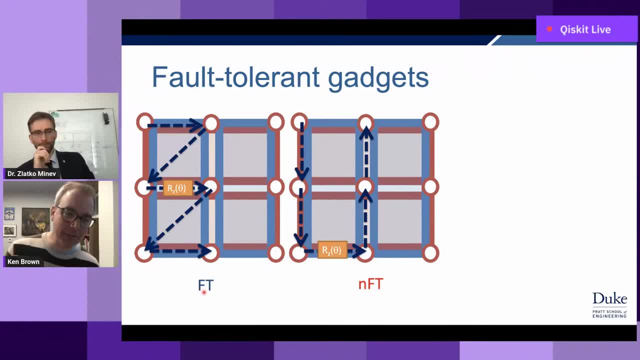 you run around like this And from a design principle, I'd call this one fault tolerant and this one not fault tolerant. The referee- one of the referees- asked us like well, you haven't proven that it's fault tolerant. So I of course wrote back: like it's just a design principle. we just do this design. 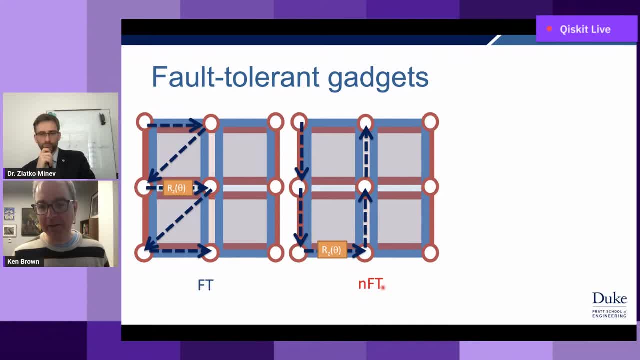 And I asked Laird, who is the lead experimental author, to just run an experiment where we inject this coherent theta error And the results to me were kind of were very interesting, so that the key result from my perspective is: at no extra error, there's basically no difference. 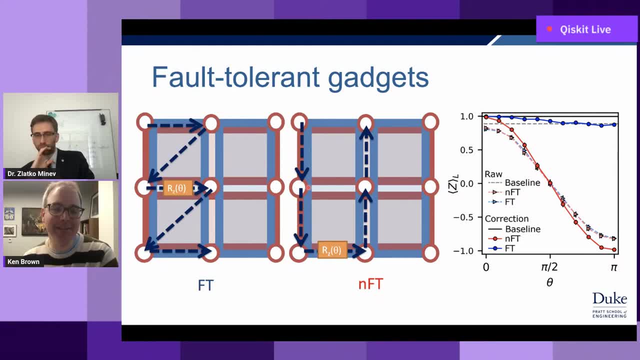 And, and what I'm trying to do is I'm trying to make sure that I'm doing the right thing. Why is there no difference? There's no difference because this z error, which corresponds to like an unwanted dephasing error or a stark shift, 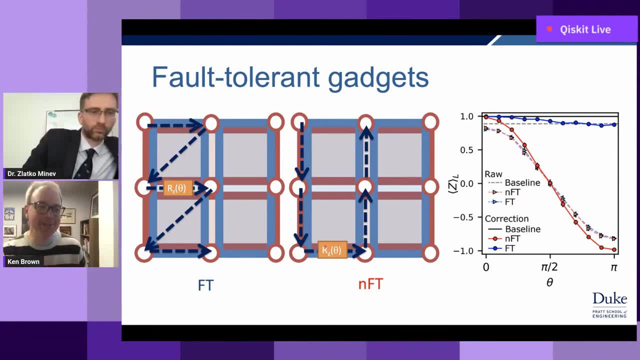 we just don't have. So we've made this fault tolerant circuit to something we don't have to worry about. Now, if we make this error happen, then we get the what you expect, which is, if you don't do correction, the probability of the parity check giving error is zero. 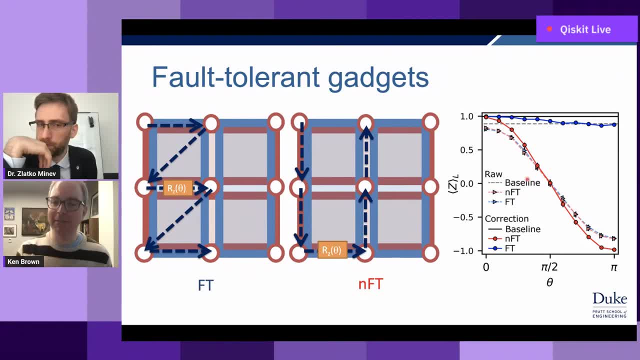 And if you don't do correction, then you get the same thing. So if you don't do correction, then you get the same thing. So the parity check giving you the wrong answer or flipping from plus to minus- follows the same pattern, because these circuits are equivalent, basically. 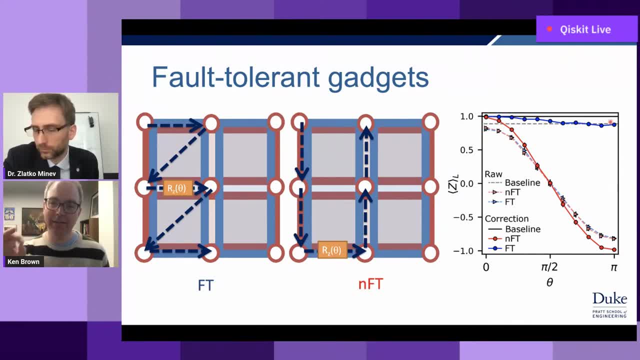 But when you do correction because of the fault tolerance, the fault tolerant method remains, gives you the correct, right, correct result, even if this goes all the way to z, because it it can protect us against that, Whereas the not fault tolerant one- this ends up becoming a logical z error. 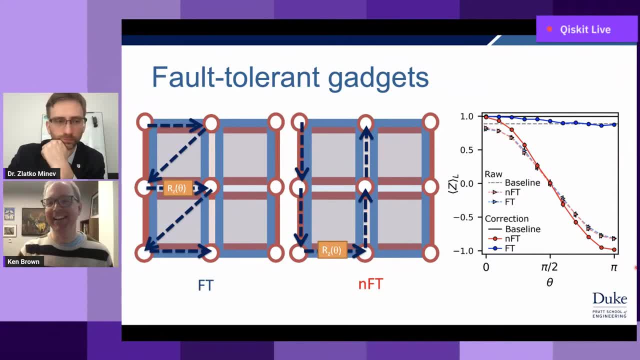 It collapses and you get- or, sorry, becomes a logical x error, and you get the opposite measurement when you measure the expected value of z. So it's pretty cool because I think it it shows, yeah, fault tolerant design works. but if that's not your error, maybe it doesn't matter. So there, 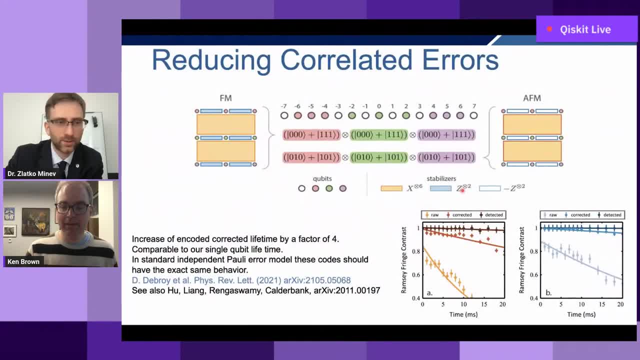 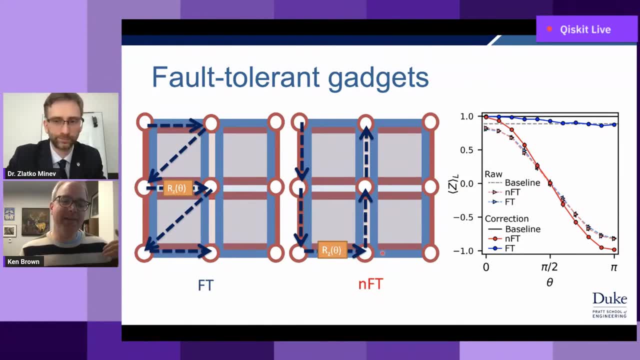 can be some shortcuts because of that. What's the dominant error to consider here? Our dominant error is still the two cubic gate error. right, and that two cubic gate error, because it- um, yeah, basically because it's an xx type error, and then that xx type error. 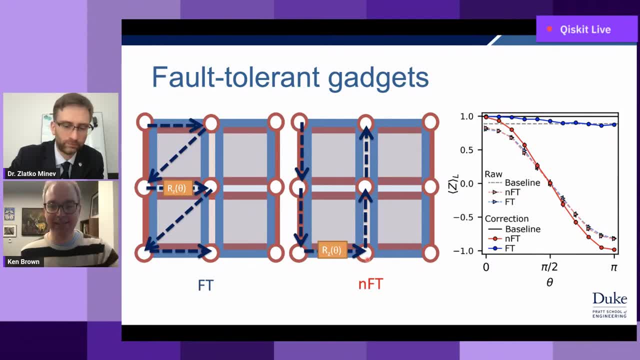 commutes with all the other two qubit xx gates. it doesn't lead to any kind of hook errors. It will it? yeah, it can basically, you know, change your, your measurement outcome. so there'll be some loss in the measurement outcome, but it doesn't propagate in a terrible way. 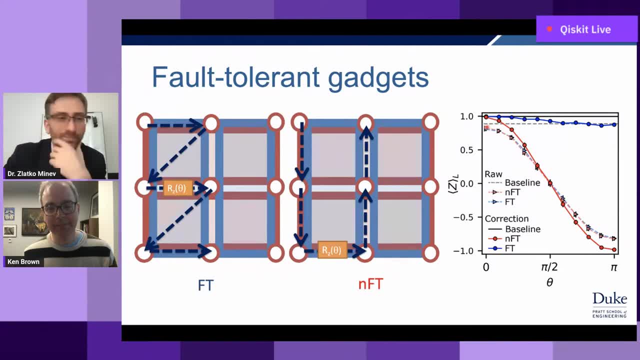 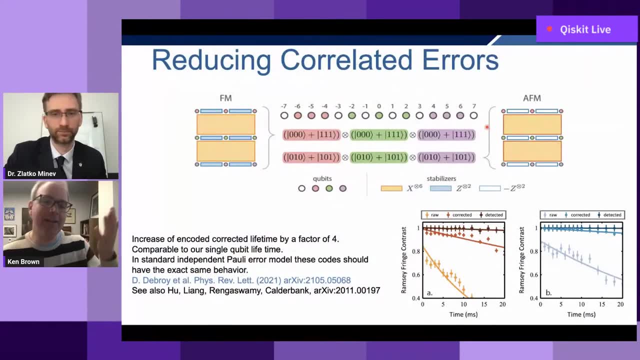 Okay, okay, good, And so then the next thing is-: okay, we do have a little bit of t2 error, which lasts, you know, usually, usually like our getting to like half a second is no big deal. The world limit for for a terbion t2 error, I think, is. 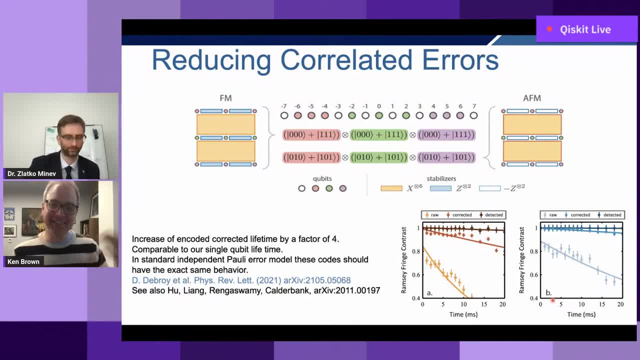 an hour now. Yeah, we usually go to like a couple ofoga hours seconds and call it good. um. so then, when you look at the, the, the states, and not at the stabilizers, you see that we've created three maximally sensitive to magnetic field states. 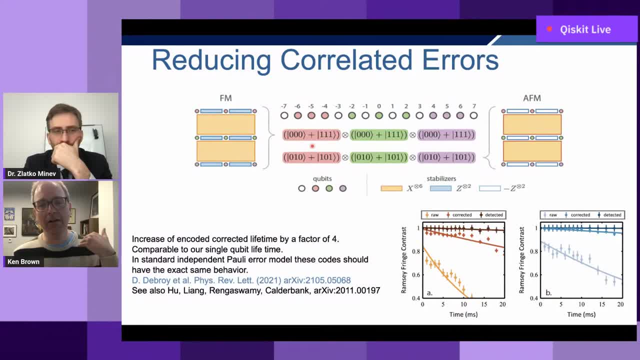 which are basically little ferromagnets, and so our logical um lifetime of just like preparing and waiting. we get a much faster t2, which, with correction, of course, gets better, but it's still. it's still fast. when you write it as states and not as stabilizers, um, you realize that. moving to, 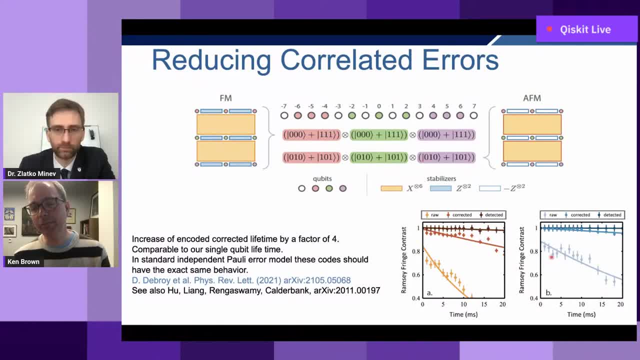 this anti-ferromagnetic type of state greatly improves, um the decay time, and then we actually get a logical coherence over these nine qubits, which is a similar time scale to our physical coherence. um, and then, from an error correction standpoint, what we've done is we've basically shifted. 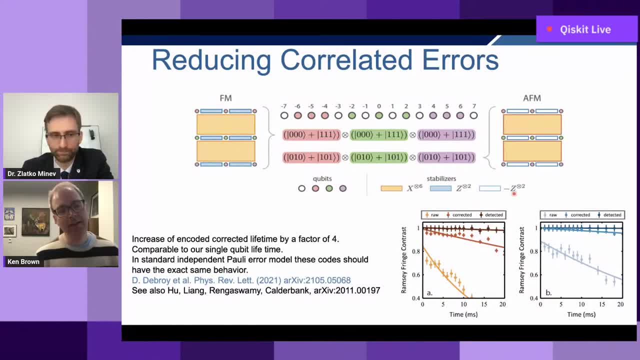 our stabilizers from z type to negative z. now what's really what i want to emphasize here is that if you only have stochastic poly errors- which is the way normally people talk about error correction theory- then this change will not do anything. it's only because the error is actually 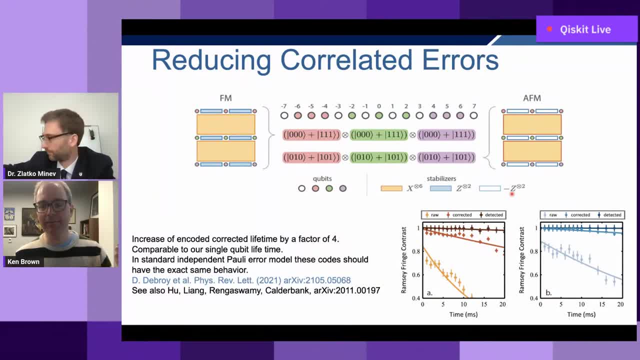 coherent that it leads to this um, leads to this game, and so so we worked on that, and there's also some nice work from my colleague, robert calderbank, where they basically showed, um, if you're guaranteed kind of global magnetic field noise, you can always build these weight to kind of checks, to totally remove uh following. 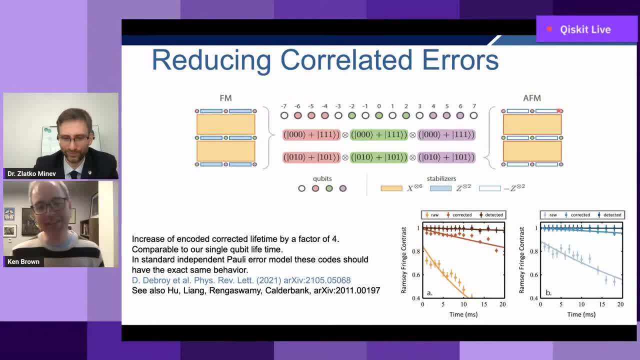 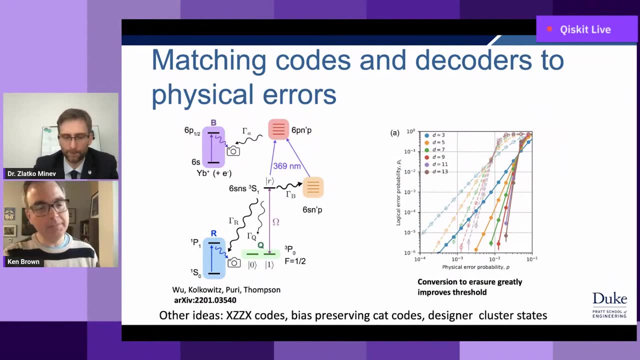 following: um, it's related to ideas from old ideas and deconference, free subspaces, uh, but it comes from a coding theory perspective which is a little bit different, uh. so, following up on that, like one of my favorite papers recently was this nice paper from princeton and yale on looking at neutral atoms and thinking about how actually there's. 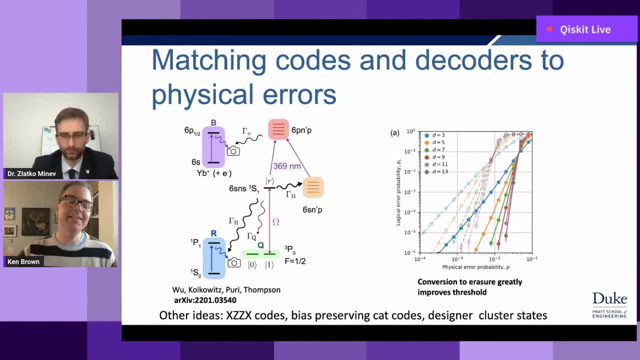 a way where we can turn the errors not into erasure errors, not into poly errors, but into an erasure error which removes your qubit, which sounds bad but you actually know where it happened and, as you can see here, by shifting to this erasure type error, these plots of 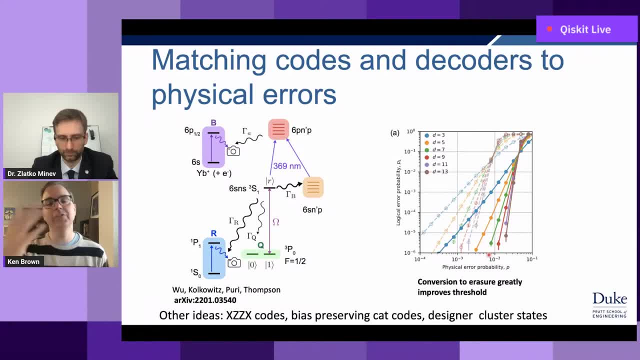 kind of thresholds of a surface code using neutral atoms, the threshold actually increases. and that goes back to that question about: is there a threshold? the answer is no, because it really depends on the details of the error model, and so by switching to an erasure error model they get a much higher threshold. 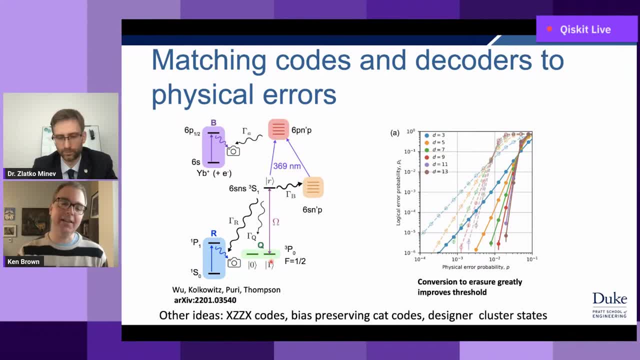 and i think i just want to point out there are other ideas that are very closely related, like i mentioned already, these xyzx codes more generally, making clifford transformations to try to map your errors onto a bias that you control. that works really nicely with some of these ideas of bias. 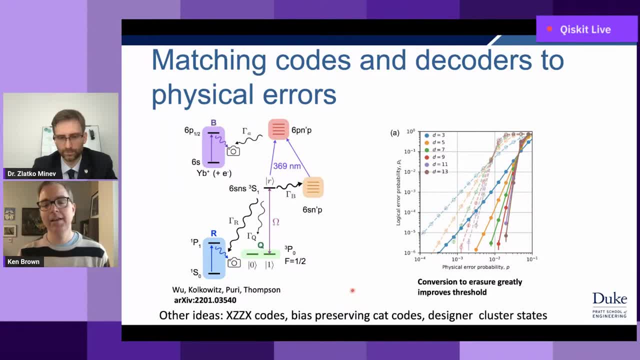 preserving catcodes, which allow you to do gates that maintain the bias. It also connects to ideas on designer cluster states, where you build clusters of different types. So there's a huge amount of interesting work here. I just want to say, with respect to the erasure, we joke that we 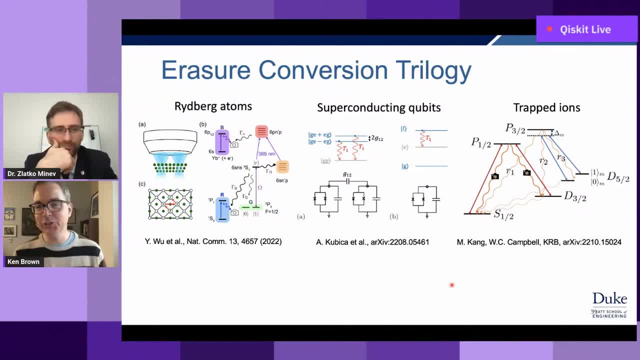 tried to do at least the third movie in the erasure conversion trilogy, which is so compelling. it was not surprising to see ideas on again. you can put together doses and junctions and capacitors and superneutrality any way you want. Here's a way where you basically transform any. 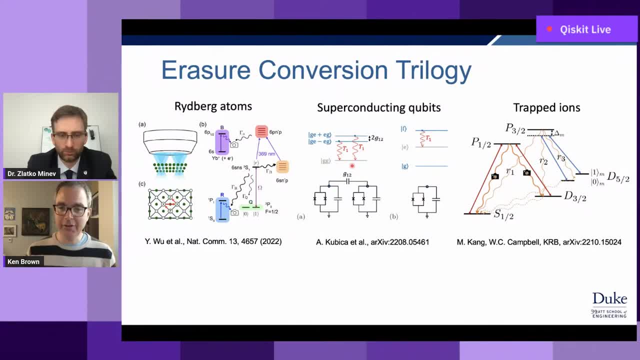 T1 error into an erasure error from your qubit state to something which is hopefully detectable. And then, with my student Mingyu, and then Wes Campbell, his professor at UCLA, we were able to show how to do erasure type of conversion using these metastable states. metastable states and then we were able to do erasure type of conversion using these metastable states, metastable states- and then we were able to show how to do erasure type of conversion. stable qubits and not just the ground state qubits and traptines. 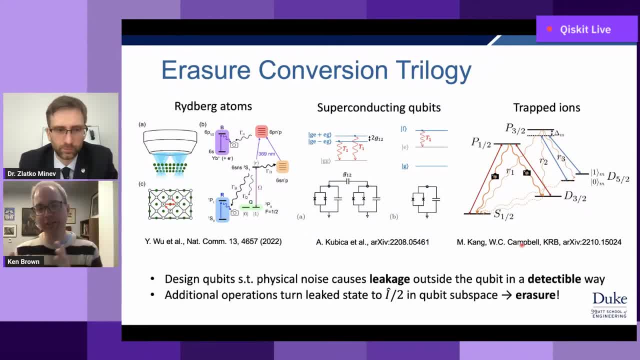 So yeah. so it's amazing thing because basically just by changing our protocol and how we, where we define our qubit space, we can actually transform the type of error and it turns out that erasure errors are actually very good and forgiving. 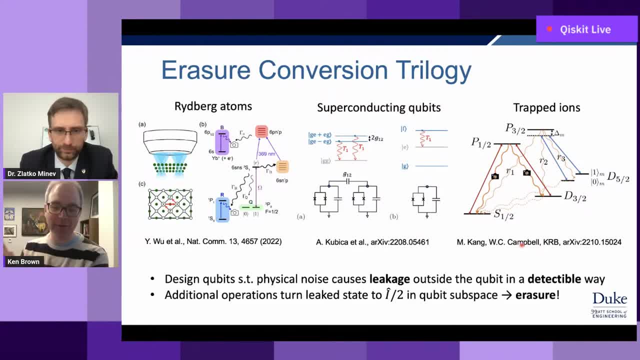 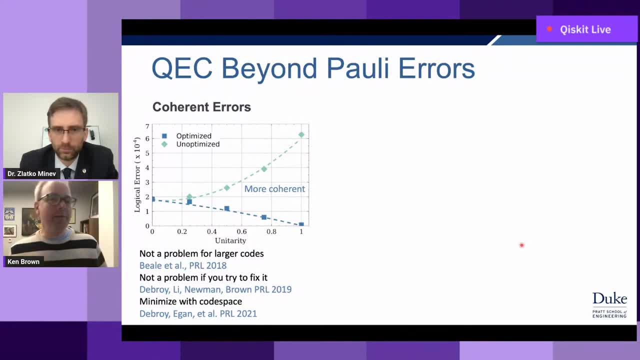 Um, like, if you could pick an error, it's, it's, it's a great kind of error to have. So then, um, yeah, summarize a little bit. So quantum error correction beyond poly errors is something my groups worked on for a long time. 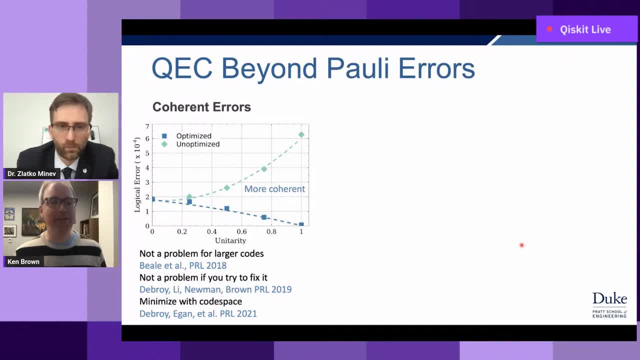 These are some some of our works on thinking about coherent errors. Uh, we showed with uh Joel Wallman, um, and very lifelong coworkers. Uh, yeah, Stephanie builds the first author there. uh, that basically for larger codes, it shouldn't matter. 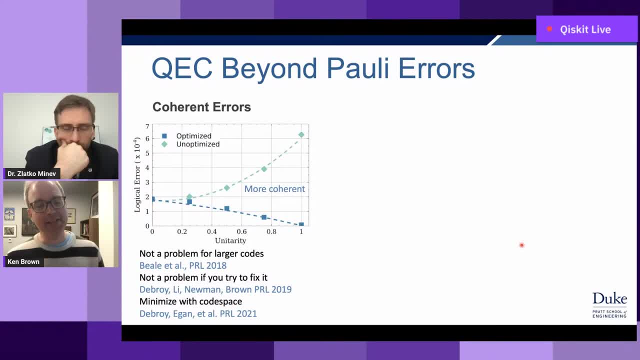 Um, better than that. if you do stabilize the sizing, you can fix it And then we can actually minimize the code space based on the coherence we have. A real problem is the Hilbert space is large And if you fall out of the qubit space and you don't know it, that's called leakage. 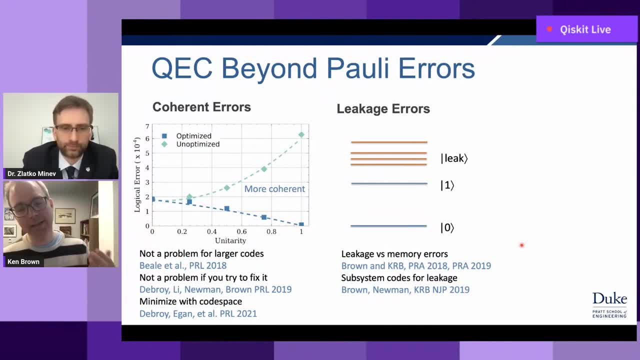 And so then, um, I worked with my student, Natalie Brown, and then Mike Newman, where we tried to um, building off ideas from- uh yeah, from IBM and Google on how to handle leakage and superconductors just apply them more generally to these codes. 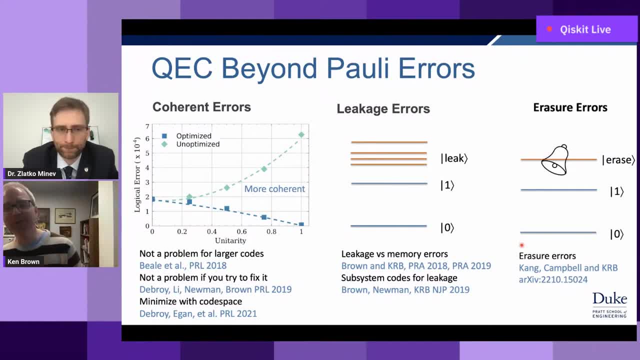 Um, and then, as I just mentioned, if you have a leakage which you can tell, then it becomes an error: Um, and and, and, and, then, and then. once you think about that, you can think well. 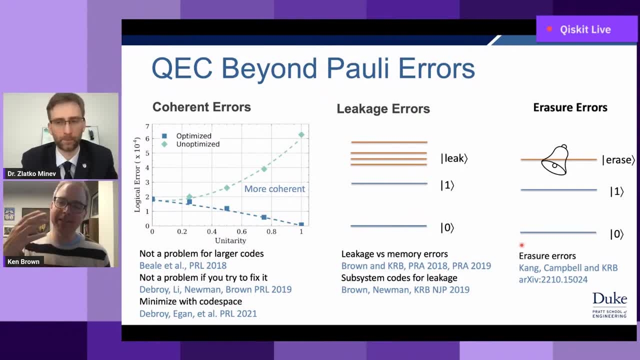 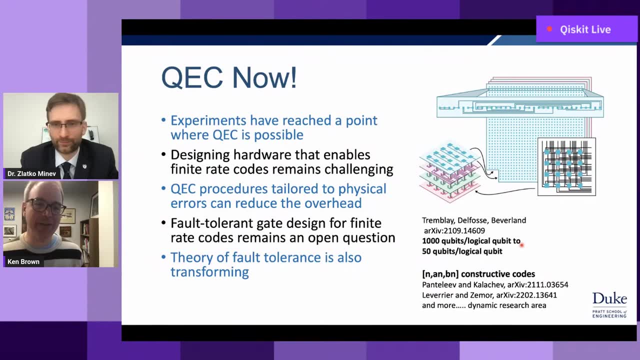 actually maybe I don't want to design systems that have lowest error. I want to design system which has the best error for future error correction. So I'm super excited about quantum error correction right now. I think there's a huge amount of um advances on the hardware side. 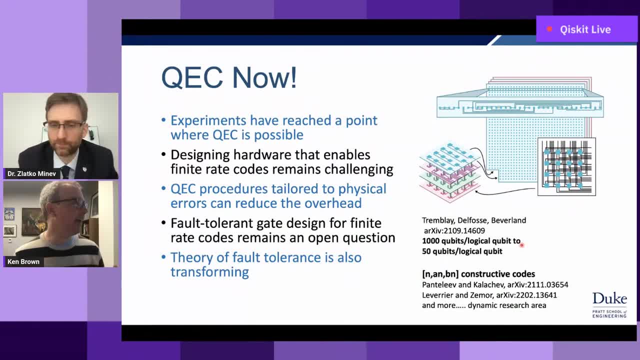 Um, there's also this, this advance in like actually thinking about the real physical errors and how that connects to your decoder. Um, I Deleted all my slides about finite rate codes, which I think has also just been um in the. 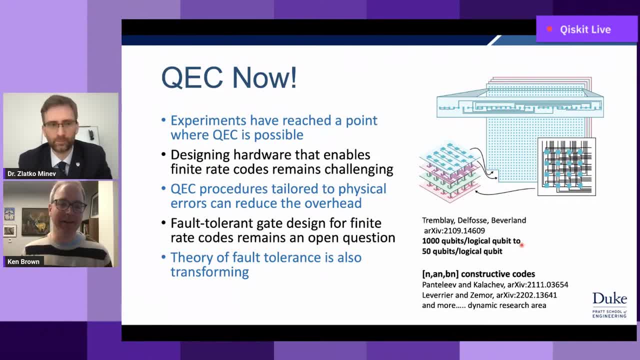 last three years, just like an explosion of ways to try to to make error correction more compact. Um, and I I think This is sort of forcing the theory of fault tolerance to transform And um, there's a lot of great work to do. 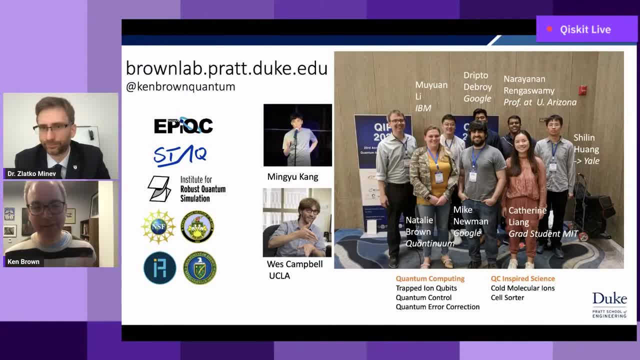 So when I briefly- uh, you know, think, of course, uh, funding the national science foundation, the army, IARPA and department of energy- um, yeah, I didn't really talk about it, but Mingyu and Wes. 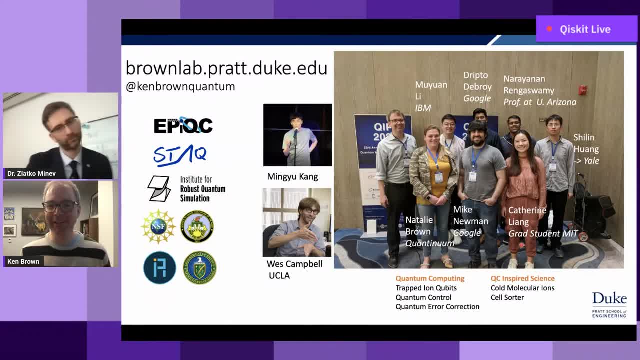 Presenting the collaborators on this erasure paper. This is a picture from QYP 2020.. With uh yeah. So, like Natalie and Moon and drip, Joe and Mike, I talked about their work with respect to uh Uh, as they can'. 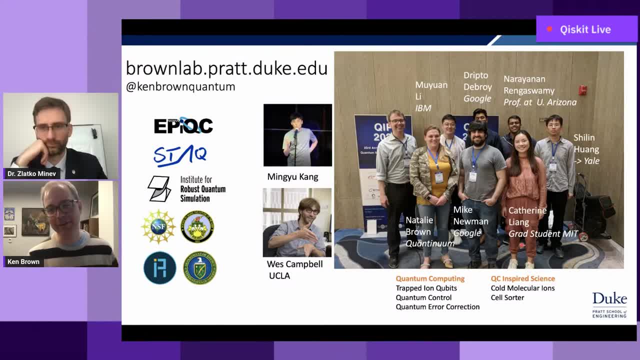 And a little bit of a leakage, and now they've all gone on. Um, I'm actually really excited, like you know. suff, no efforts, the, Uh, the, the inn, the heavy hex code IBM paper. Just Mike on this. 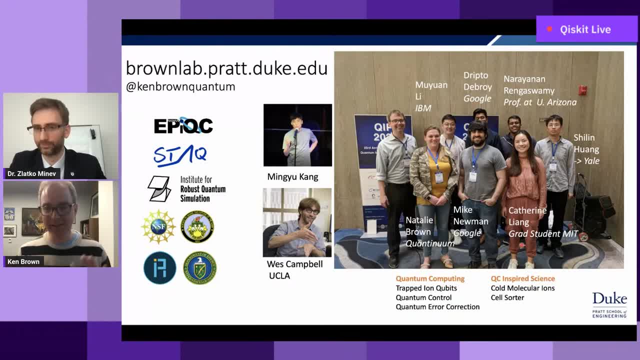 Distance Five paper logical C-naught between steam codes, I don't know. It makes me like a very proud advisor. I guess Narayanan worked with Robert Calderbank on this, getting rid of all coherent errors I mentioned. he's now a professor. 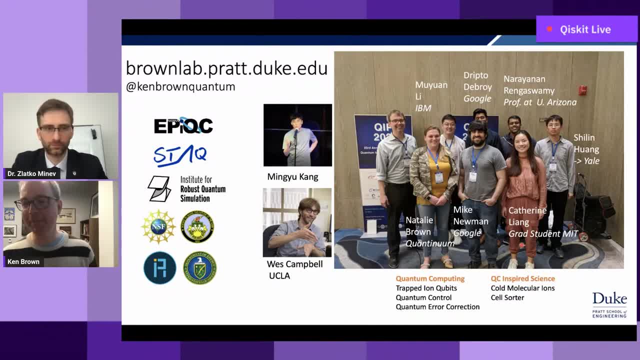 at the University of Arizona. If you're looking for a PhD advisor, you should think about him, And you can also think about me, but also think about him. Catherine is now a grad student at MIT. Shilan will defend his thesis next week. 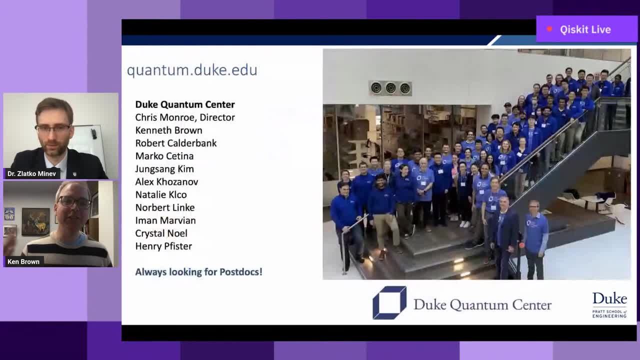 and then we'll go off to be a postdoc at Yale. And then I just also wanna say that the group has grown quite a bit in terms of the quantum that's going on at Duke. We now have this Duke Quantum Center, which Crispin knows the director. 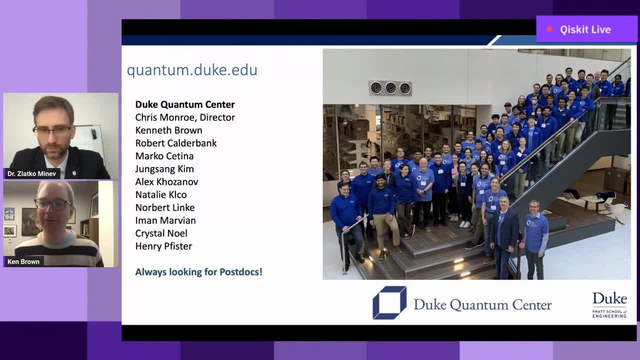 We have all these nice faculty. We're looking for postdocs in all types of work, from theory to experiment to engineering, And with that, thank you for your time and I'm happy to answer any questions. Thank you very much, Ken. 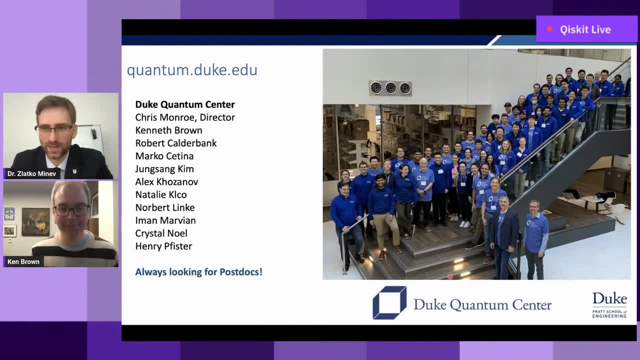 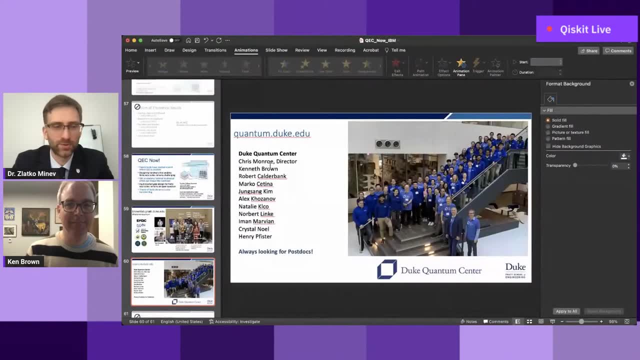 for the really nice work and congratulations on the great results. There were a few questions that I waited on until the end, so folks feel free to post those and repost questions and add questions as we get to the end here. Very nice picture with color-coordinated shirts. 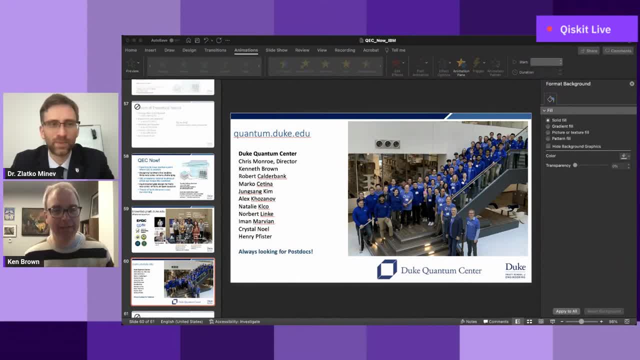 Maybe we'll start with a question from the middle of your talk, from Juan Wei. How were the two-qubit Mohler-Sorensen-Gates benchmark? Was it with randomized benchmarking or decay or parity oscillations? If you could tell us more about that. 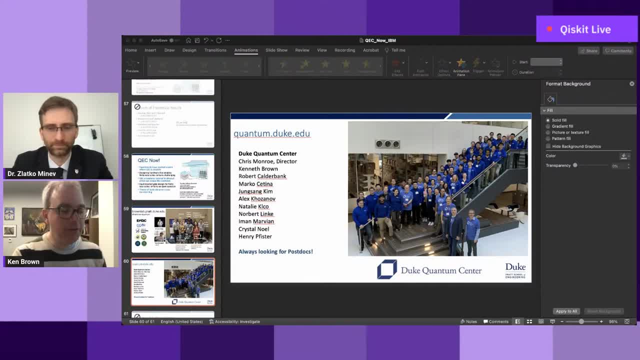 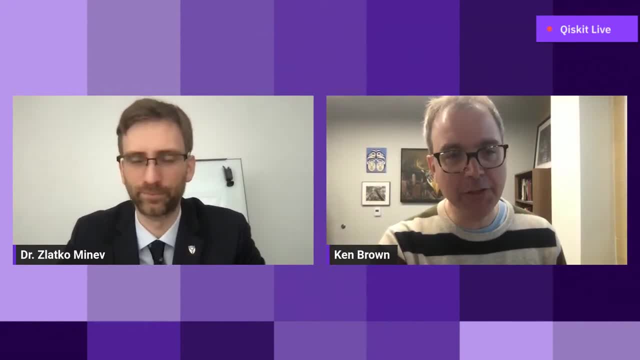 Yeah, so we normally we do kind of two things. So the number we usually report is a parity oscillation report. So that checks the parity oscillation checks that the entanglement fidelity is maximal And the thing which it misses. 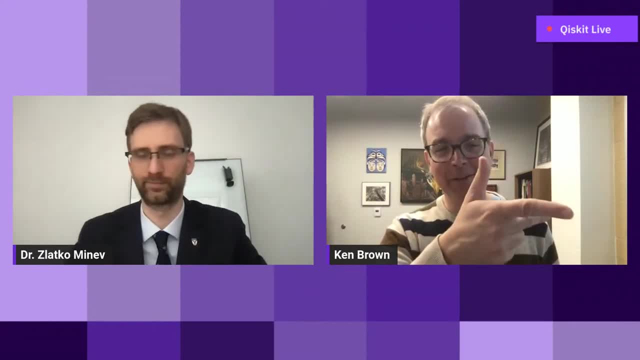 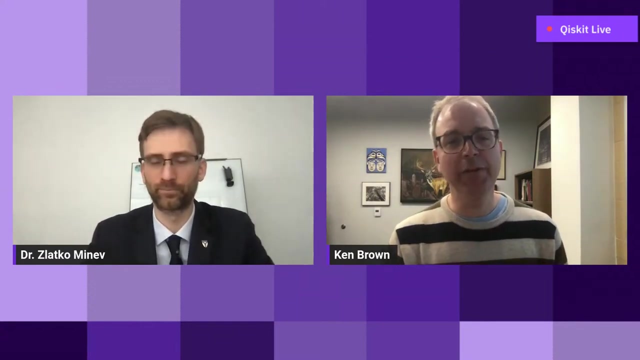 is it misses. it's a weird thing to talk about, but you have like X, Y and Z of your single-qubit gate and you have X, Y and Z of your two-qubit gate. you're lucky those things agree and this parity oscillation misses that. okay, so we do a different. 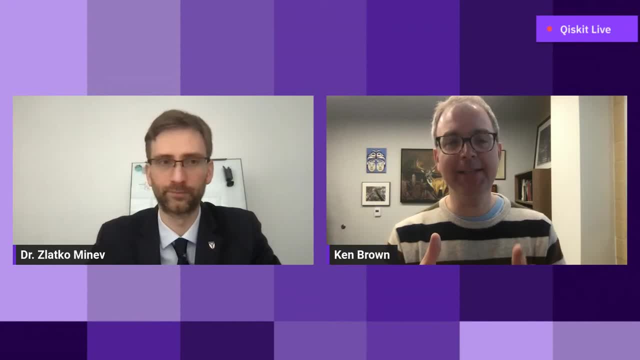 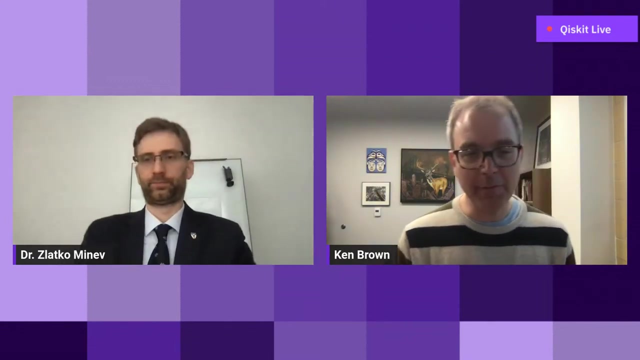 type of check which allows us to see that these things are aligned with each other? um, like, one easy way to do it is you basically feed it what you think should be as eigenstates and show that nothing happens. um, yeah, we do not usually do to keep it randomized benchmarking, because, um, 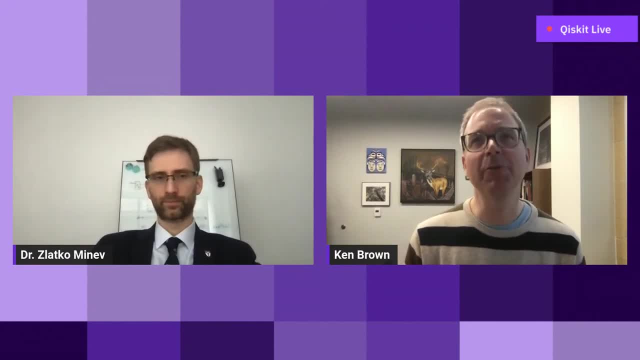 we have done to keep it randomized benchmarking. the numbers are reported from parity- excellent things to keep. a randomized benchmarking takes a long time and it- um, yeah, i just haven't. i. i would say okay, so sorry, now i'm gonna. my big picture problem is this: 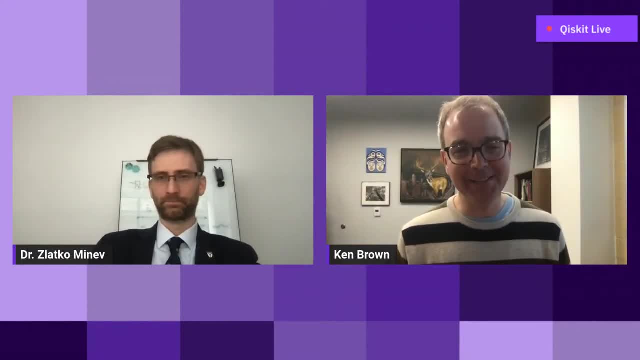 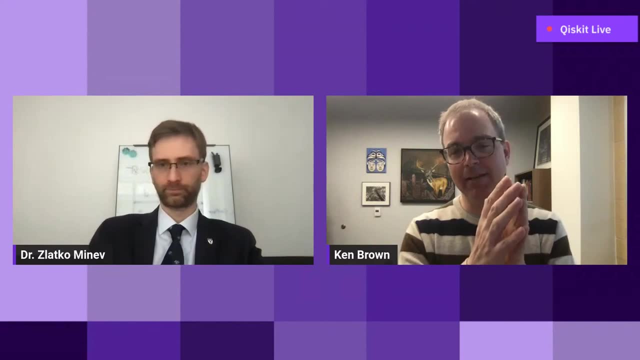 i think characterization tools should help you fix your gates. um, and oftentimes when you have a a very complicated characterization tool which ends up taking a pile of data over long periods of time, which also kind of mixes systematic data, that that results you get doesn't tell. 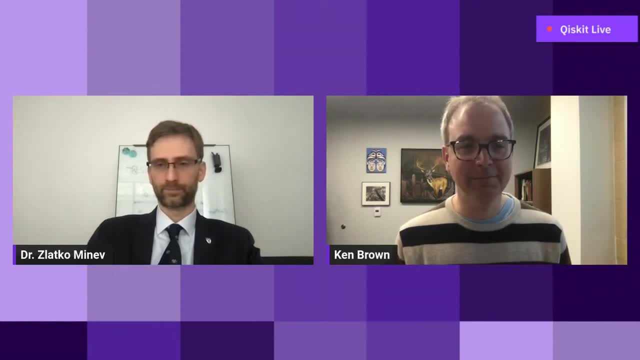 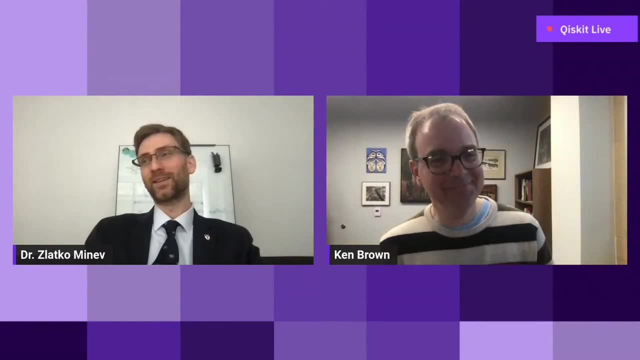 you how to fix it, say, um great, thank you. i uh, yeah, i yeah. i think our audience has a lot of diverse backgrounds. some of them are definitely hardcore rb people and some are you know much more about. let's find out actually what each poly term and 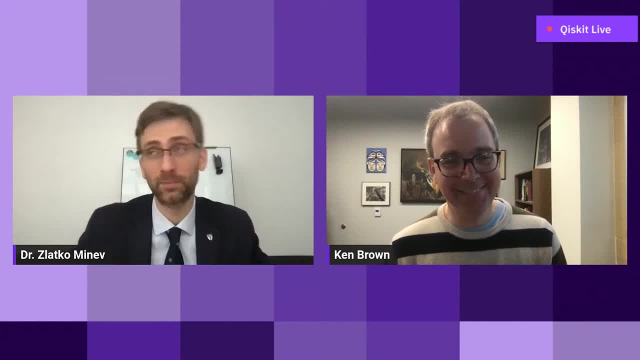 the error is- and we've had a number of talks here on uh by myself and others on, you know, really learning the noise in the quantum device at scale, including crosstalk, and really understanding as many of the possible generators or the actual terms in the noise as possible. so i, i totally 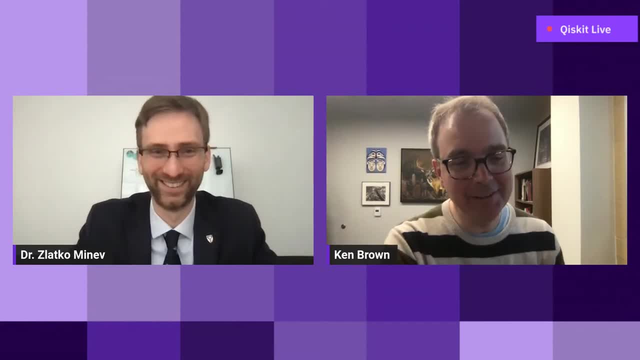 agree with you. yeah, i just want to say my favorite. i don't um, i yeah, i don't have this, have this light in my talk, but one of my favorite examples is we were using um gate set tomography from sandia national labs using their version of it um and. 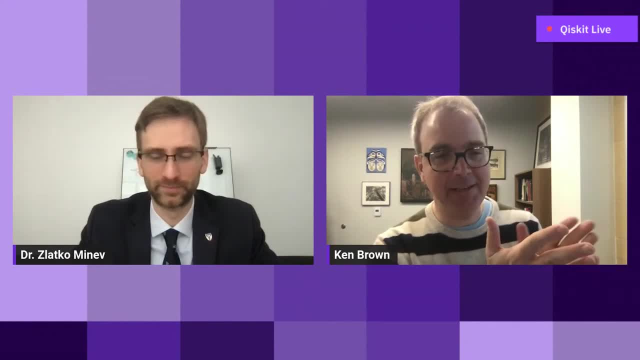 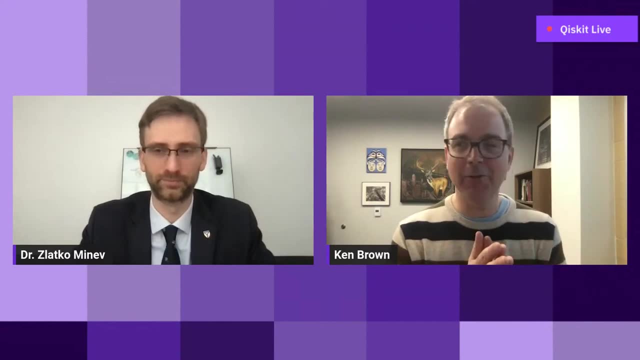 what's funny is we use this kind of composite pulse technique to take three single qubit gates to make one really good single qubit gate called sk1, and we know it works and so we. we've always compared like um. so if you do randomized benchmarking with single qubit, 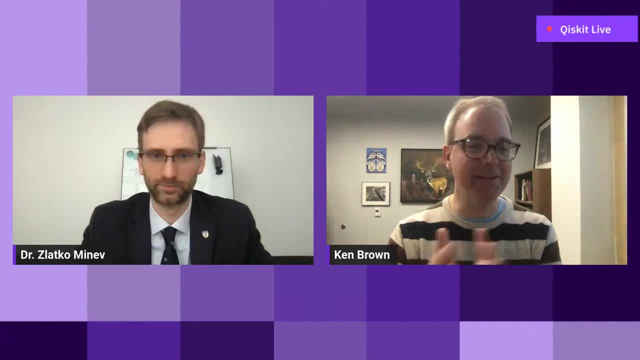 gates versus these composite pulse gates. the composite policy, randomized benchmarking, is always better. you do gate set tomography. it's better. and then we asked: well, can we close the loop and take our gate set tomography results for single qubit gates and predict if the composite pulse will help us? 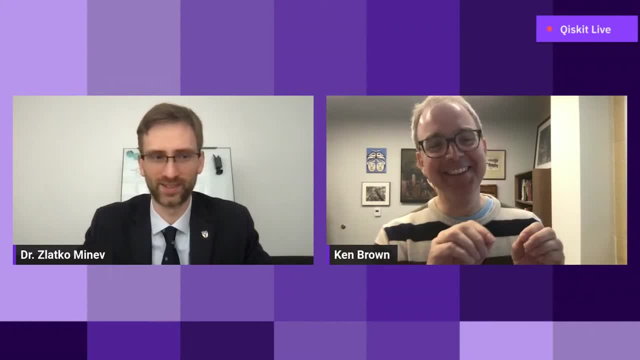 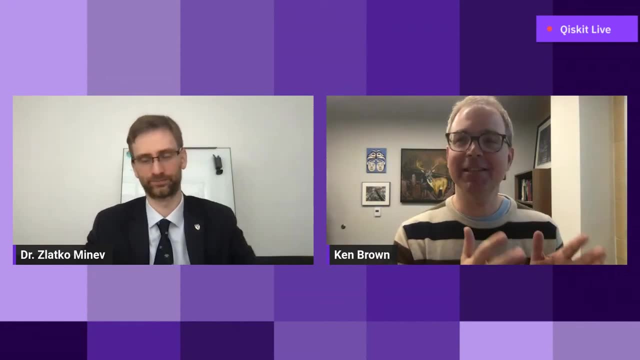 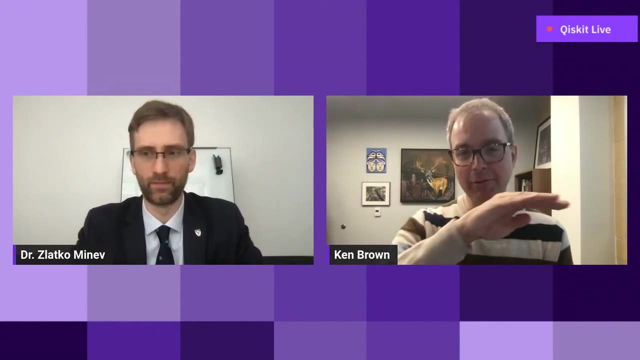 and its prediction is no. its prediction is that the, the, the, the. yeah, this prediction is no. it'll actually hurt you and the reason is because gate set tomography assumes errors are always constant. but composite pulse actually is great if you have like a slowly varying error. 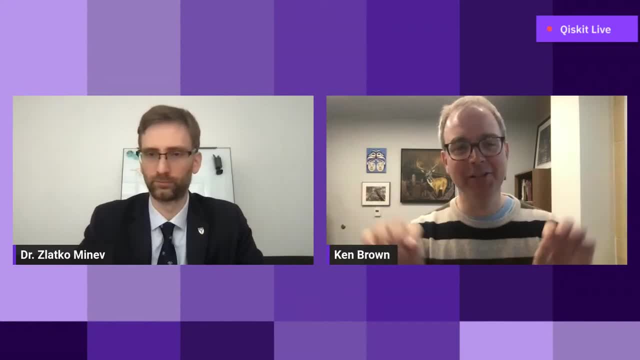 so when you take all that gate set data, like it just scrambles to an average. but if you, if you, yeah, if you- um, i don't know you- i guess you have this analytical hypothesis that it should work and then you can see it does, but it's, it's. i, yeah, i'm always um. 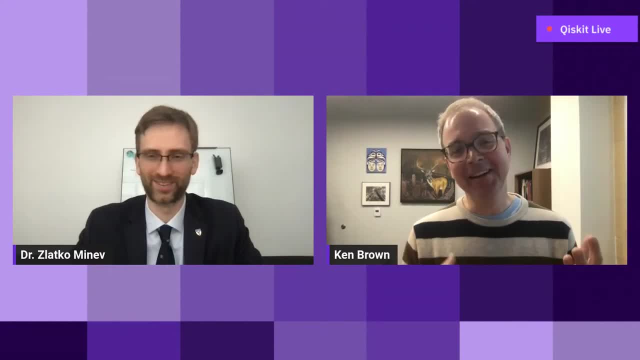 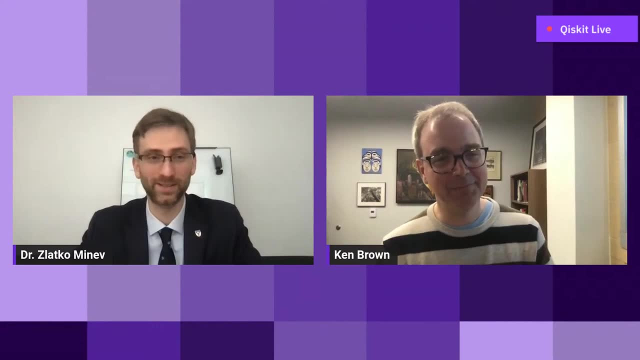 well, i mean, as you know, it's like i'm very interested in this problem of like: how do we characterize in a way which makes things better, exactly, exactly. and i'm excited to see i think there's more and more work in in coming out in the community. that helps with that, but that's not the topic of today. 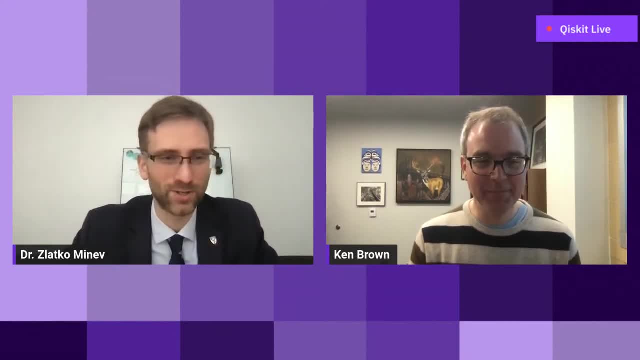 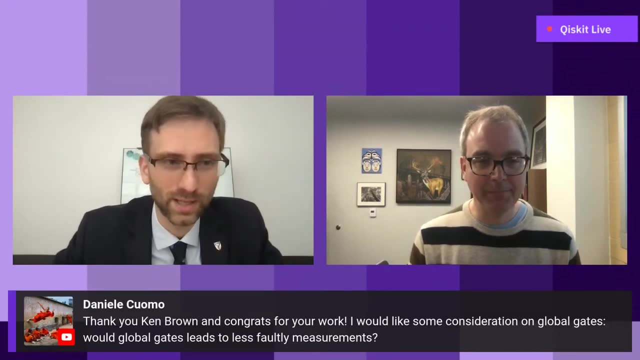 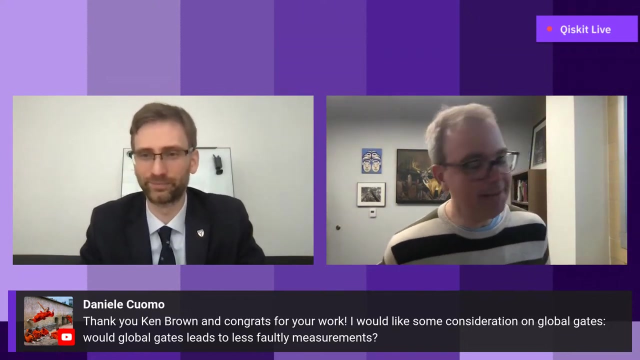 question from danielle cuomo. thank you, ken, and congratulations for your work. i would like some considerations on global gates. would global gates leads lead to less faulty measurements? yeah, so, uh. so in a, in a trapped ion quantum computing um, you can just basically generate um, an easing type interaction between any pair um, just as 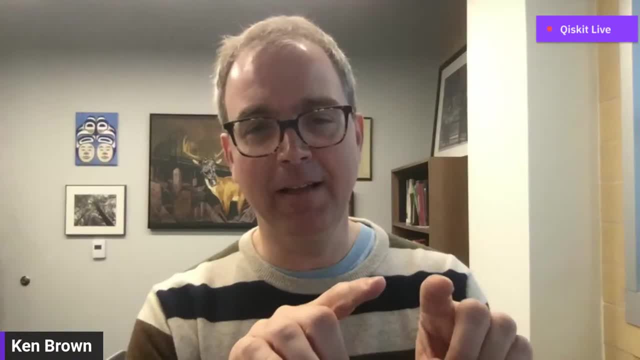 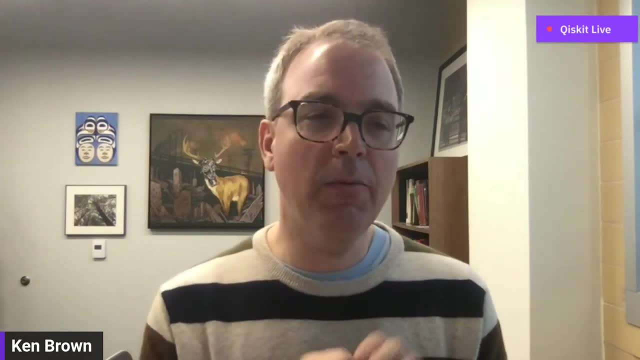 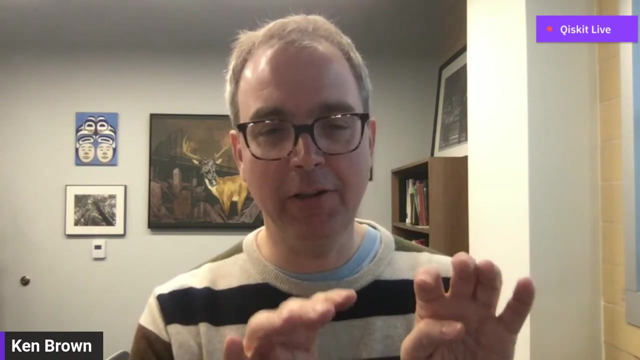 for other people who maybe don't know about global, ms gates: uh, you can actually make an easing interaction between all the qubits at once. so what's interesting is, from a theory of fault tolerance method, this global interaction all at once, if i assume, poly type errors. 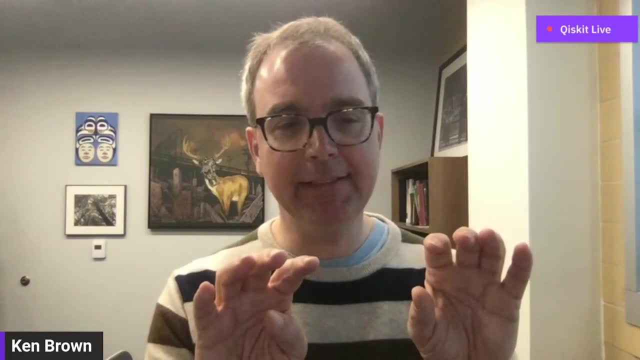 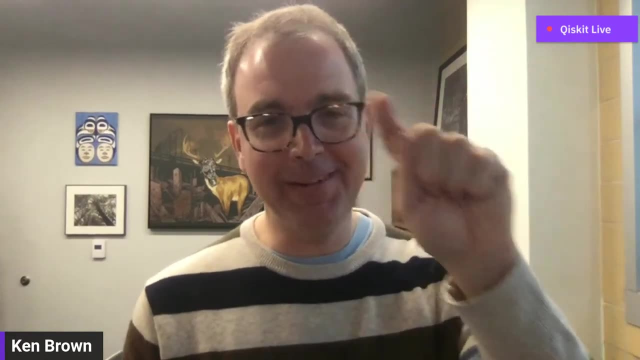 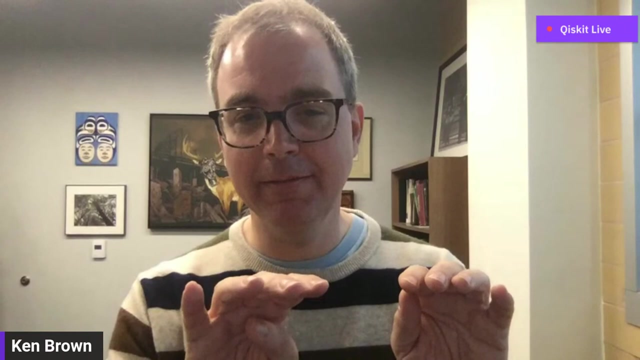 could be really bad. it basically would allow errors to propagate to all these pieces. but that piece of data i showed you, where our careful selection of c naught order didn't matter, says that in that experiment we could do the full global gate, and it would be. it would, um, it would probably be better because it would. 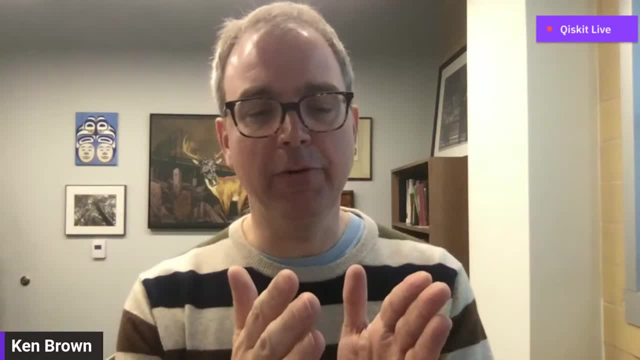 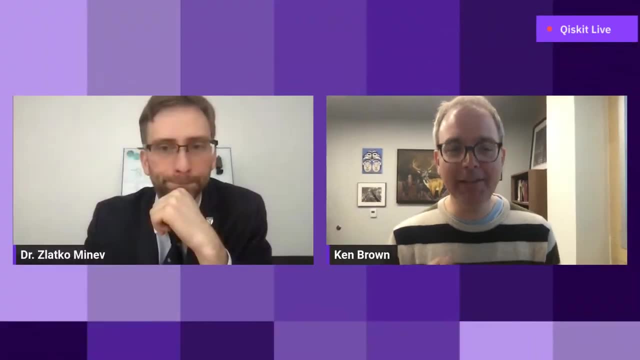 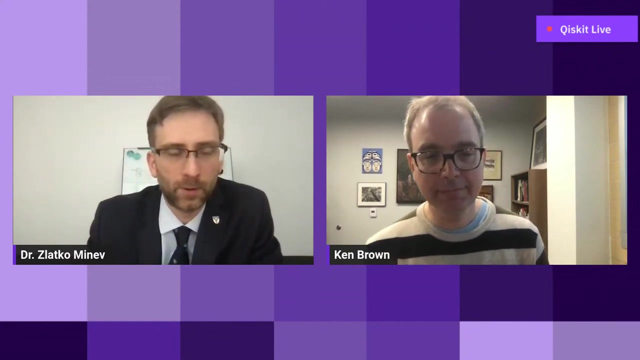 happen in less, less overall time and therefore, um, you know, some other side effects of heating etc. should be better, but isn't it? yeah, it's, that's a great question actually, and it really depends on the errors that actually happen. excellent, thank you. um quick question from boris bervanov. 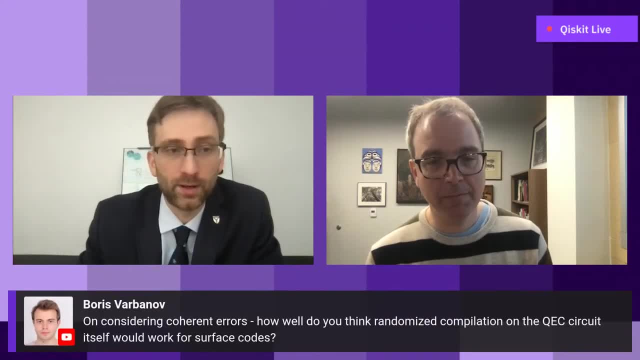 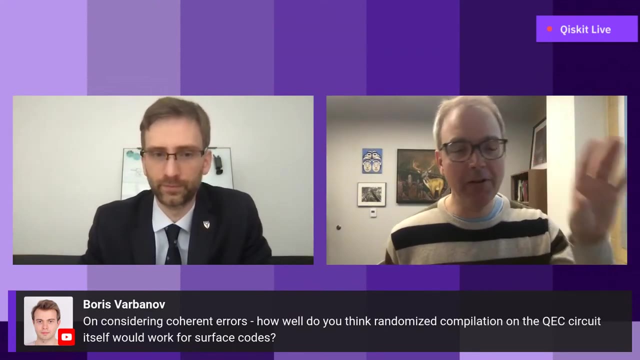 on considering coherent errors. how well do you think randomized compilation on the quantum error correction circuit itself would work for the surface code so effectively? twirling, yeah. so for the distance, um, for the, for the distance, the small code, we looked at distance 3. It seemed like it kind of the poly measurements, kind of do the randomized compiling for you a little bit. 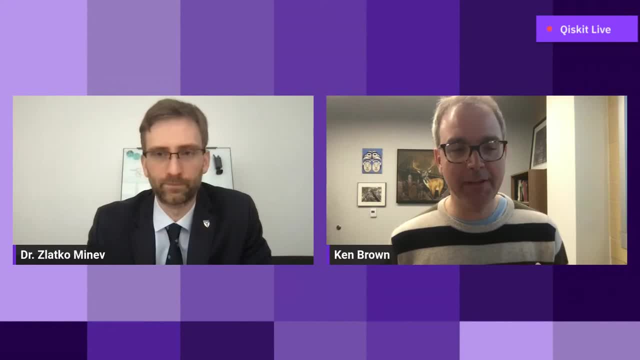 I do think randomized compiling often helps. like is a great- what do I want to say? kind of a hedge, So like if you don't know what your coherent errors are. randomized compiling is great because it just, you know, averages them to some point. 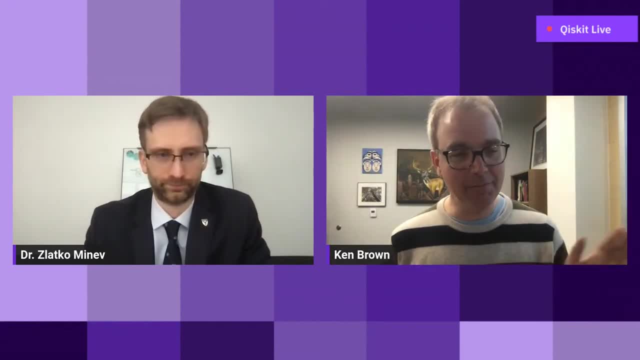 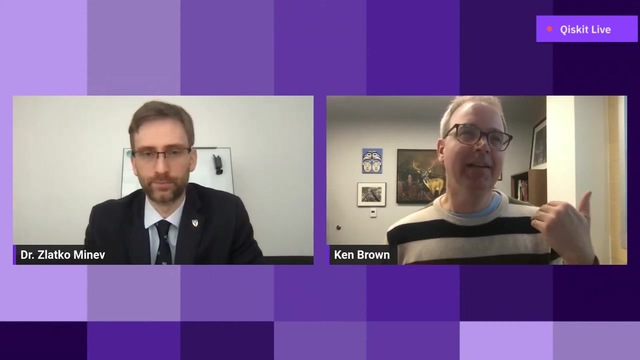 Again in work. if we look at the Bacon-Shore code example, where the coherent errors- having errors be more coherent- helps you. If we randomized compile the circuit we would lose that key. So if you have a lot of knowledge about you don't need to know the strength or magnitude of the coherent error. 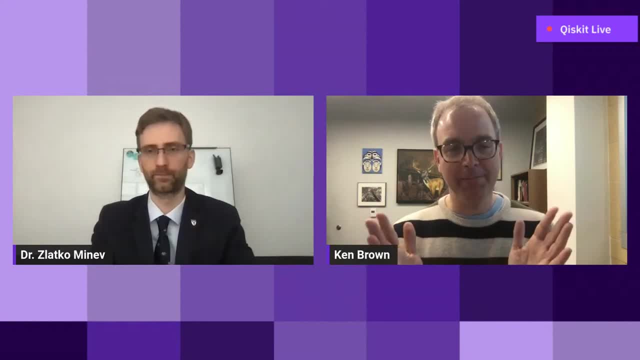 But if you have a lot of knowledge about its expected form, Then often you can do better than randomized compiling. And then I want to say that actually some nice work from my student who's about to go work at IBM, basically we can put them together. 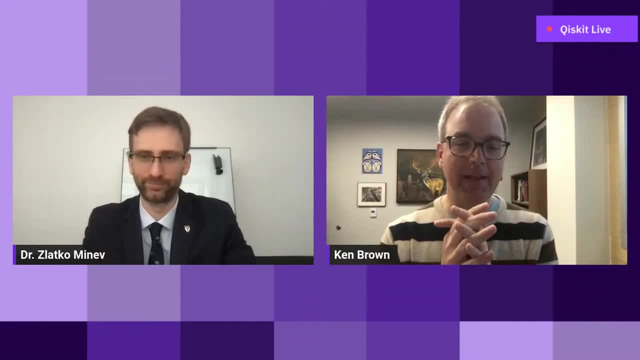 So we can take the part where we understand how the errors connect and do our special trick, and then we can take that block and do randomized compiling outside of it For that coherent error And then we can do a lot more coherent errors we haven't expected. 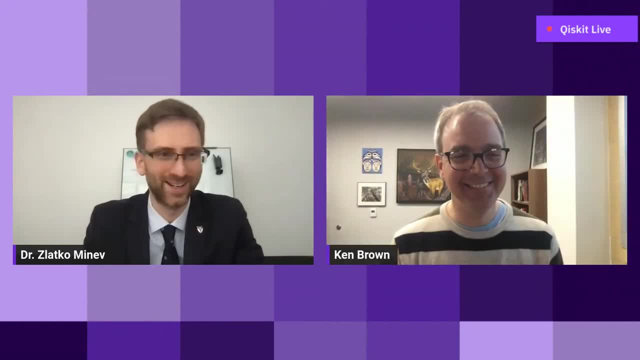 That's excellent, I can echo, for how great Swarnendik was. Now a follow up question, perhaps For well on the simulation side, for theory research, what factors does your group use for simulation of large systems of qubits? 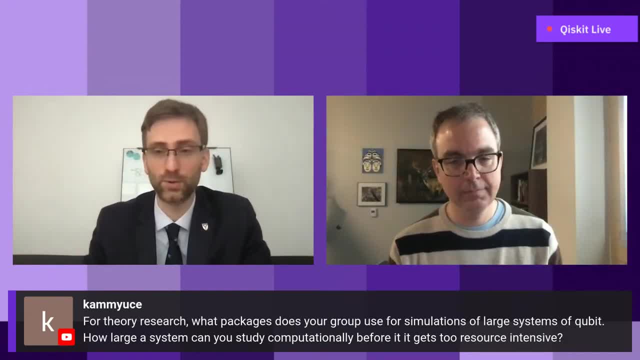 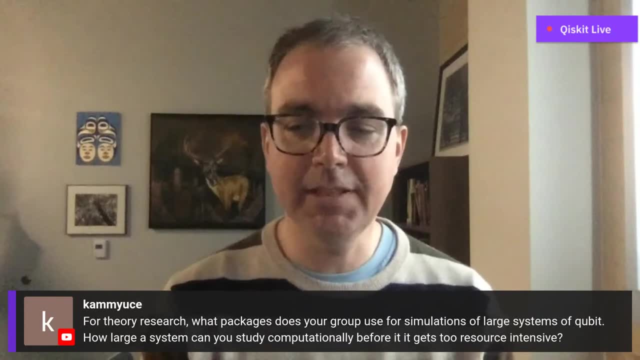 How large a system can you actually study computationally before it gets too resource intensive? Yeah, So that's a great question. So you know, for some of our largest systems we use things like, you know, stim or pie matching or whatever. 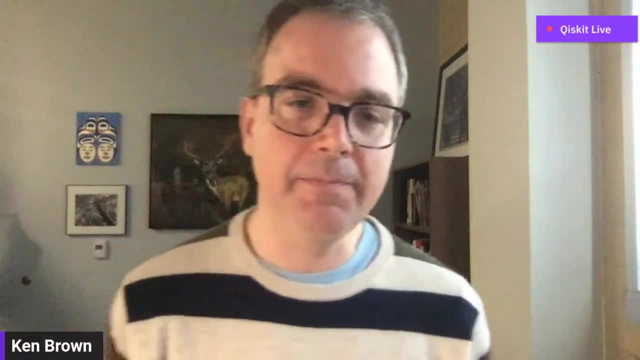 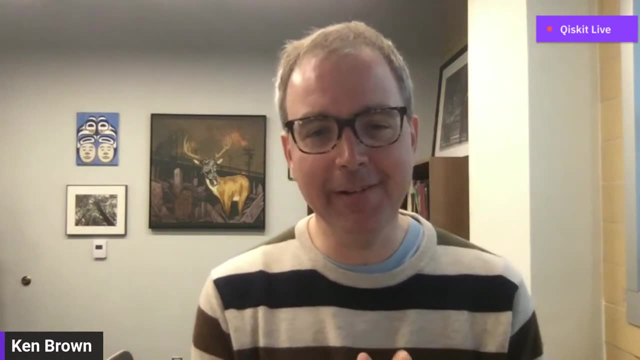 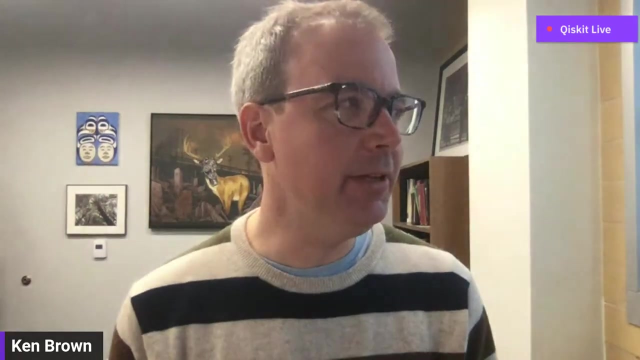 But when you use those systems you have really kind of like limited types of error models, right? So then, if I want to look at coherent error models, then we- yeah we use, you know, QSIM kind of packages where we just model the whole. 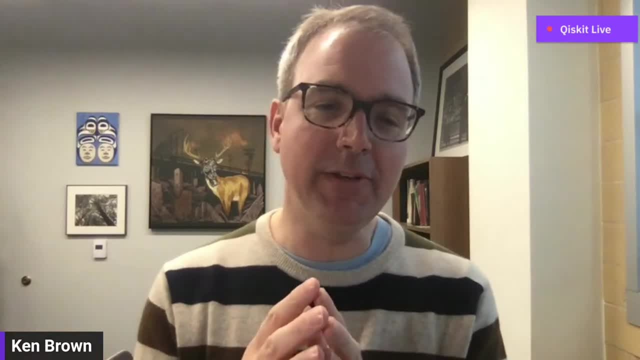 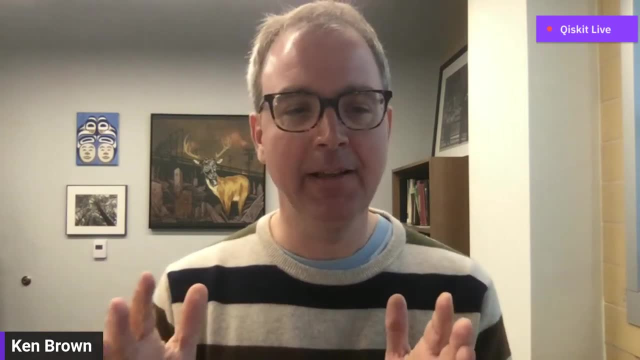 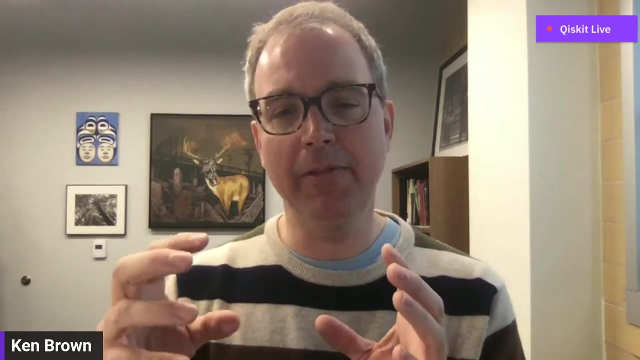 density matrix. And then for us, you know, once you get beyond, you know 10, 15 qubits, that starts to get really pricey. And so there was some really nice work by Thomas O'Brien where he basically thought about how- because you're always measuring these syndrome qubits- 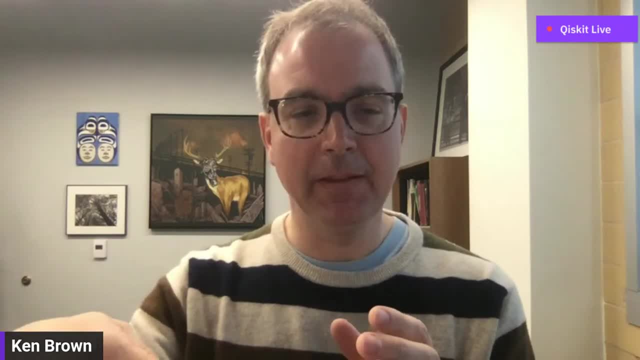 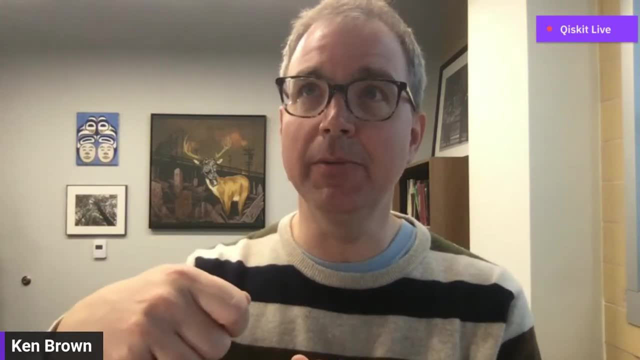 you don't really need them to be active all the time And so you can actually work with this smaller Hilbert space. but then you have to be careful about how you- basically how you account for time, But but yeah, that's, that's a real challenge, I think. 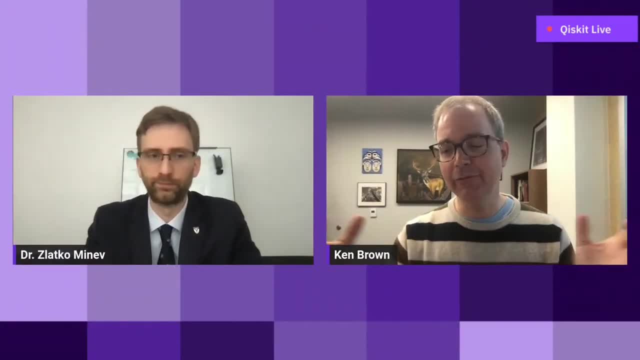 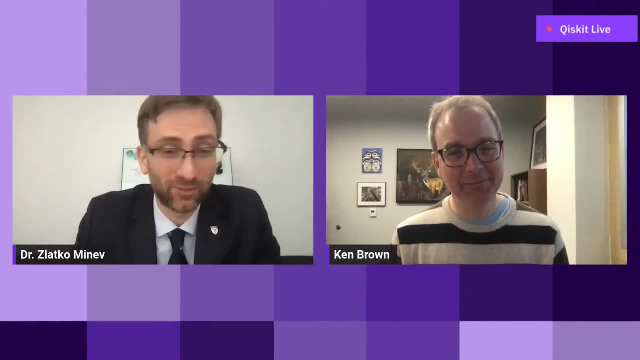 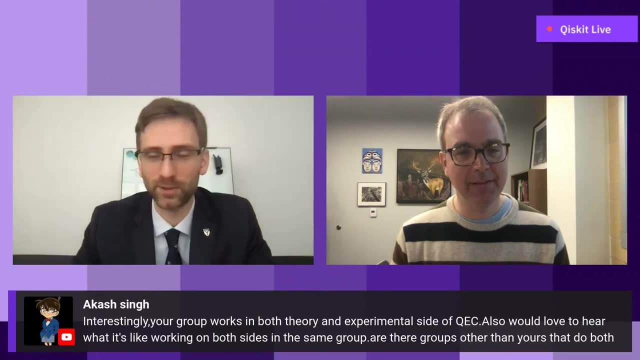 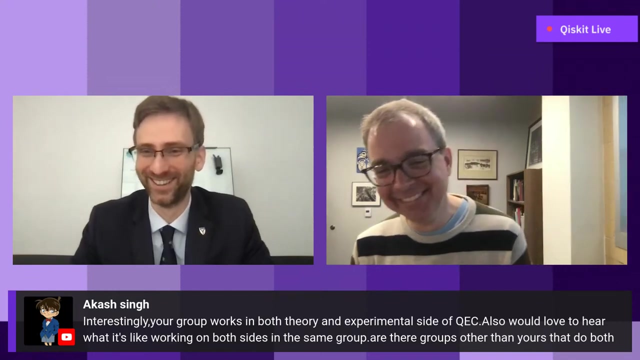 it's a common trend. And final question from Akash: Interestingly, your group works both in theory and experimental side of QEC. Would love to hear what life is like working on both sides in the same groups. So I think there's more of a career question. 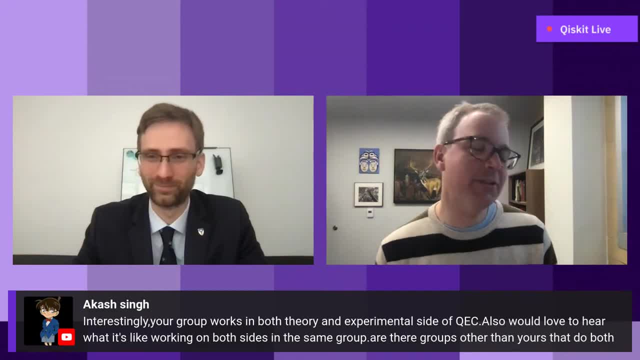 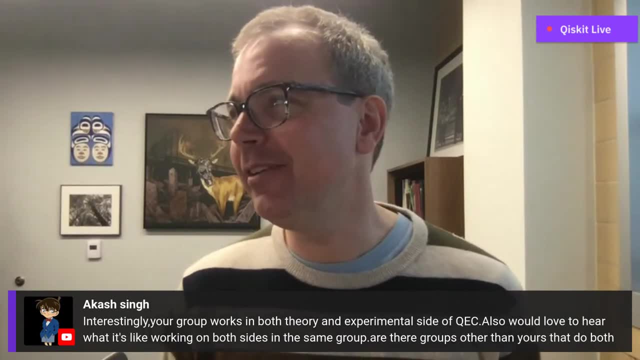 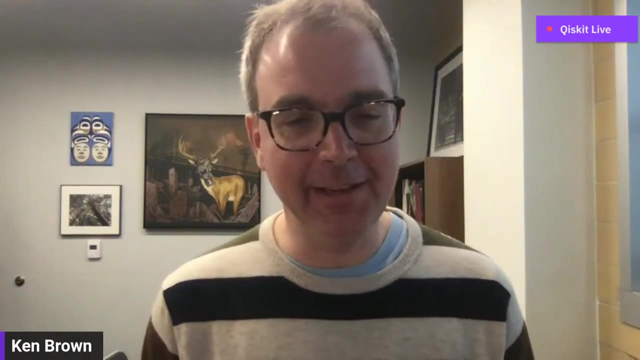 Yeah, Okay. So I mean: yeah, So my my B, I was just recruiting grad students yesterday. I do think like that is. one very special thing about our work here is that if you have a theory, if you're a theorist and you want to run the thing on an experiment, you 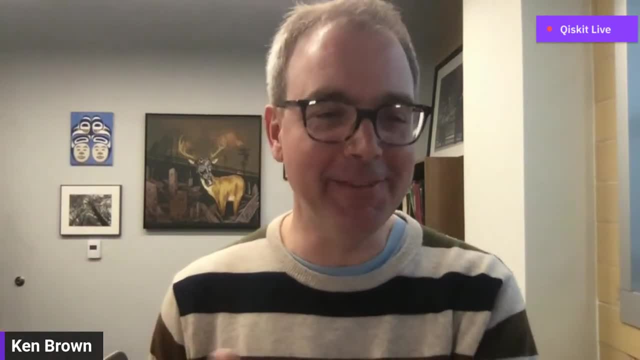 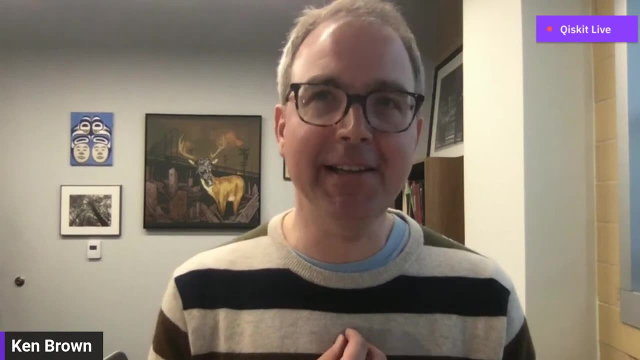 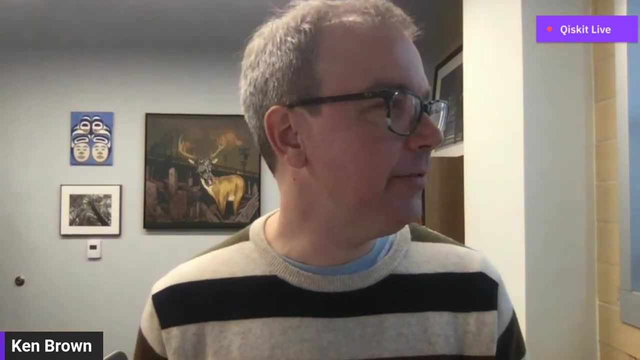 just walk over to the other side of the lab and like convince them to give it a try. I think I would say, you know, the way that I got to this position was as a PhD student. I just did theory And when I was finishing my PhD I felt 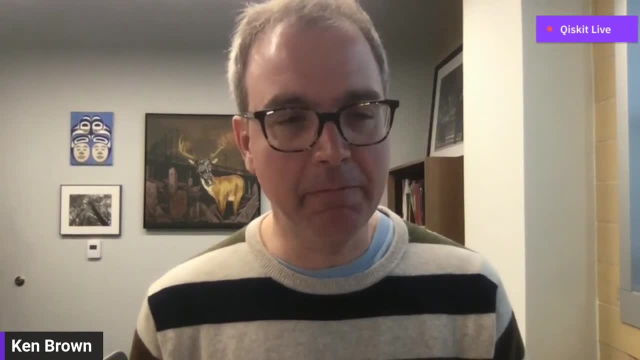 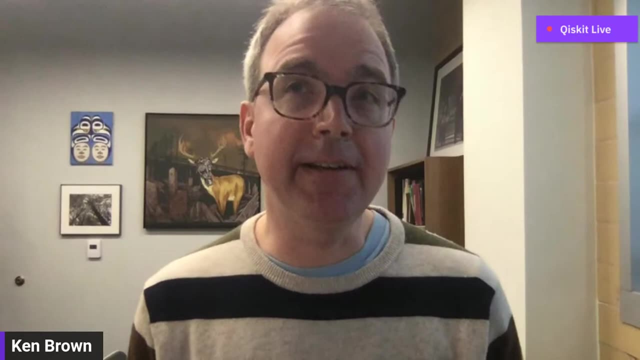 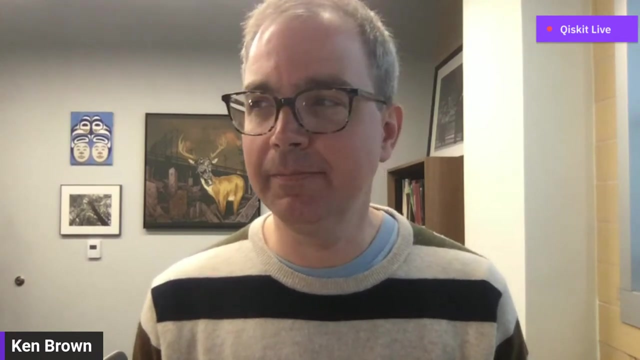 I felt like my theory was really disconnected from- yeah, just just disconnected from what was actually going on. And so I then did an experimental postdoc with Ike Chuang and then that kind of informed me of yeah, yeah, really informed me about like where this connection was. 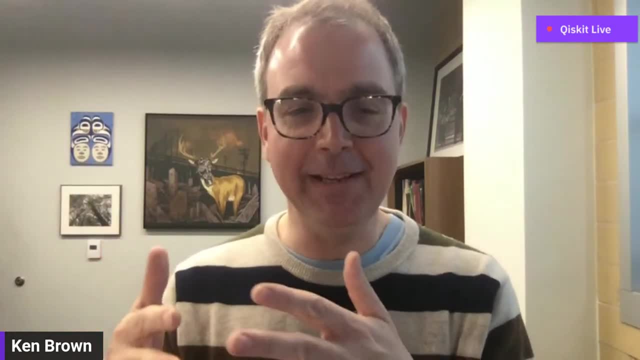 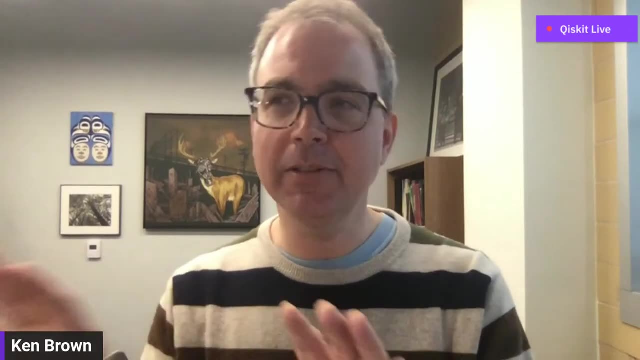 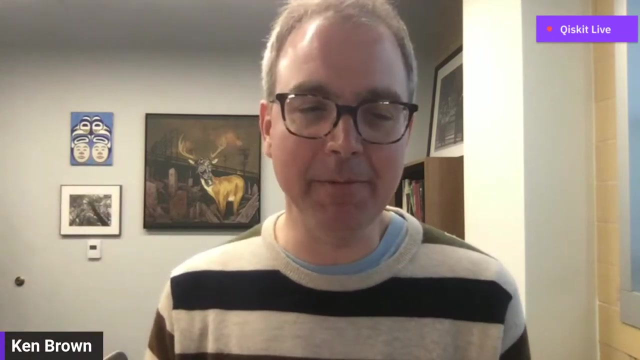 So I would say, if you want to head this way- I think you know, being a theorist who works closely with some experimental group really does open up new questions to ask, Because when you, when you don't talk to experimentalists, you just kind of imagine like, okay, these are these, I imagine these layers will happen, but maybe they don't happen.